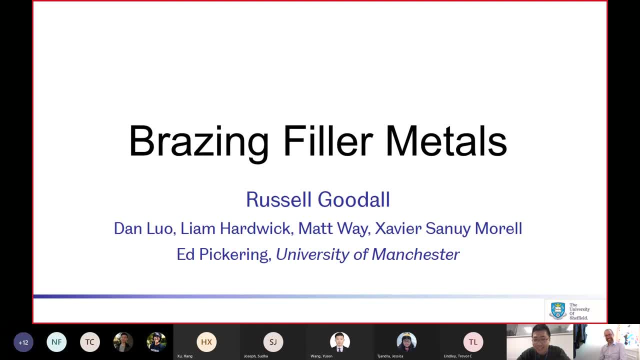 student conference in metallic materials. If any of us are interested in that conference, you can ask for more information from Russell. And today Russell is going to give us a talk about filler metals for brazing and how to design better brazing alloys by avoiding intermetallics. 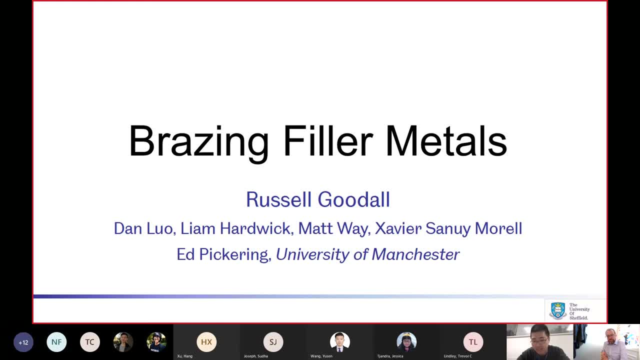 and using ideas from high entropy alloy research. So now let's welcome Professor Goodall to give us to take over the screen. Thank you, Thank you, Thank you very much. Just before I start, one thing to check. Am I aiming for about half an hour for the for the talk? 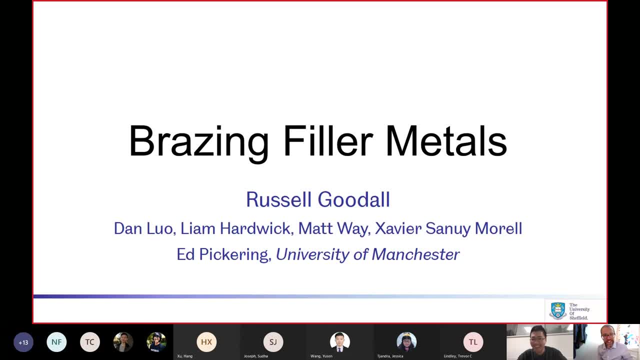 Yeah, it can be 40 minutes. Okay, that's, that's good, Because I I intended it to be half an hour But looking at it I think maybe it could be a bit longer. So we'll see. I'll do my best to nice not to keep longer than they need to be. But yes, thank you very. 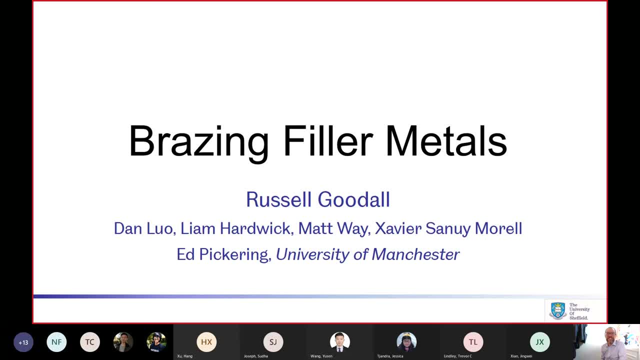 much for that, for that introduction And the plug for the conference, And also, indeed, for the invitation to speak today. My name is, say, Russell Goodall, And you see on the slide a name of a number of my research associates and students who work with me on this, And I should also acknowledge 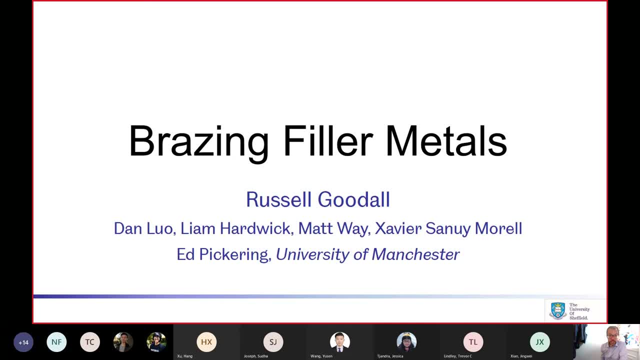 Ed Pickering from the University of Manchester, who's been, and continues to be, co supervisor of some of those students, with some good input into this work. So brazing filler metals is my title, And what I want to talk about today was first of all the brazing and explain. 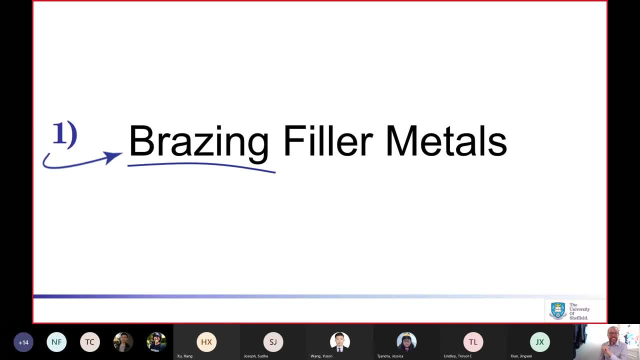 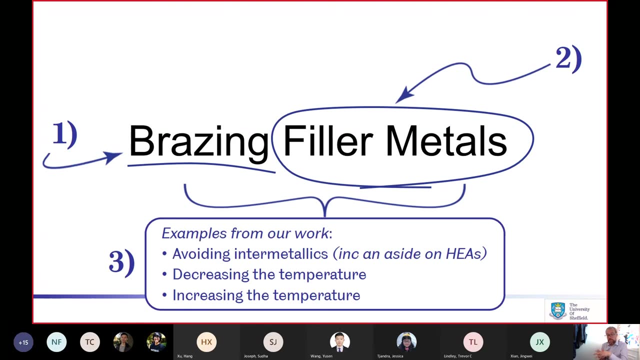 what that is. you might know, but just make sure. And then to zoom in on the filler metal side and say what I mean by by fillers, And then to to carry on with that. I wanted to talk about some examples from the work that we've been doing in this area, about trying 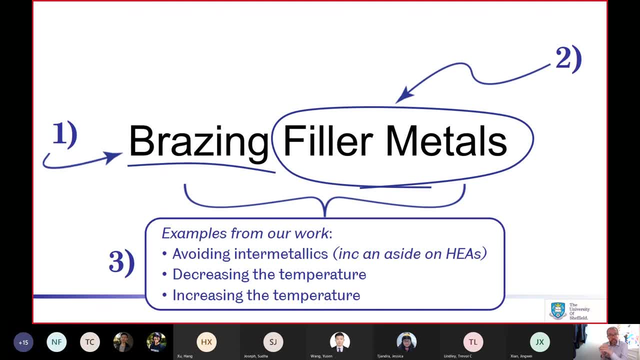 to avoid intermetallics in in the joint- And that's where I'll say a little bit about high entropy allies- and also trying to decrease the temperature of fillers operating at and also to increase the temperature- Two of the different challenges that we've tried to address. 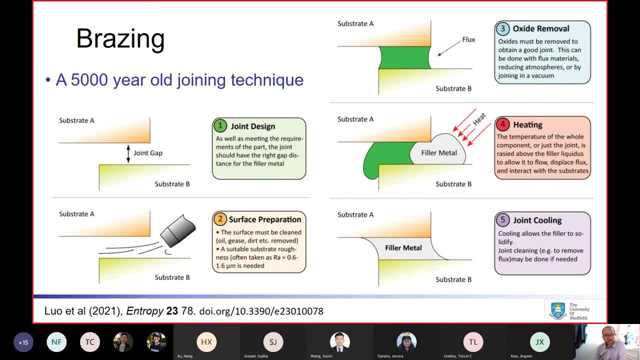 One of the challenges that we've tried to deal with. So brazing, first of all. brazing is a really old technology. It's been around for thousands of years and you can trace it back 5000 years or something, something like that. It's a way of joining two pieces. 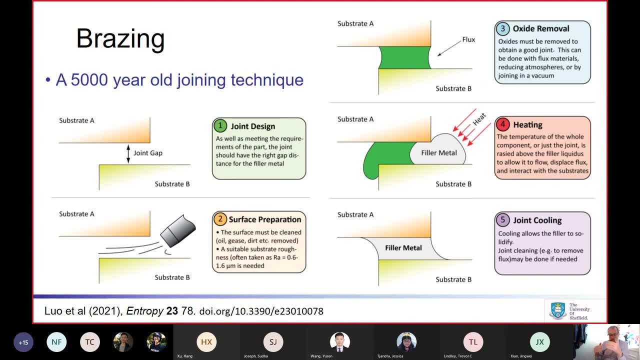 of material- often metals, but but not always. You start off by bringing those two pieces of metal together with a certain distance between them. You clean that surface and then you need to get rid of the, the oxide. Certainly if it's a, if it's a metal, most of them have a surface oxide and that will impede most. 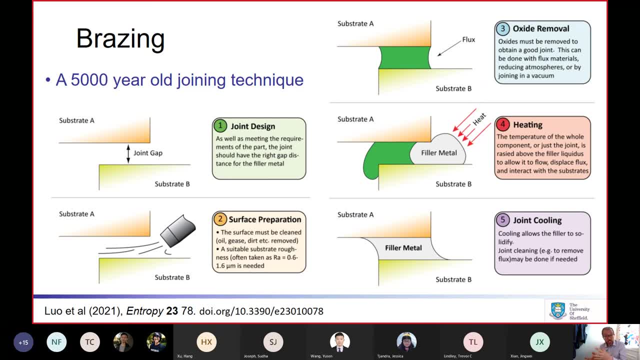 brazing processes. So you might use a vacuum, You might use a reducing atmosphere, if you have access to a furnace that can do that, Or you might use a substance called a flux. This is a, a softener salt, actually something that can be made. 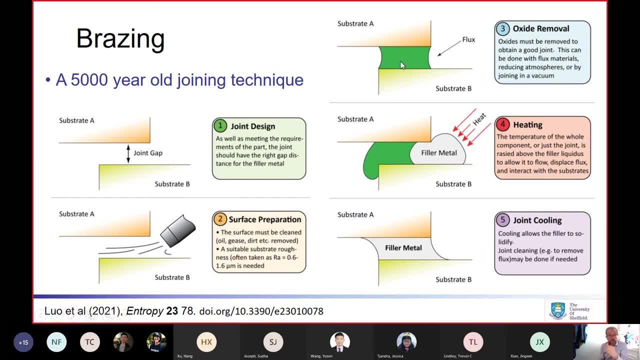 Melted flow into the gap, react with that oxide, dissolve it and sort of clean that surface ready for the filler metal, which is what you introduce next. You, you put the filler metal, you heat the joint. You obviously probably have to heat. 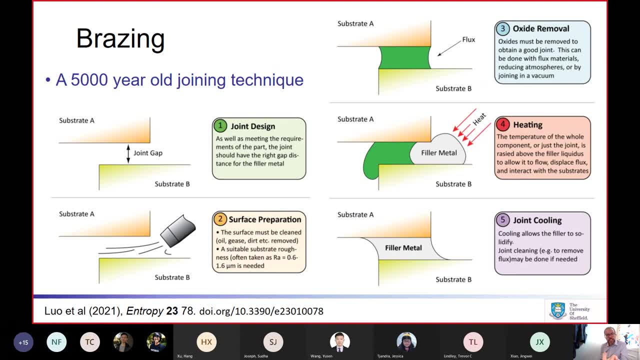 it to get the flux to work anyway. but you, you carry on heating that joint, You introduce the filler metal. the filler metal melts and then is drawn into that gap by capillary action And displaces the flux as it does so, And then you cool down and you end up with your 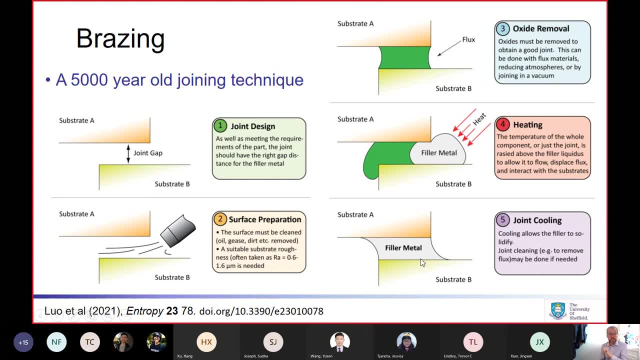 two pieces of material and the solidified filler metal in between them, forming a joint. That is the, the brazing process. There are many different variations: flux or no flux, type of heating, various things like that joint design as well, But that's the core. 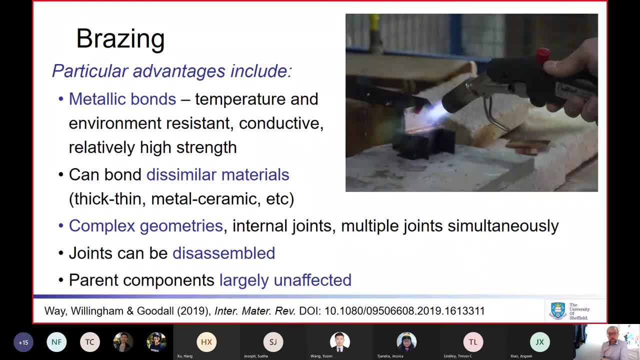 of the brazing process. So brazing is what? Well, despite being old it's, it's still used, and it's used because it has certain very key and specific advantages. You produce metallic bonds, so the bonds are electrically conductive. they're, they're thermally. 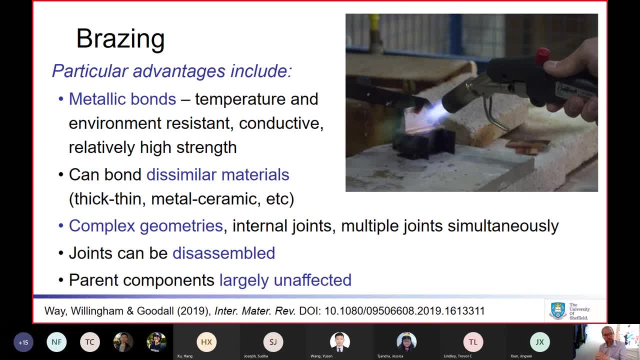 conductive. they're quite high strength. That can be important. You can- and this is perhaps one of the key advantages- You can join dissimilar materials so you can join different alloys. You can join metals to ceramics, ceramics to ceramics- Not with without any limitations whatsoever, but certainly with a very, very wide array. 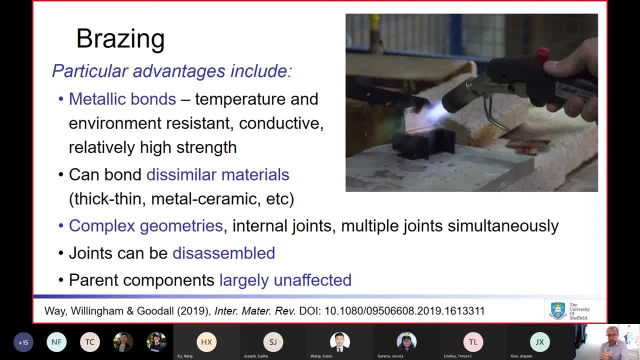 of different joining possibilities. You can also make joins between quite complex joints, and that can include joints where you can't. You can't see the, the, the joint, You can't get a- maybe a laser beam or electron beam into it. You could do several joints at the same time and that's one of the advantages for 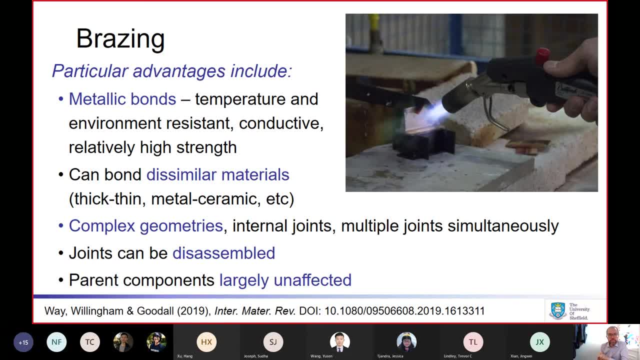 Say soldering, which is a related process to to brazing in the electronics industry is you can do many, many joints rapidly. You can also join thick components to thin components, because you're not actually melting the material that you're joining. The joints can be taken apart and that could have some implications for recyclability and 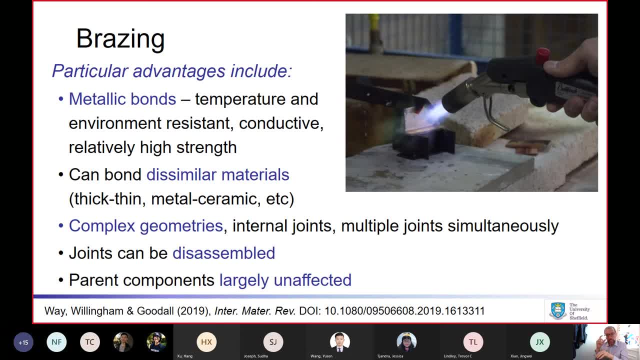 things like that, and also another key advantage is that the, the parent materials, the materials you're joining, Are basically unaffected by the process. hopefully, if you get it right so you can join it, You can join materials without affecting microstructural change upon them, which of course can also. 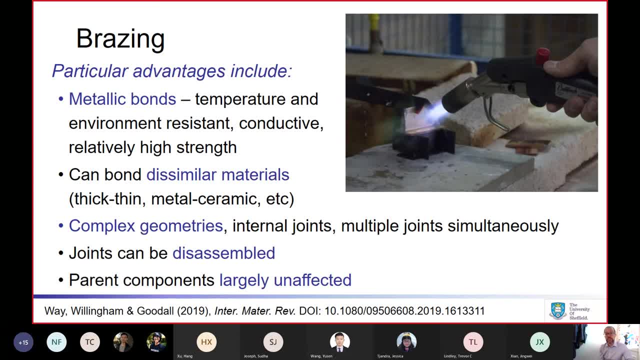 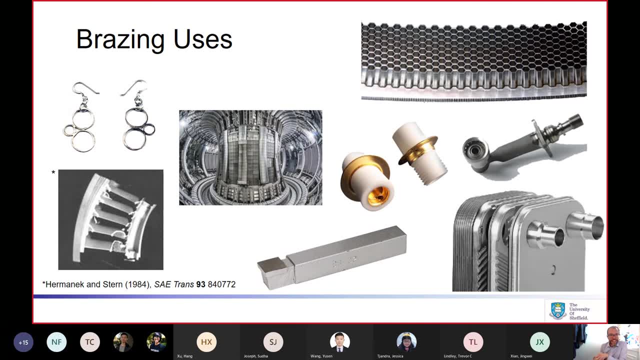 be an advantage if you've got particularly optimized microstructures. So where is brazing used? All sorts of different specific applications used in jewelry, silver soldering they call it, but the temperatures involved are brazing temperatures. It's likely possibly to have a role in infusion technology. 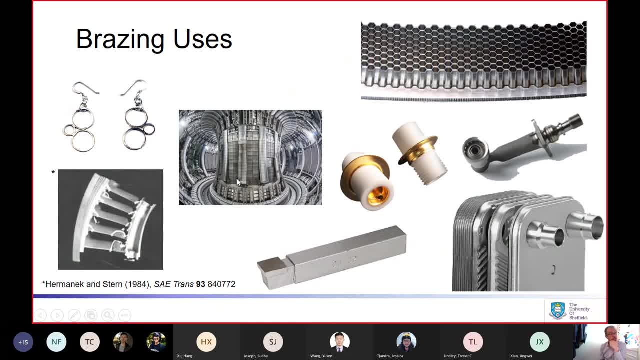 Some of the joints there between different materials may require brazing. This section of a turbine blade down. here is an interesting example. It's not used in turbine blade manufacture especially, but this is actually a repair. It's a ground based turbine for electrical generation from steam and the white lines. 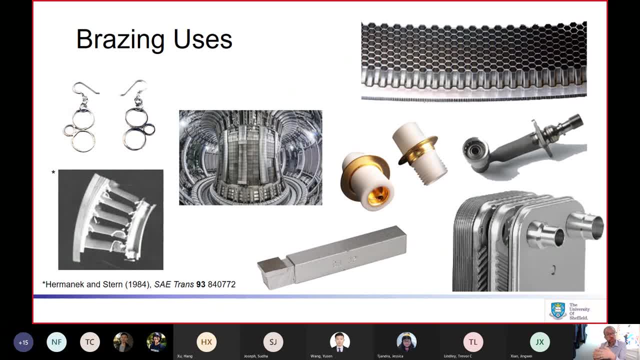 you can see in that Crack, Crack, Crack, Cracks and it's been repaired, It's been rejoined, The broken components have been re joined by a brazing process and that can extend the lifetime. It's used in ground based turbines because of, obviously, the sort of the safety case for 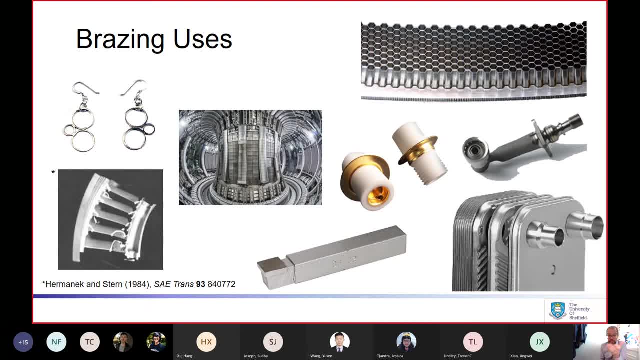 air for aerospace is a bit different but it does have a valuable role there. Other components, also aerospace. we've got the honeycombs joining thick to thin Some of the complicated parts in fuel nozzles. this article at the middle bottom is a tool so joining the, say, the tungsten carbide tool tip. 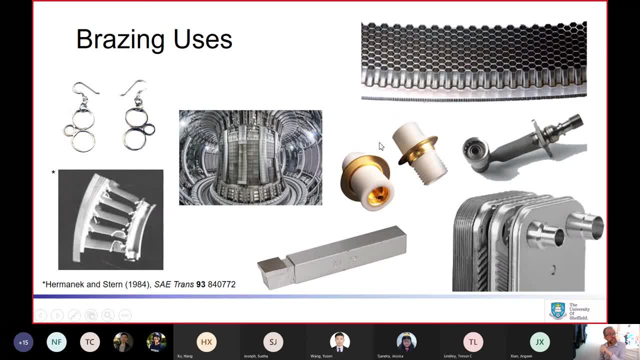 onto the body. that's done by brazing these components. in the middle are some electrical ports for vacuum technology, where you need to combine conductive metals with insulating ceramics and have a gas tight seal. so that's uses brazing and the final component down there is a heat. 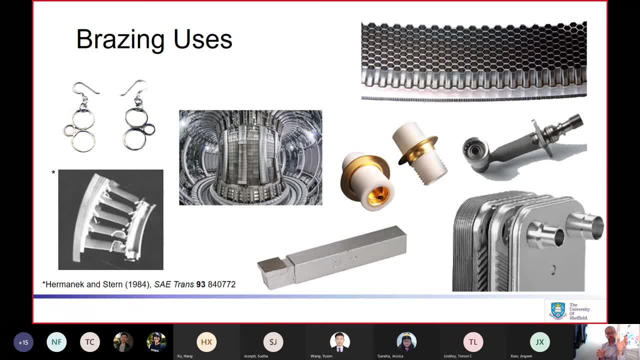 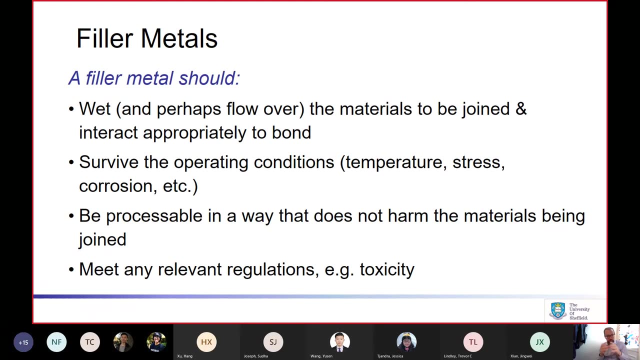 exchanger. so quite a broad array of different components which depend on brazing really, or certainly for which brazing is a very important technology. okay, so I then said we'd move on to the, the filler metals. so this is the bit that melts and actually sort of does the brazing, so a filler. 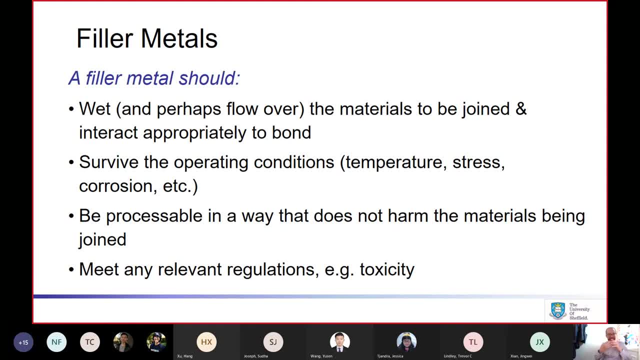 metal. well, it's going to need to to wet when it's molten. it needs to, needs to be happy being in contact with the metals. the materials it's going to bond might need to flow as well, and it's going to need to produce a joint. it doesn't produce a joint, it's clearly no use. it's also going to have to survive, whatever. 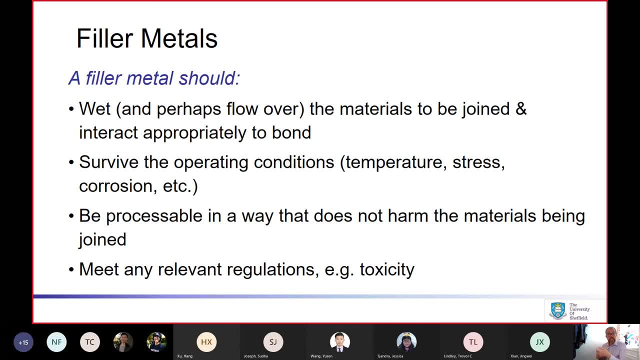 the operating conditions are the temperature, the stresses, any corrosive or oxidizing environments, anything like that, and it's going to be have to be compatible with processing that suits the materials that are being joined. so not too high temperature, not too reactive, those kind of considerations, and, of course, if there are regulations in that particular. 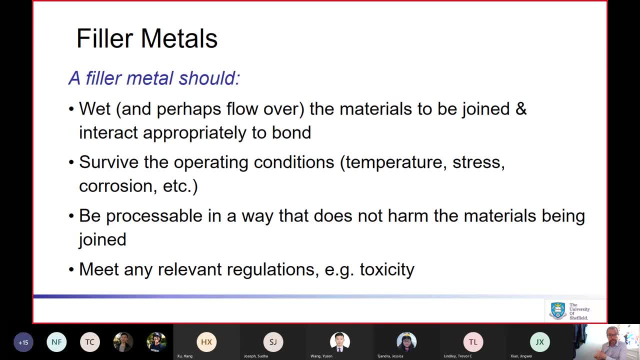 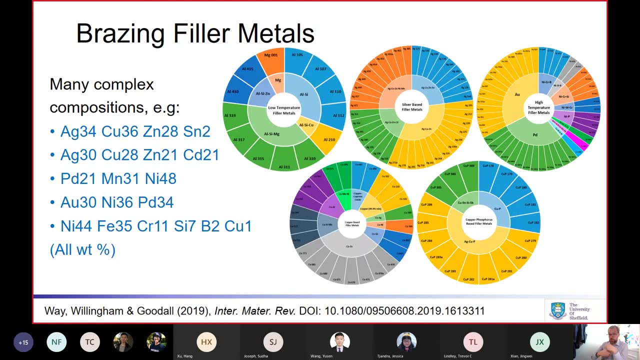 domain, then it will have to comply with those many filler metals of 30, 40 years ago would have had cadmium in them, but that's been largely phased out because of the, the toxicity requirements, for example. now, because of those broad array of different requirements, which are different for 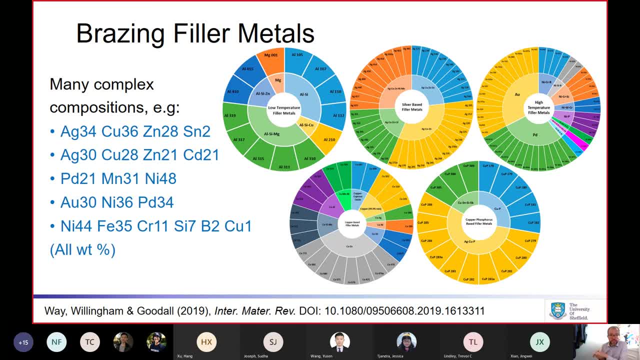 many different applications. there are lots of different applications that are going to be used for different filler metals out there and they can be quite complicated alloys. so these sort of radar charts show different families: low temperature fillers based on aluminium and magnesium, silver based, high temperature ones that can be based on gold, palladium, nickel and then the copper based. 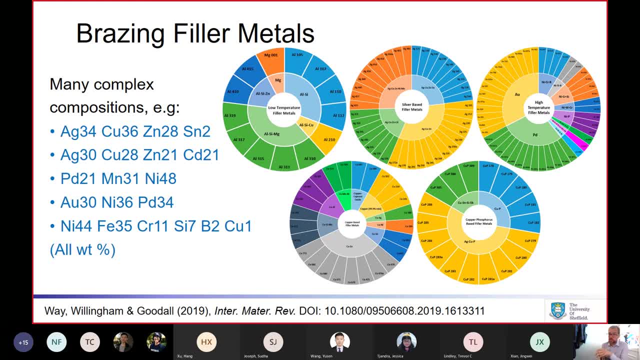 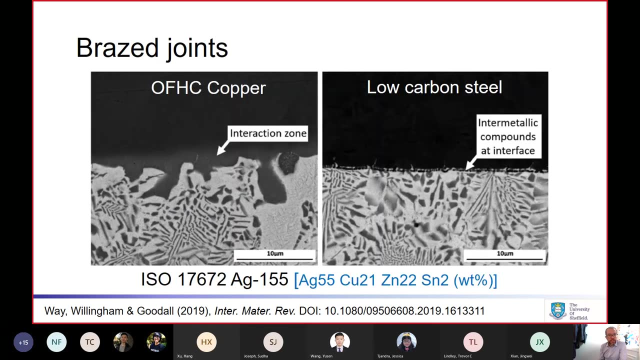 fillers. all sorts of different alloys are used, and some of them have actually quite quite a lot of elements in them and quite complicated property, and we need to use those as well. so what we're now going to look at are some of the best conditions for our problems, and I think they're gonna be pretty easy to look at. you can work down over and 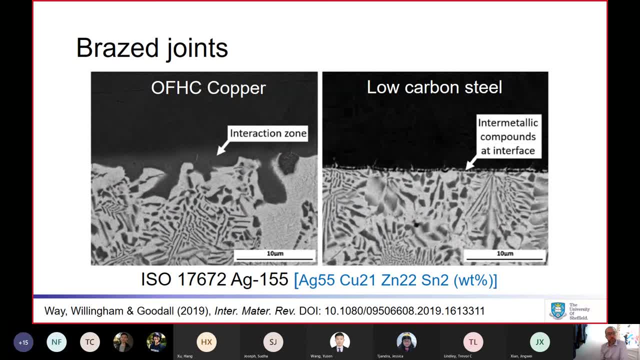 through it. break your chain if you try to set them in, going to a specific fault processing method when you're installing two or more instruments, and don't do that because you're gonna be able to work around it if you have a device that is a little bit smaller, if you're 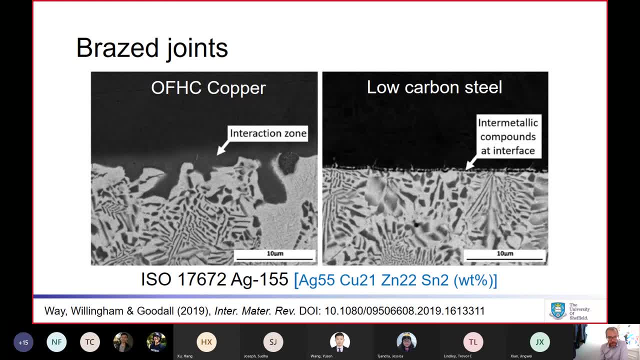 using a well made French chain. you've got to get in there. but when you're doing that, you're going to need a lot of delete or some sort of blurry sort of memory in order to achieve some sort of these kinds of problems. so that's kind of what we're looking at with this first group is we're talking about? 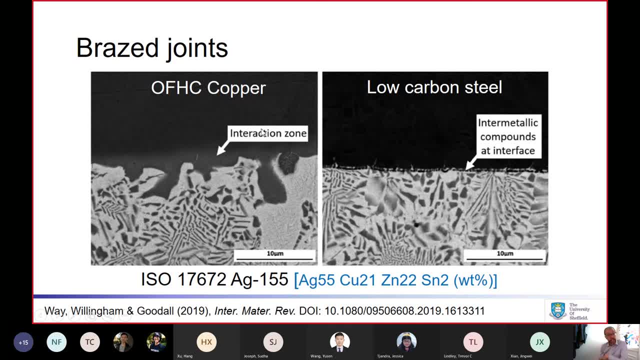 the first image it's copper and in that case this particular filler it's got copper in it. it alloys with the copper. you can sort of see in the micrograph there's a slightly hazy zone. as it's, we've got this interaction, some dissolution and diffusion happening between the two. 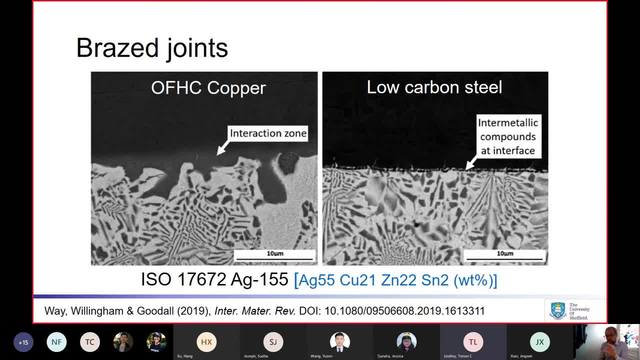 that's helping to make that bond, but that's not essential. we can also use this filler to bond to steels. in the steel's case, we don't get particular inter inter-alloying or diffusion. we rather get the formation of some intermetallics, this line of compounds forming at the surface. we get 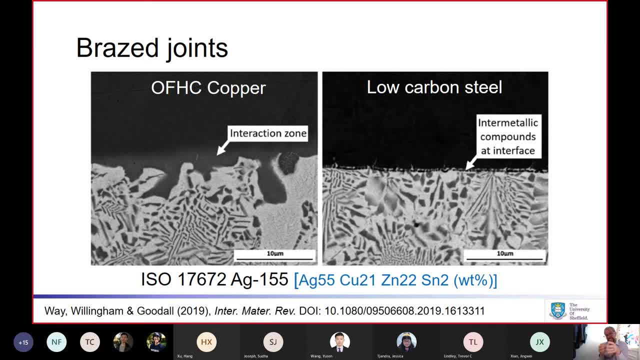 intermetallic formation through reaction between the two, and it's that that makes the bond um in that particular case. so different things can happen. it's not a uniform picture by any means, but it does. both of these instances would fulfill those requirements for fillers that i set out. 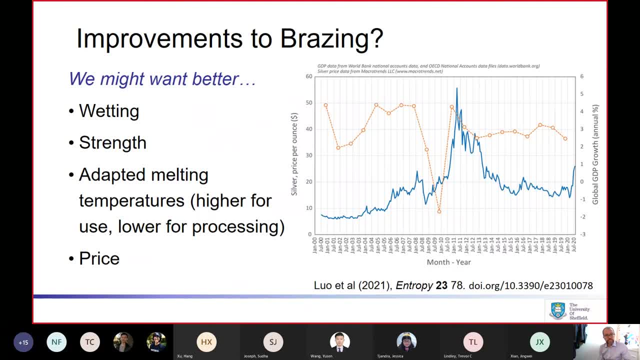 earlier, um, so what might we want to do? uh, clearly, brazing does a lot, it does some good stuff, it's a good technology, but, uh, i've talked about us working on it. so there's clearly things we might want to improve, um, and of course, we want to improve any of those particular behaviors, any of those key. 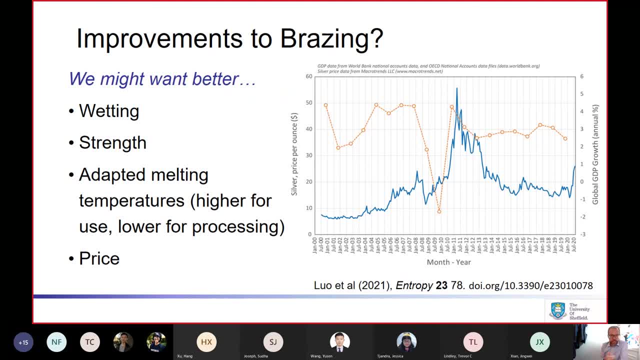 behaviors, perhaps for new applications on new materials. sometimes wetting isn't very good. the no Duck wetting is not very good because it's going to well. you know you want to do it with the. probably wetting isn't very good. the no duck wetting isn't very good, but you know a little bit of. 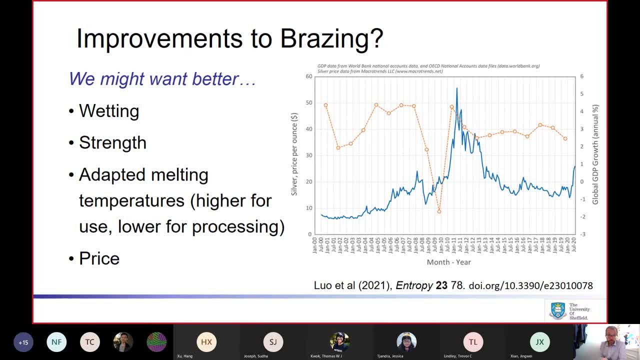 wetting isn't very good because the more wetting you can do with the material, perhaps a lot more fillers don't respond well to all materials, particularly new materials, So we might need to develop new fillers. as a result, The joints are actually pretty strong. They're not as strong as 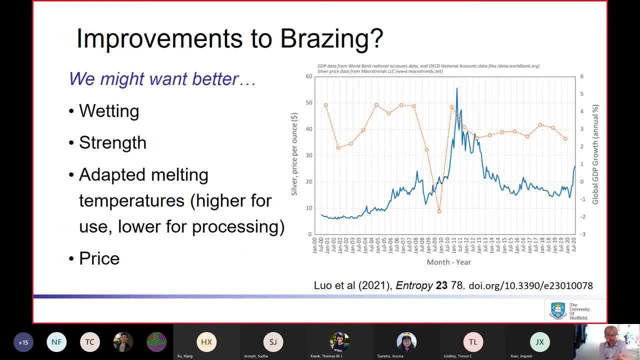 a well, but they're stronger than an adhesive or something like that. So strength isn't too bad, but it could be better. We might want to improve the strength. We might want to adapt the melting temperatures. We might want to increase the melting temperature because applications demand. 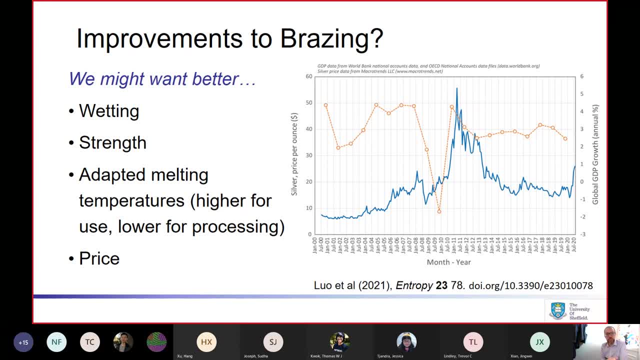 often higher temperatures, Or we might want to reduce the melting temperatures to make our processing easier. And also, of course, price. Price is always something we'd like to bring down And some of those fillers- some of them use gold, some of them use palladium, some of them use 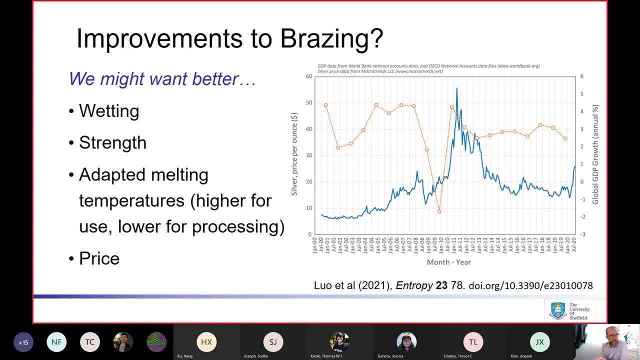 silver, And these are ones that are, you know, not ultra rare or extremely specialist examples. They're not. They're used moderately widely And of course the price of those is very volatile. The graph there shows, for the last 20 years or so, how the blue line, the price of silver, has varied, And 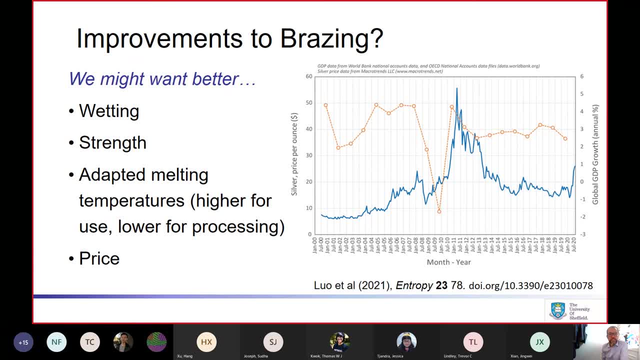 it's, you know, relatively volatile, obviously tracking the inversely, tracking the state of the global economy. So when the economy suffers a shock, as it has done at the moment, the price of silver and gold as well, Well, we'll go up and that can make those, those fillers, a lot more expensive for the applications. 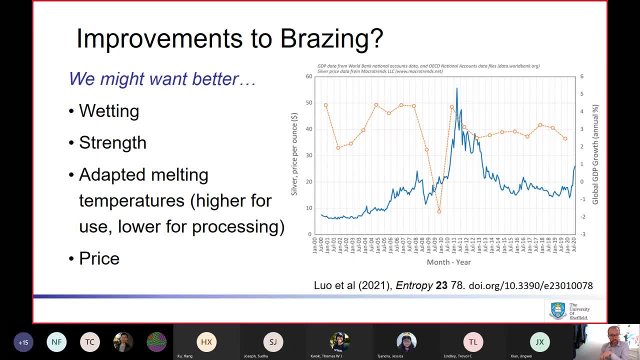 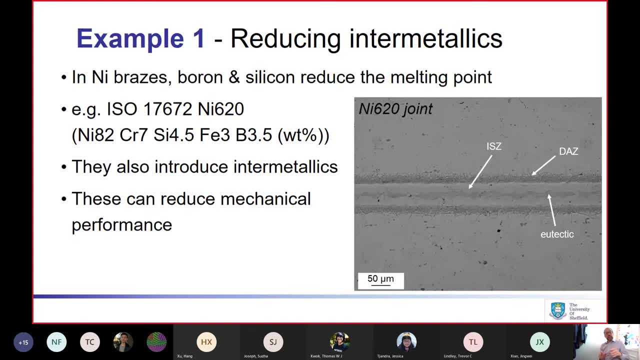 they're used to. So these are the sorts of things we want to achieve, And I'm going to talk about a few examples of things we've tried to do in this sort of area. So the first example I wanted to mention was the idea of trying to reduce intermetallics And this 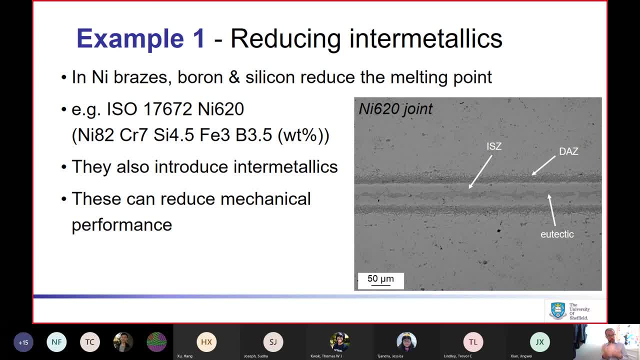 is in particular in brazing nickel or brazing superalloys. So it's sort of the jet engine type or aerospace type uses. at least Now, in those kind of alloys, the filler metals that are used for brazing nickel, we have many of the same elements that we might find in a superalloy. 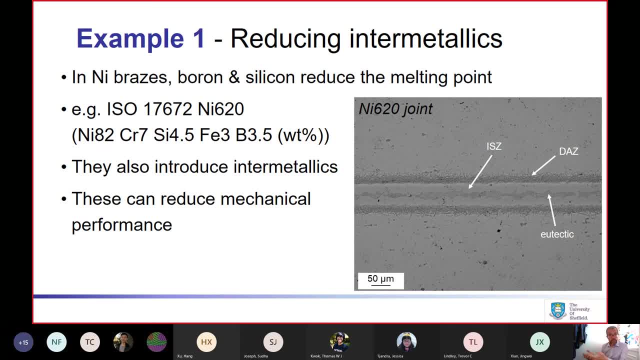 But to bring the melting temperature down so we don't end up melting the materials we want to join. the standard compositions often use boron and silicon And these are added in to reduce the melting temperature. So a fairly typical one: nickel 620.. 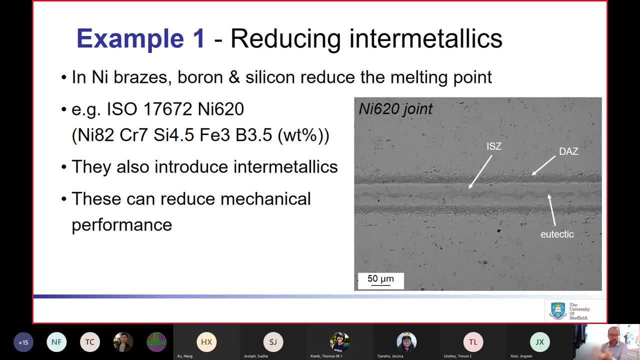 It has nickel, chrome, iron, but it's also got some silicon and some boron in there And they're very effective. they do reduce the melting temperature so that we can get that alloy to melt well before grades of superalloy, But they also leave behind intermetallic silicides and borides. 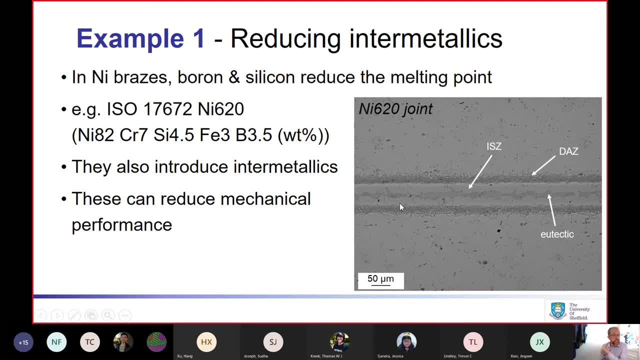 And if those are concentrated along the center of the joint. so this is two pieces of superalloy and the line in the middle is the is the joint line And this middle bit here where we get the eutectic around there, there can be the. 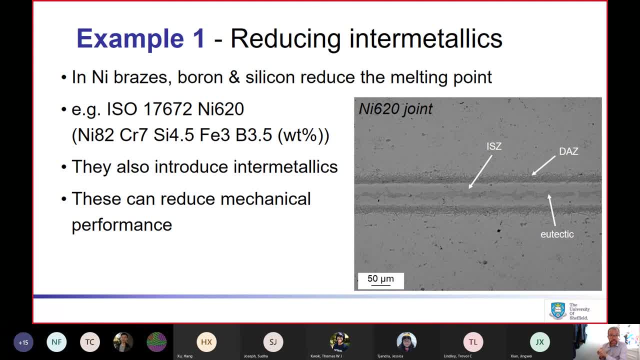 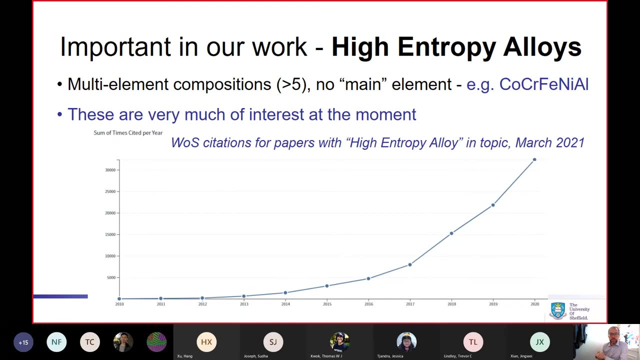 formation of intermetallics which can harm the mechanical performance. So we want to get rid of those, if we can reduce their amount at very least. Now, in doing this, and in fact in doing quite a lot of our work, we've drawn upon the ideas of high entropy alloys, And I'm sure you've 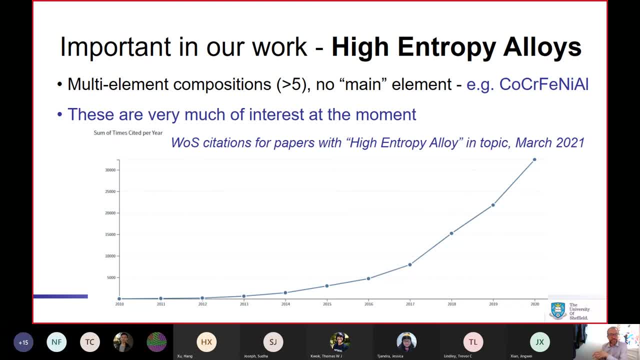 heard about these. You may work on these yourself or encountered them in your research, or you may just have heard about them. But, very briefly, these are alloys where we have multiple elements and there isn't really a main element that we can say dominates. 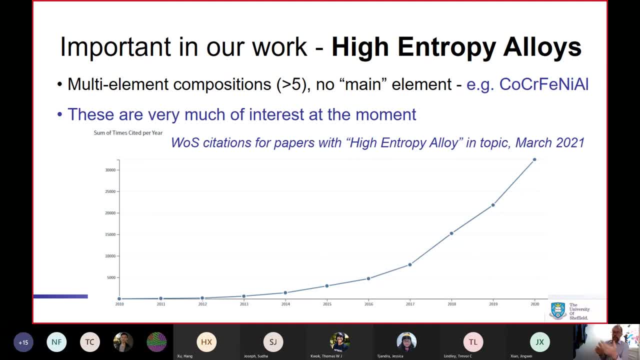 that composition. So it could be, for example, equiatomic cobalt, chrome, iron, nickel, aluminium, The same amount, the same proportion of atoms of each of those combined together, And these are of course very much of interest for us. 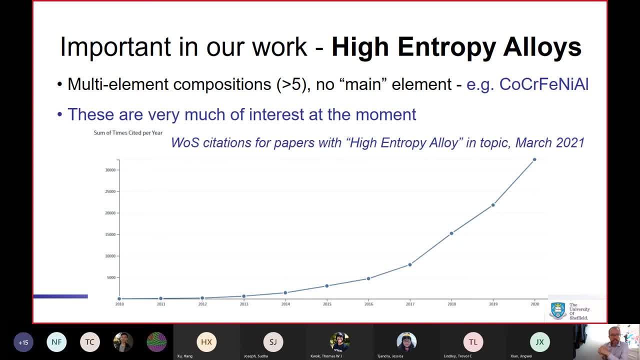 They've shown exciting properties and all of this sort of thing. And if you look at the citations that are coming in for papers with high entropy alloy, we see this massively exploding rate of interest and citations in the area And this is the kind of 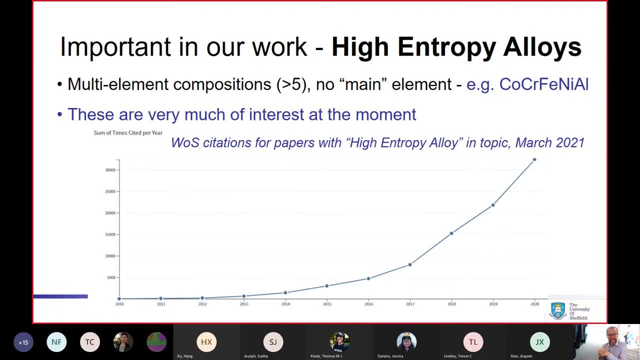 graph that people do sometimes show when they want to say that their research area is exciting. I would just caution you to be a little bit careful of this kind of data, though, because when I was producing this, slide the data here for the citations in high entropy alloys and how that's increasing. I decided to look at some. 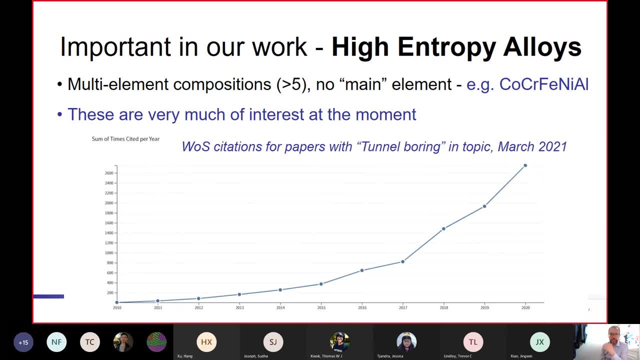 other topics And if you look, for example, at tunnel boring, you see a similar, actual. there's not too different a rate. oops, wrong way that way. So, comparing the two, maybe ever so slightly higher for the HEAs, but not too different a rate in terms of the increase. 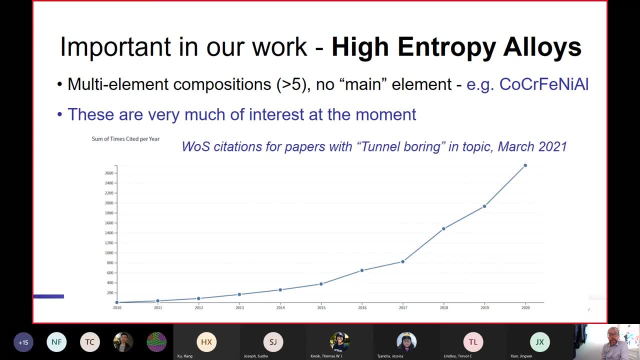 the baseline number is lower, but the increase is going up. Now I'm not a geo technologist or anything I don't know. Perhaps there are exciting advances in tunnel boring, but I think the point is that the volume of all research is increasing. 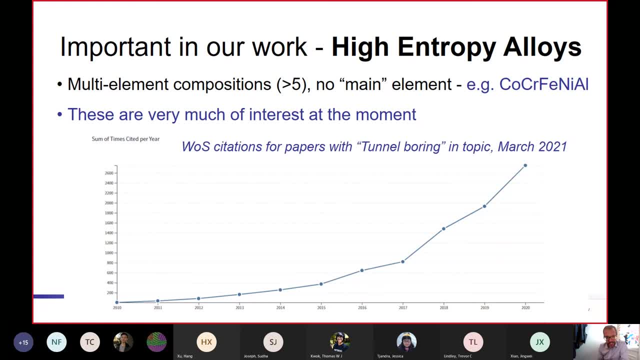 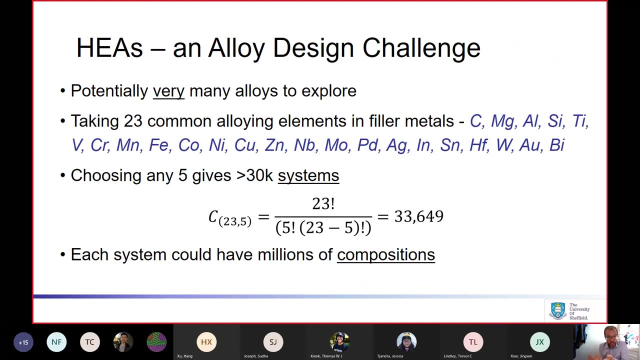 So the citations of everything are going up. But taking that aside, leaving that aside as a side point, HEAs are an exciting topic, a topic of interest in metallurgy at least, And they present- whoops, they present some potential advantages here If we can get. 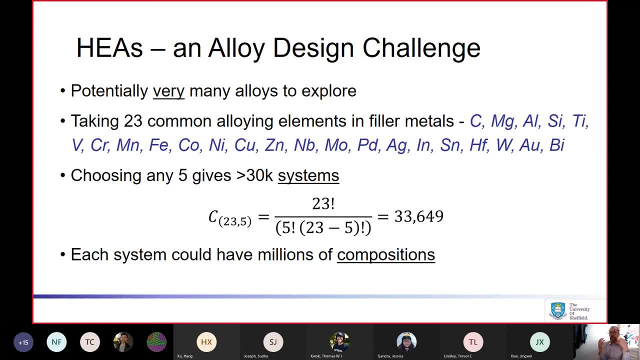 one of the cited effects of high entropy alloys is that this, the entropy of mixing, promotes mixing. The high entropy of having multiple elements in similar amounts can promote the formation of a solid solution, rather than distinct phases, rather than intermetallics. So there might be a route by. 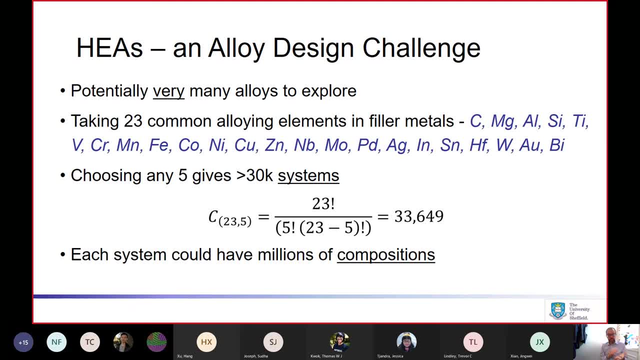 using high entropy alloy type alloys to have the melting point reduction effect that we want but not get the intermetallics. So to get for the brazing situation, the lower melting temperatures but not the problems with brittleness. So they present an advantage but they also present a challenge. 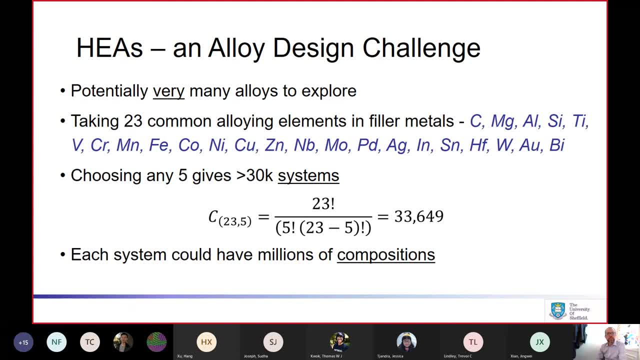 because there's a load of different alloys that we could explore. If I looked at filler metals in the metal in general, going back to those, those sort of standard fillers that I showed earlier, there's about 23 elements that crop up in there. the elements listed there: 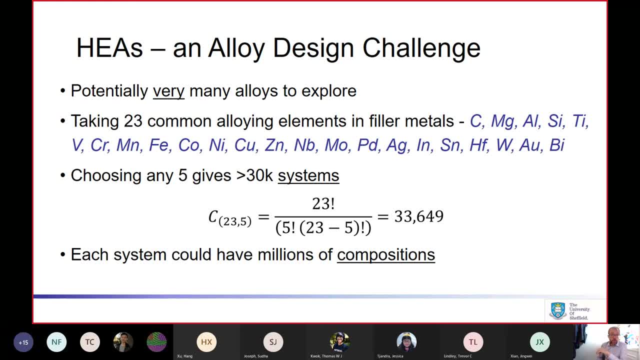 And if I was to choose a five component alloy that gives me more than 30,000 different systems to look at different selections from those And, of course, if I, if I want something that's not equiotomic and I want to vary. 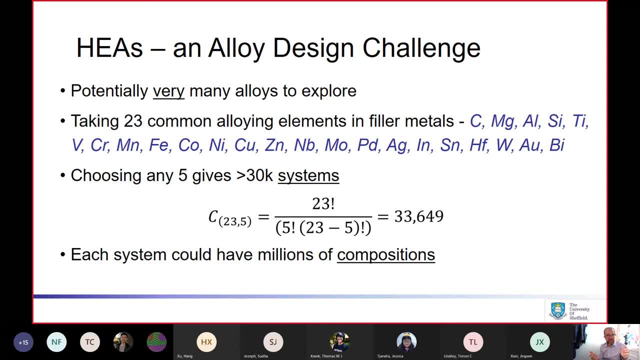 the compositional levels. I could have millions of different alloys to to search. So I can't- really I can't- do this by random exploration or by making lots of alloys and hoping that one is going to work. I need some kind of clues to to help me to do that. 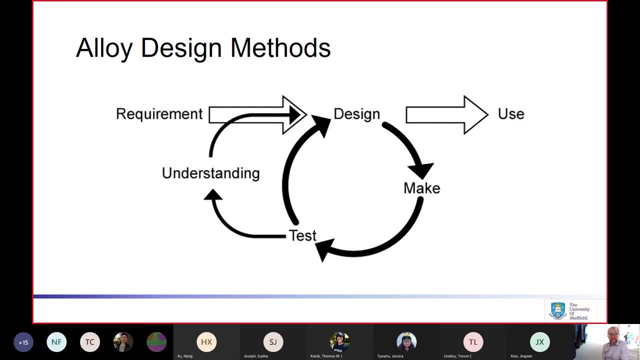 So we have to have some sort of methodology behind our alloy design And that's really like any kind of design process that we might do in engineering. We start off with some sort of requirement. We have a design, we come up with use, what knowledge, what understanding we have to come up. 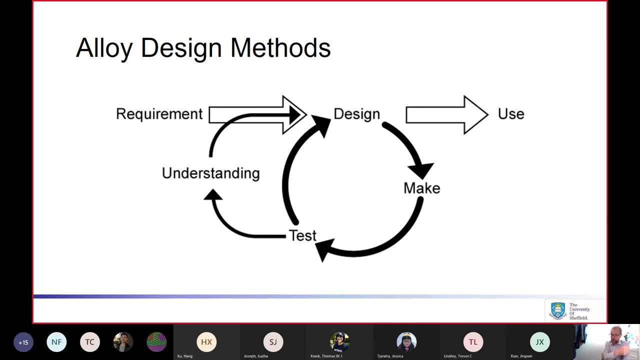 with a design, We make it, we test it. that might inform our understanding better, or we may iterate our design and eventually we have something ready for use And we try. this is how we try and do it with with our alloys. We get our requirements from our industrial partners. We we make a design. 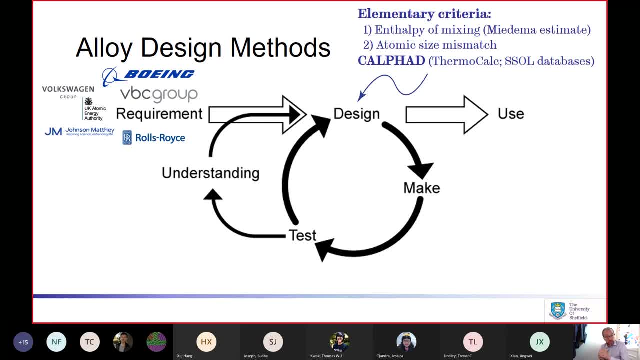 Now for this. we use some relatively simple criteria that we can calculate based on the elements. We calculate the enthalpy of mixing using the Medema method And we also calculate the average atomic size mismatch. Both of these are relatively simple. We can- we can do this with a simple script. 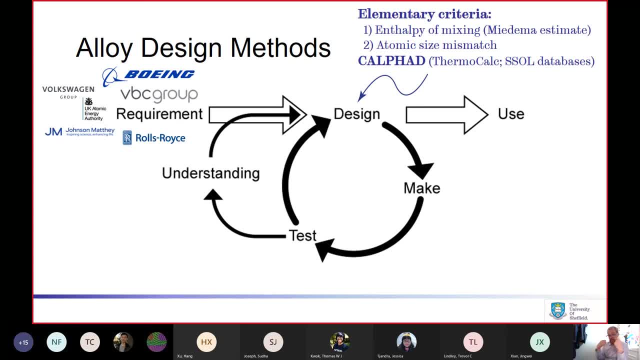 a Python script or similar And by doing that calculate these numbers for hundreds of thousands of compositions. We want the enthalpy of mixing to be small and slightly negative, to try and promote mixing, And we want the atomic size mismatch to be as small as possible, Also to promote the formation of a solid solution rather than. 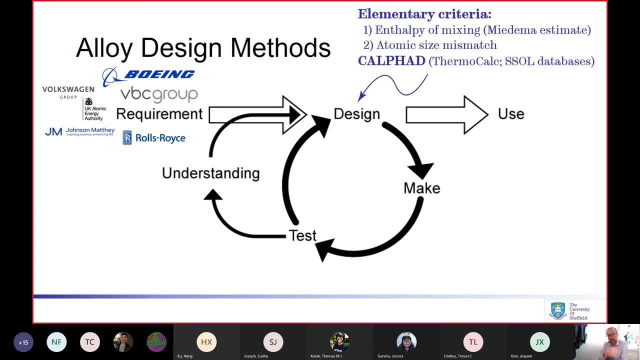 intermetallics, And this lets us go through very large numbers of compositions and discard the ones that have a very low chance of working. So this is what we do, We, we, we apply that route to go through many hundreds of thousands and take our best ones and then use CALFAT to learn more about. 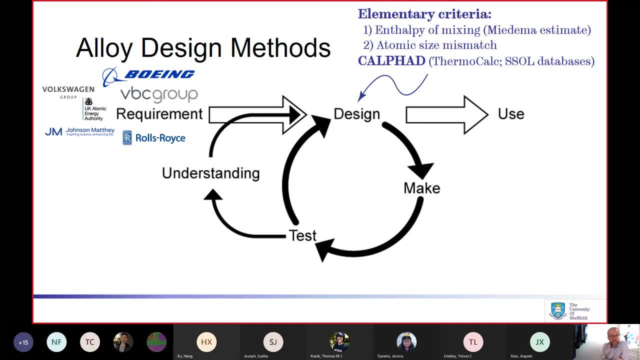 them to learn about their melting Temperatures, a bit more about their phase compositions and things like that. We we use Thermo-Calc and we've found the best results for this kind of still quite screening sort of stage. We're not worried about absolute precision. We want some answers that will help us. 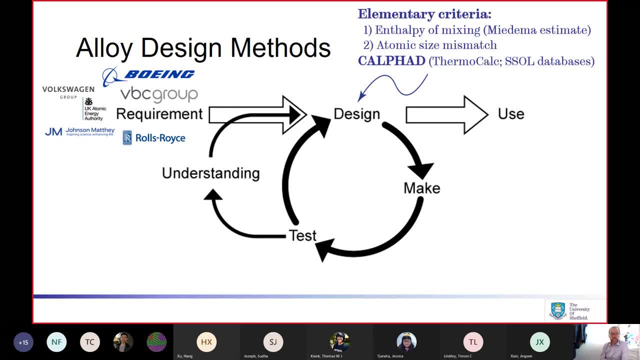 move on to the next stage. We find the solid solution. databases work best. for that There are high entropy alloy specific databases that Thermo-Calc have have issued, But we don't always. we don't always find for us that they, they may give us the best answers. Once we have that, 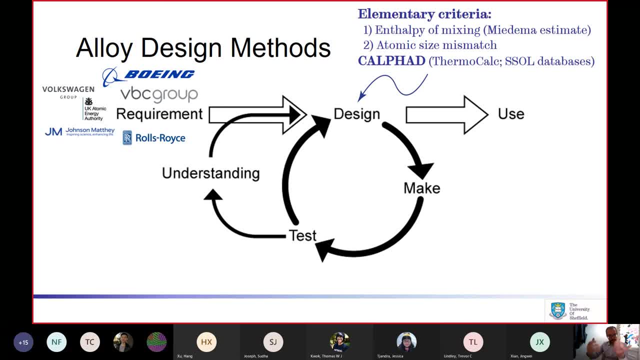 once we've taken a massive number and funneled it down to a smaller number and then iterated those a little bit with with Thermo-Calc, we then proceed to make the alloys. We might use arc melting, We might use induction melting, We can even use powder processing gas atomization. 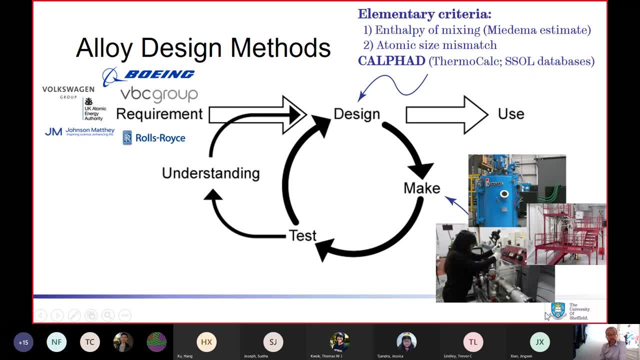 to to make it in powder form if we want to, because some brazing alloys are used in in powder form So we can test them. We try brazing with them. We look at their microstructures, their phase compositions and so on. mechanical properties perhaps and hopefully that will. 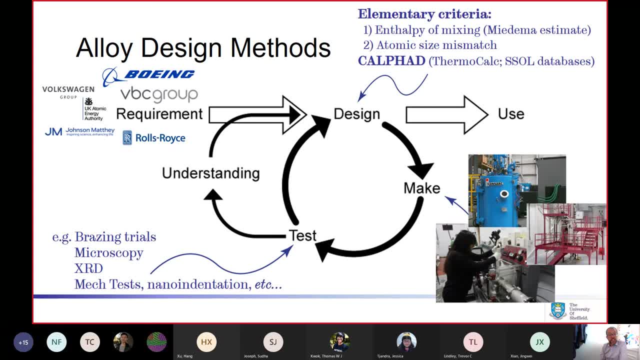 either lead to to good, good designs, better designs. It might even give us some understanding, which is what we really would label as sort of physical metallurgy, basic understanding of of how alloys work. And, of course, the holy grail will be if we get through all of this and actually 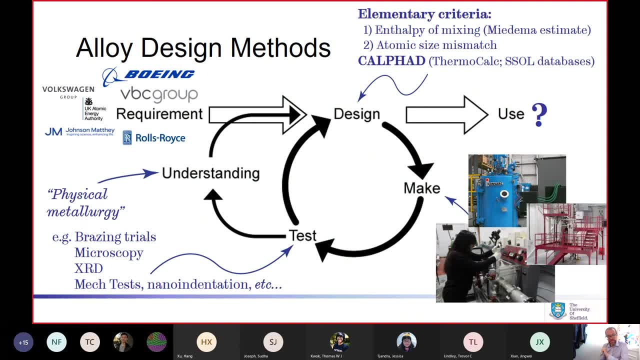 manage to get something that that can be used, And you know that's the. the end target is seeing some of these designs come out and be actually applied in practical situations. So this is our approach and we use this quite widely for our brazing alloy design In this. 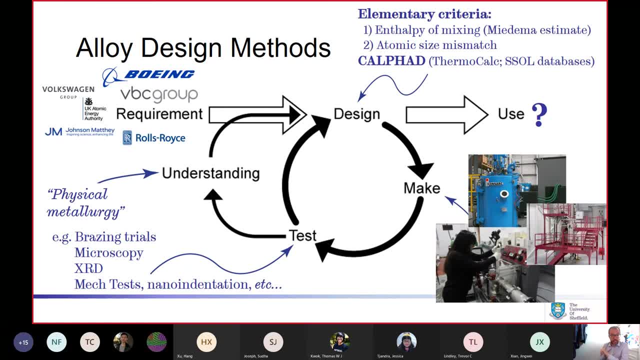 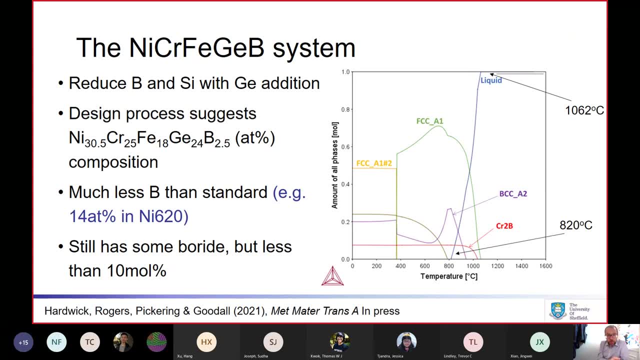 particular example, the reducing the, the intermetallics in, in nickel brazes. we, we, we took an approach where we we wanted to reduce the boron and the silicon and we explored a number of different possible ways of doing this, But we 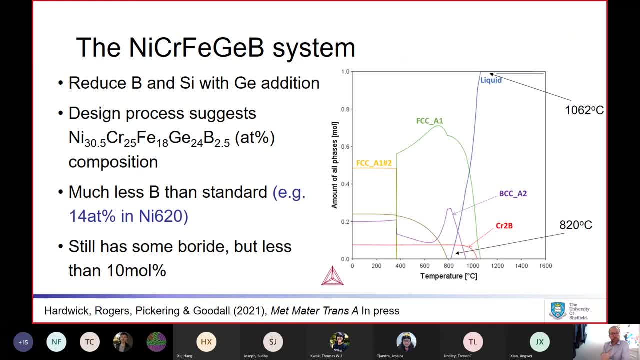 found that there was some signs that using germanium, adding in germanium, would allow us to do that, And through that design process we ended up with this particular composition shown here: nickel, chrome, iron, germanium and boron. So we've got rid of the silicon entirely and 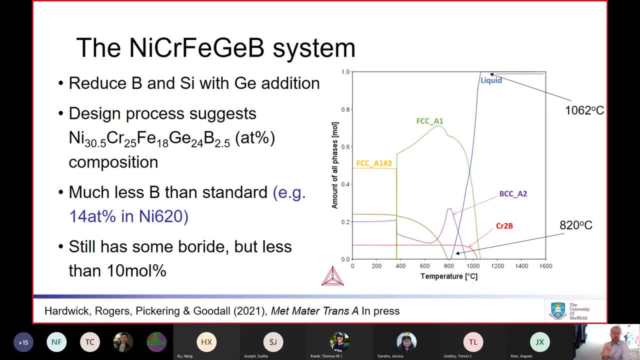 we've actually reduced the boron quite a bit. So this alloy is shown in atomic percent. So that's much less than the standard amount, Because it would be about 14 atomic percent in nickel 620 grade. Our thermocalc shows: 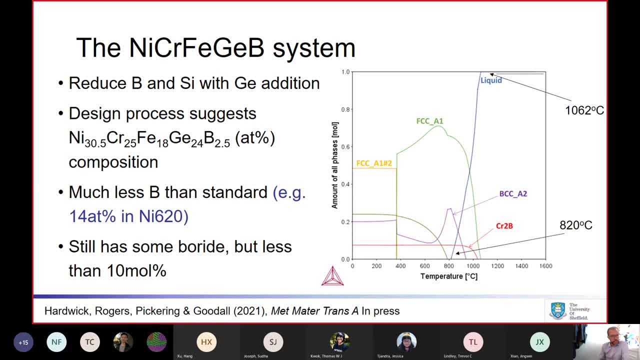 indicates to us that there's still some boride present, but it's it's relatively small, small amount, So we hope to be able to live with that. So we proceed, after the refinement there with thermocalc to make the alloy up. This is the. 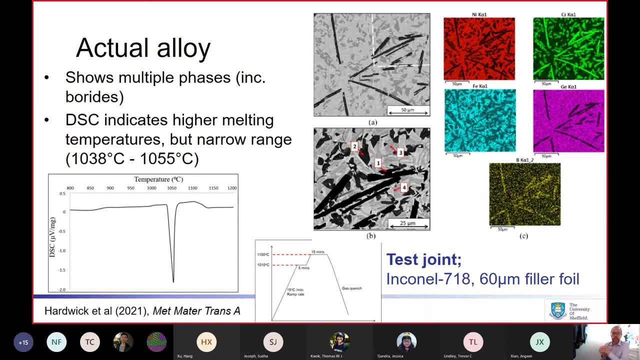 this sort of the as-cast, just the bulk filler metal. It has multiple phases. more actually find them was predicted by thermocalc and actually a slightly slightly higher melting range, but still quite a narrow range, which is good. That's generally what you want for a filler metal. 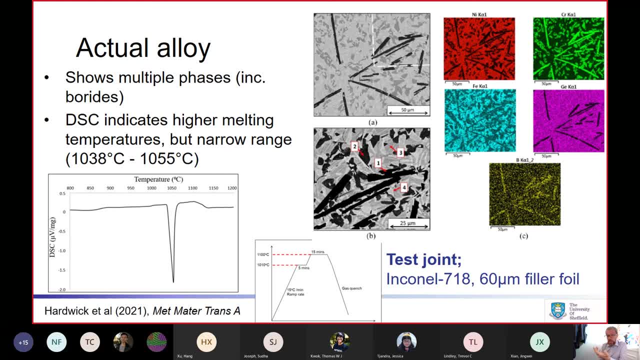 So we can look, we see, yes, there are some borides in there and they're quite big borides in the as-cast state, which is wouldn't be ideal for for a joint, but that we wanted to sort of progress. this because the filler metal in its bulk form is not the 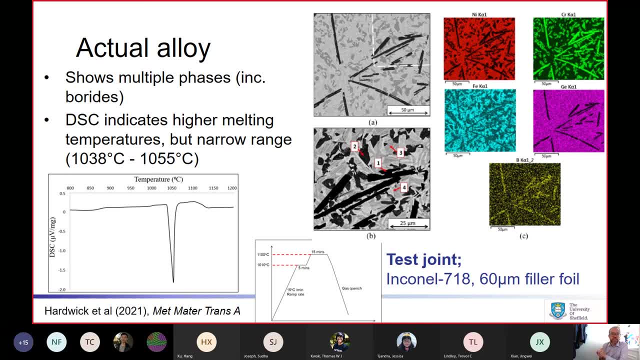 is not the end goal. We want to sort of analyse a joint. The DSC lets us set a thermal profile for a brazing trial and we carried that out. a test joint on Inconel 718 with a 60 micron thick filler. 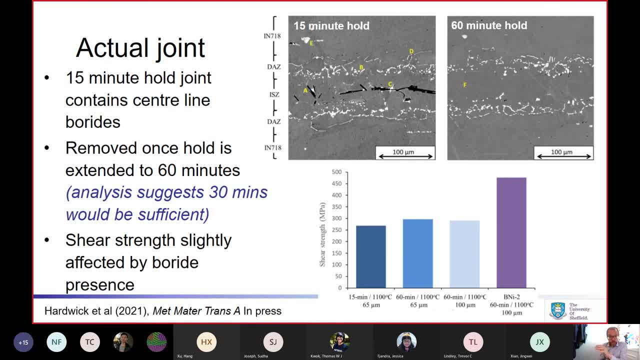 And we've. these are the sort of results we find Looking across the joint again. So the top, the top and bottom are the Inconel and the bit in the middle is: is our filler solidified to make the joint? Now, if we hold it for 15 minutes, we see these: 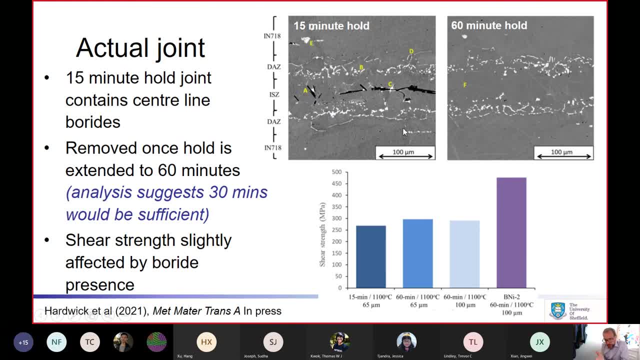 these phases, these big black phases right along the middle of the joint, which are borides. That is not an ideal structure. Certainly, visually doesn't look ideal to have the borides concentrated along the middle. but if we hold it for longer, because boron is, 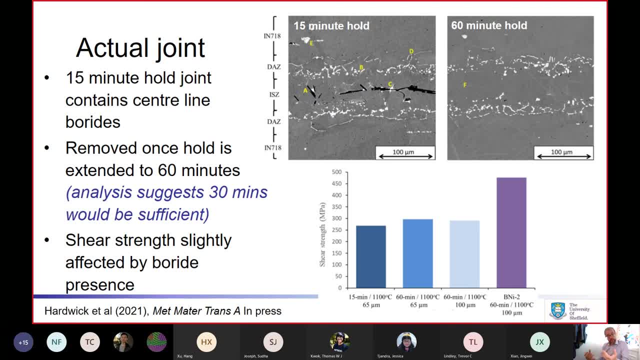 quite a small element. it's quite mobile, It can diffuse away So that longer hold produces a joint that doesn't have those those borides visible. And in fact when we, when we sort of fully analyse the various different tests we did, the indications are that about a 30 minute hold time. 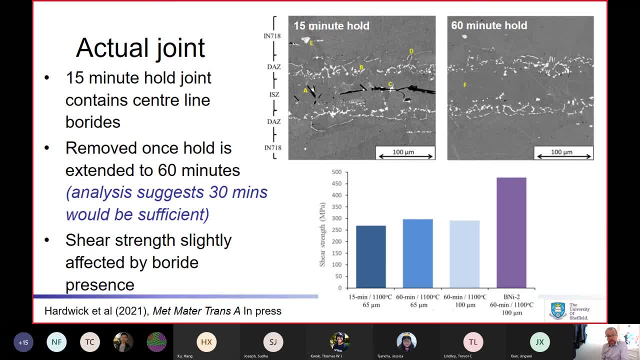 is probably going to be suitable for this alloy. So far we've assessed the shear strength. We haven't looked at the sort of the further mechanical properties that might also show some more differences. but the shear strength of the joint shows well, actually not a. 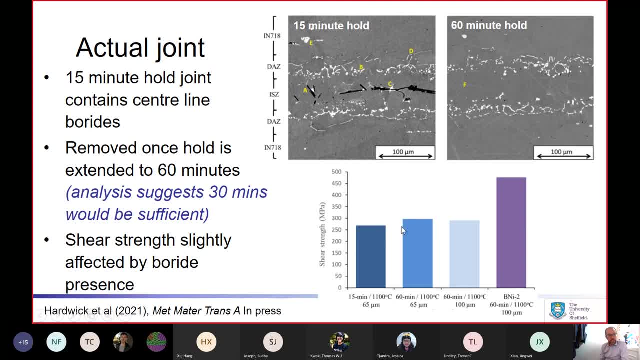 not a tremendous effect of of the boron. All right, All of our alloys, whether they're 15 minute or 60 minute tests give us relatively similar results, And we're not quite at the level of the standard fillers. The 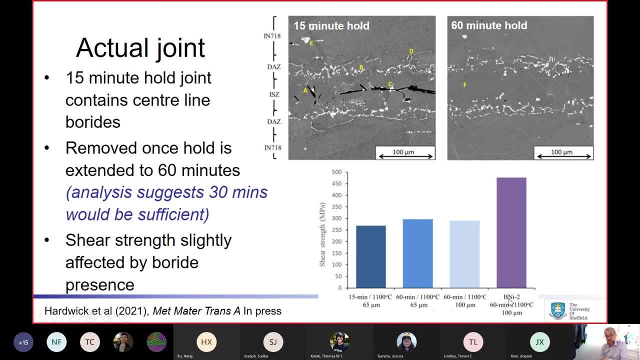 BNI2 is actually an American designation for the nickel 620 grade. It's the same, the same alloy. possibly due to the effect of some of these bright, these bright phases here are germanium phases, that that that are produced, perhaps there. 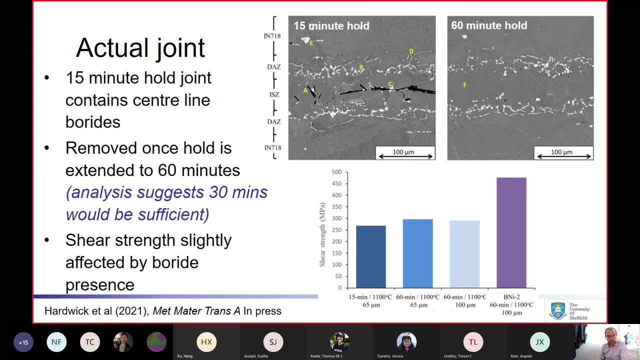 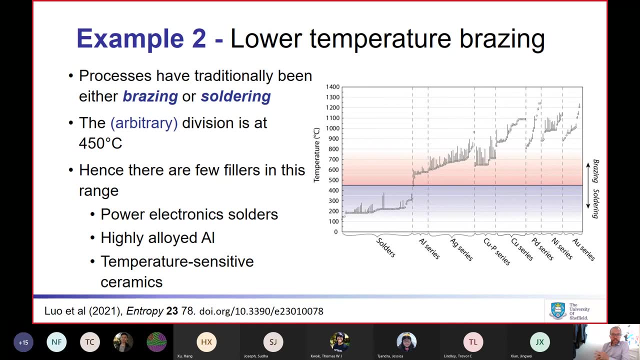 They're having a role, but also our joints are by no means yet optimised, whereas the the nickel 620 composition is. So we we're we're certainly looking further at this as a composition. So for my, my second example- that's the first- was talking about, obviously, 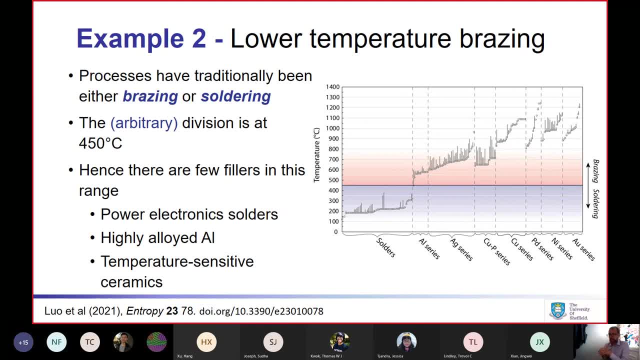 reducing the intermetallics. Another area of interest is to reduce the brazing temperature. Now historically, certainly within the the English speaking world, there's been a division between brazing and soldering and are set between an arbitrary temperature of 450 degrees Below that it's. 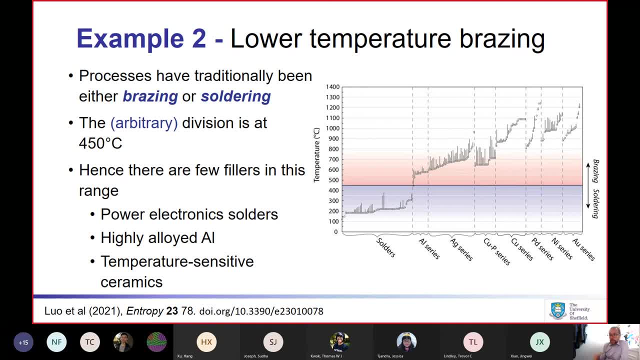 soldering. above that it's brazing, And it happens that, because of historical use, there are not many fillers around that gap. So the graph here shows melting temperatures in different groups of fillers: the solders, and then different series of brazing alloys. 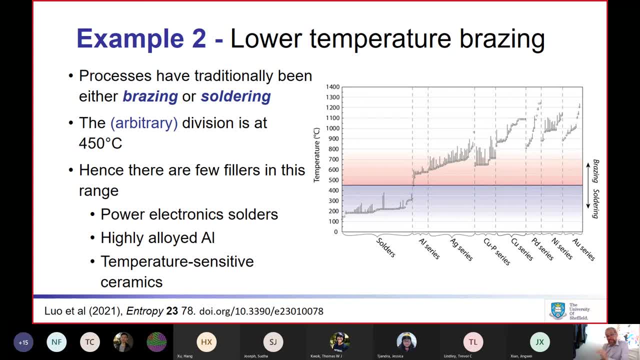 And the the spots. the bottom bit is the, the, the solidus, and the line extends up to the liquidus. So solders all have very, very similar melting characteristics. And then there's this jump between the solders and the aluminium series of brazing fillers, And then it progresses up to 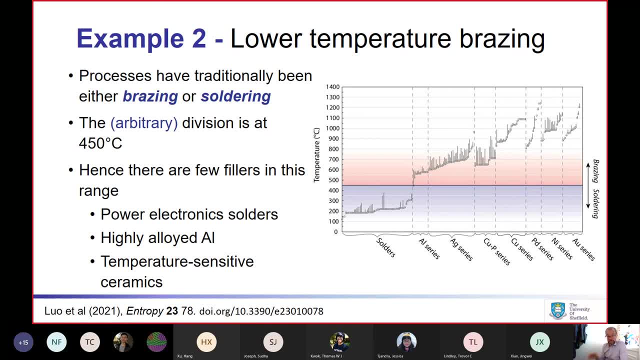 to higher temperatures. There's not really much in that region. If you want to process at about 400 to 500 degrees, you don't have a lot of choice. Historically probably we didn't really want to process at that temperature, but now we do. 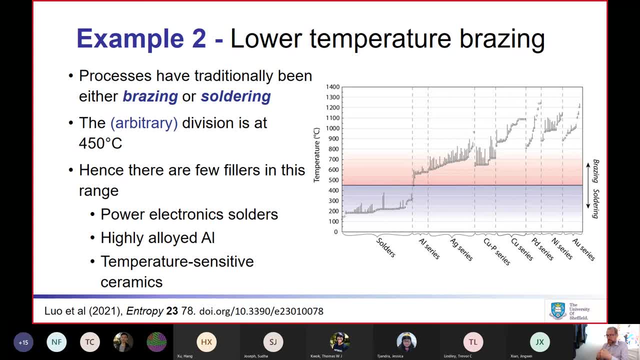 From the solder side- power electronics applications- there's more power, there's more demand placed on those. So they're getting hotter and they would like higher temperature solders. And from the brazing side things are coming down: Some very highly alloyed grades of aluminium, high strength aluminium. The melting temperature: 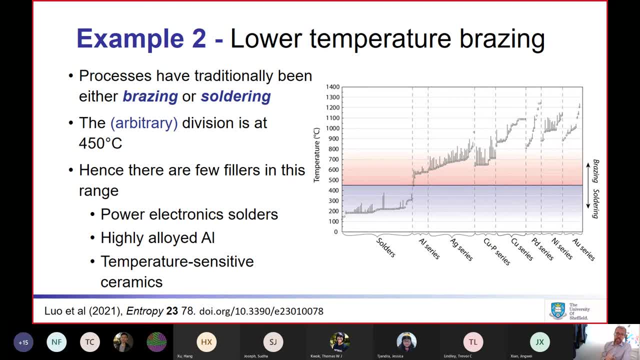 of the aluminium is reduced so much that you can't reuse the aluminium brazes on that without melting it. And there are also some functional ceramic materials that are temperature sensitive where you don't want to heat them too much in the brazing application. 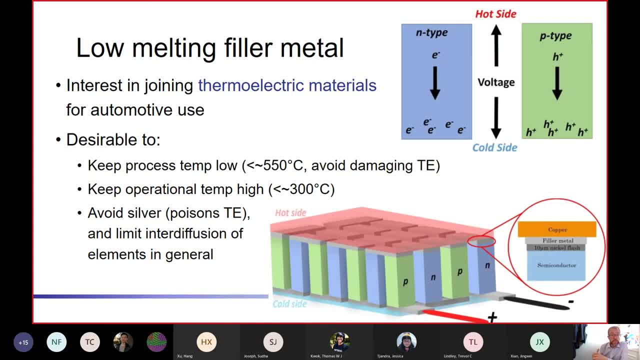 And that is that latter one is the example I wanted to talk about here, because we did some work on on joining of thermoelectric materials for use in automotive for sort of recovery of waste heat. So a thermoelectric material is one that generates a charge difference in response to a temperature. 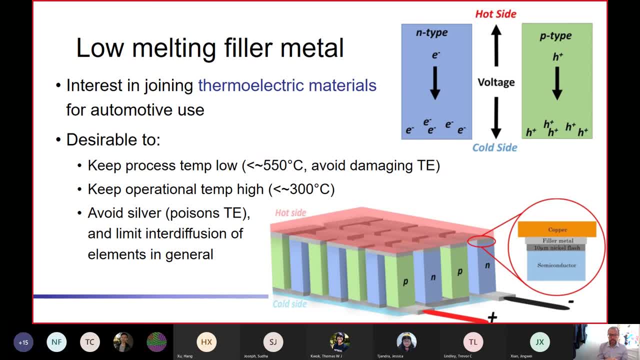 difference And if you create the right types and join them up in the right way- take the sort of pieces of the thermoelectric and join them up into a circuit, a device between, and place it somewhere between a hot and a cold side- you can generate sort of electrical power in that way. 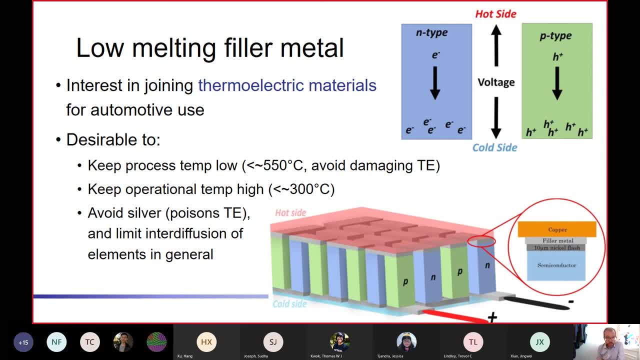 So there's a few requirements here. Brazing is a desirable technology. There's lots of joints, lots of joints between different materials that need to be made quickly, So brazing would be quite desirable, but the processing temperature needs to be quite low, because if it's too high, 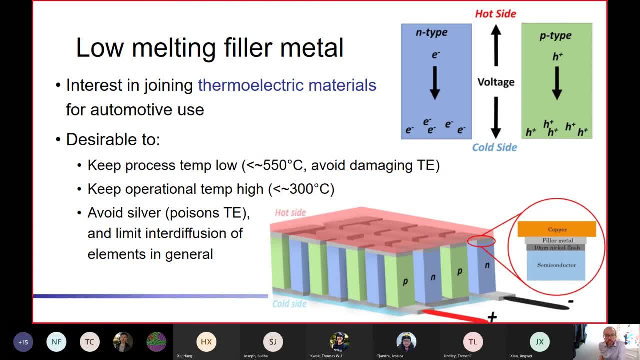 the sorts of materials that would be used for these materials. These thermoelectrics could be damaged. Their properties could be altered. We need a relatively high operational temperature though, because if it goes in the exhaust it needs to survive those conditions. 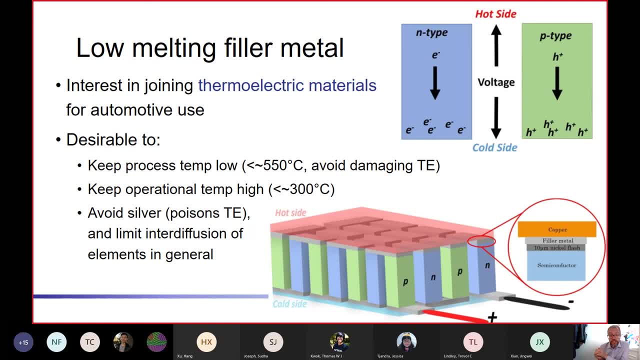 The best fillers to do this are the silver based ones. But the problem with that is the silver can diffuse through and interact with the thermoelectric and effectively poison it, changes it And it no longer has its design. It's a very desirable property. 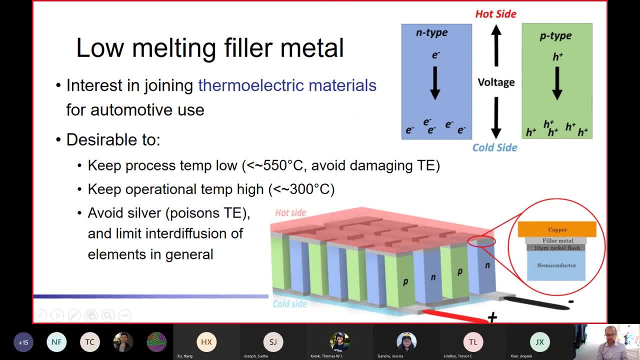 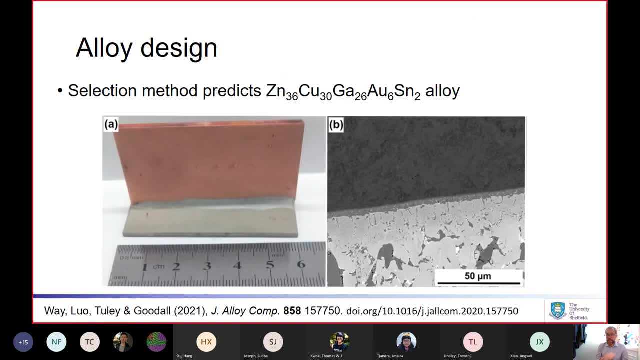 So there was a case for a bit of a redesign of the filler metals in this, in this situation, And that's what we did- We used our design approach and we came up with quite a novel composition of an alloy. Actually, there wasn't much data on some of these elements used together, but a zinc, copper, gallium, gold, tin alloy. 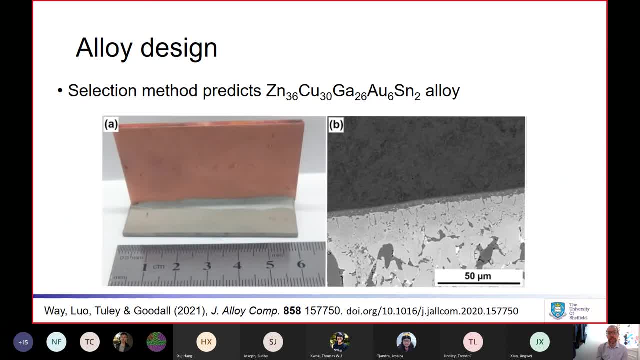 So the gold perhaps isn't super desirable from a cost point of view. But we tried composition. We did some applications without gold and they simply just weren't as good. There was a clear performance improvement with having the gold. So in the sort of applications this would be used in, you might put a nickel barrier, a diffusion barrier, on your thermoelectric and you want to combine that to a copper heat sink. 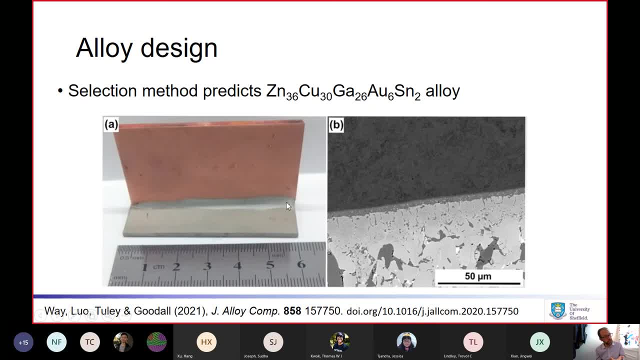 So we did some trials bonding nickel to copper And there's our filler in between and it bonds quite well. And looking at the interface, this is the copper side, This is the filler side. The interface actually looks quite good. There's not defects at the interface. 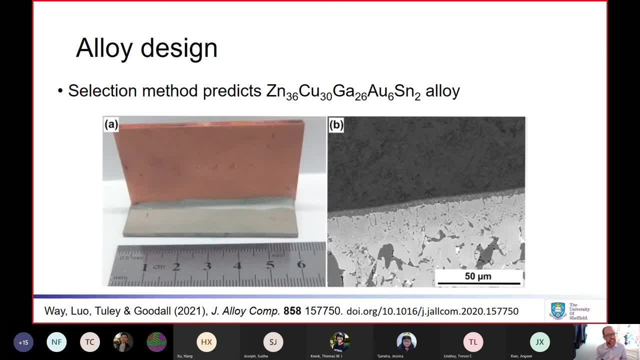 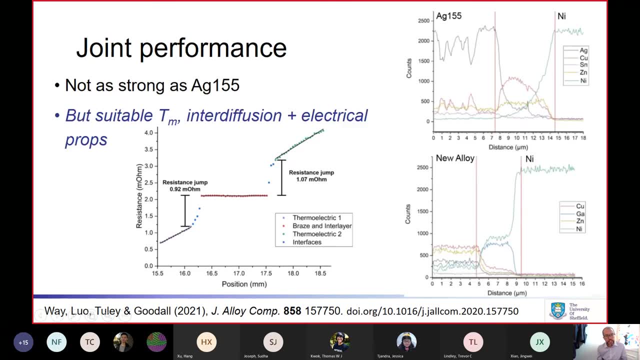 The alloy itself looks well. that's quite an interesting microstructure, let's say, But as a joint it looks reasonably good. When we probe the mechanical properties it's not as strong as the silver fillers, But this is not really an application where strength beyond a very much a base level to hold the component together. 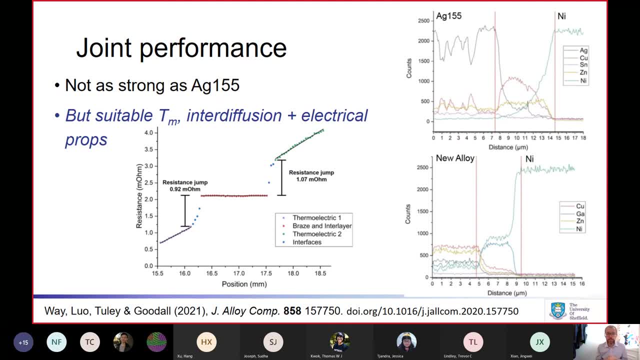 It's not a structural role, So the strength doesn't need to be super high. And when we compare interdiffusion or diffusion into the nickel from the silver based alloys, the conventional alloys and our new alloy, we're a little bit less. 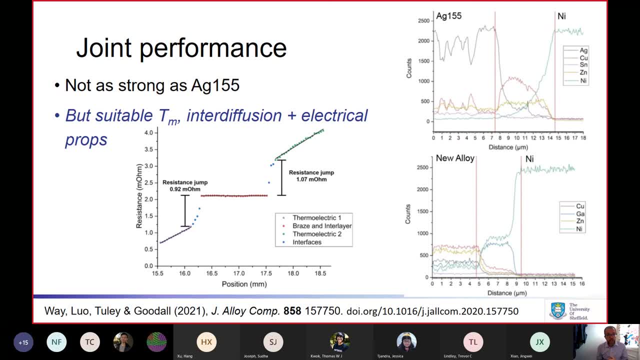 It's all quite small, but we're a little bit less. There's less going through And, probably most importantly, looking at the electrical performance, the resistance across that joint, which is what really matters for the efficiency and effectiveness of the thermoelectric. 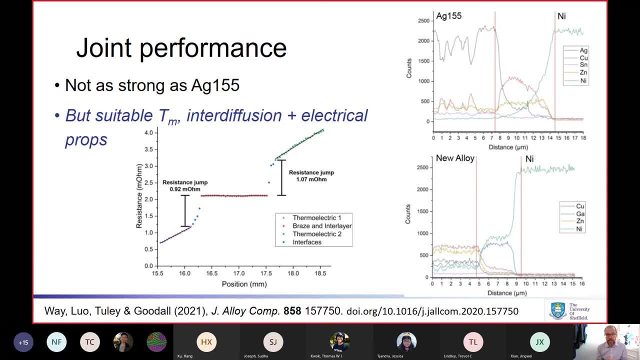 That's within the sort of the acceptable range. So that's an alloy that might well be suitable for that use once the full development of the thermoelectric materials themselves is completed. My third and final example is about moving towards higher temperature brazing. 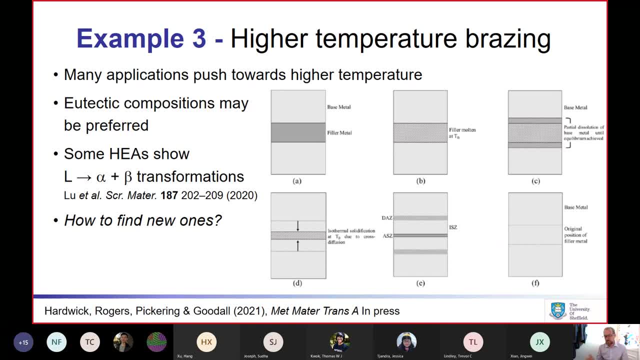 And there's obviously- and this is a common thing in many applications- You see it certainly in In aerospace, in nuclear, like fusion, things want to go towards higher temperatures, higher than the current technologies allow. You can relatively easily design a high temperature alloy, but for it to be a brazing alloy it's got to melt below the temperatures of the materials that you're using. 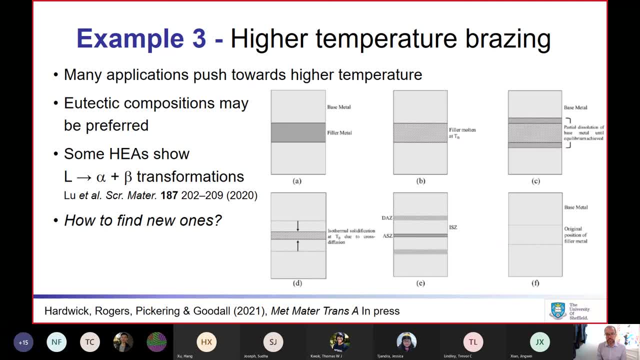 And for that reason we might be interested in eutectic composite compositions. Now that obviously lets us bring down the melting temperature. But another Advantage of a eutectic- particularly if it's a quite a deep eutectic, a steep sided eutectic- is if we can engineer some compositional change of the filler. we might make it so that actually, once it's done its job, there's no low melting temperature phase left in our material. 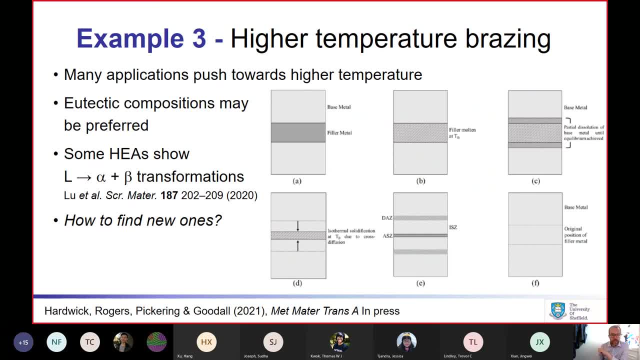 So I've tried to take, I've taken this sketch out of a paper that we wrote to try and illustrate this: If we imagine joining some, some base materials with a filler, We melt the filler and then perhaps, if we keep it molten, the filler might dissolve some of the base material or it might diffuse into the base material. 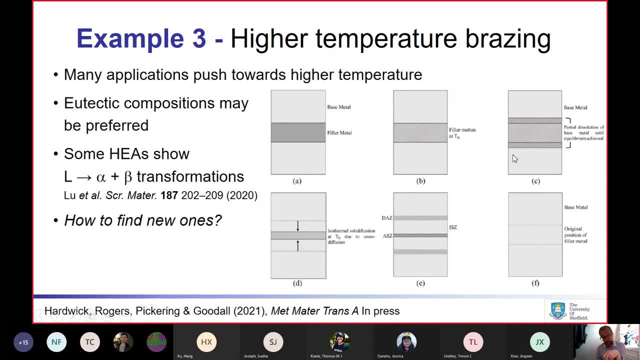 And as it does so, it's going to alter its composition. And if it's a deep eutectic, if we move away from that eutectic point, we may quite rapidly go to an area where the melting temperature is above the temperature that we're at. 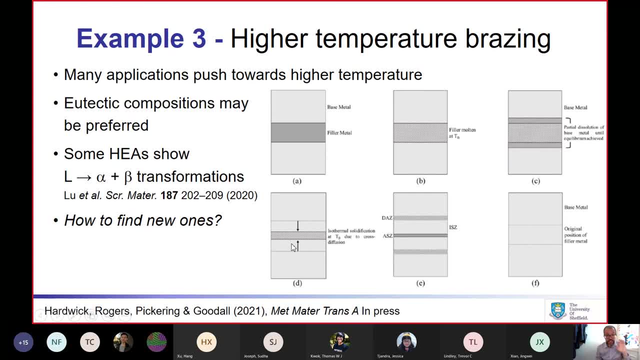 So we might see solidification in from the side At that at the brazing temperature, so isothermal solidification, and that could even proceed through until until we have full solidification, potentially if we leave it that long. So finding high temperature eutectics could be interesting. 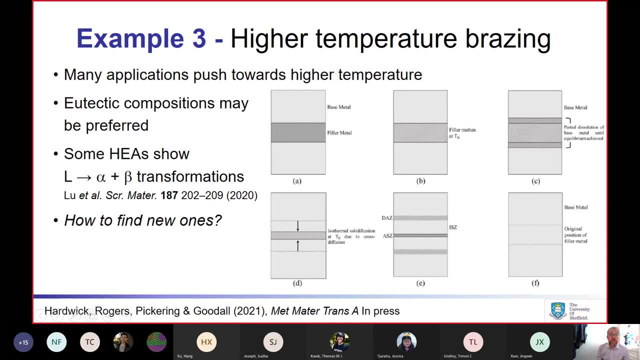 And it's noted, we noted- others have noted- that some high entropy alloys show liquid to alpha plus beta to two phase transition. And it's noted, we noted, that some high entropy alloys show liquid to alpha plus beta to two phase transition. So there could be some interesting eutectic HEAs that are out there that we want to find. 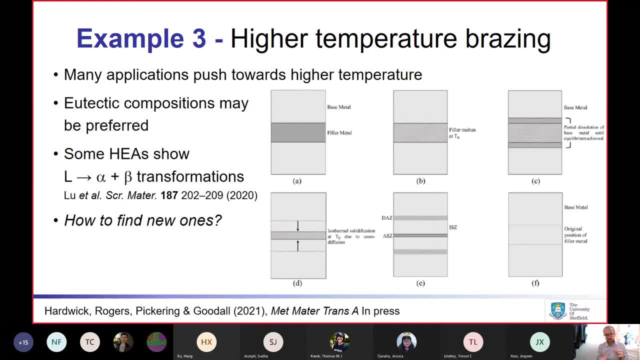 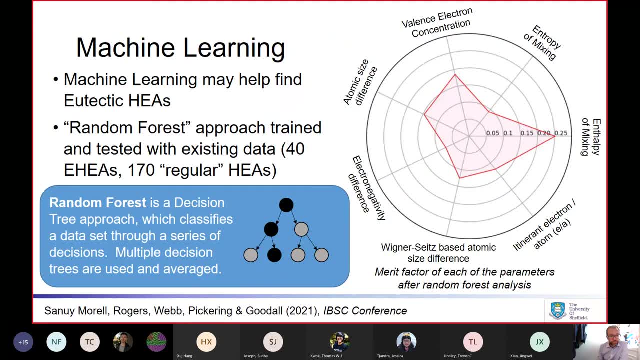 But how do we find them? Our previous search approach just tries to find alloys that are going to mix and form an alloy. It won't tell us if they're likely to be eutectic or not. So what we've been trying with this is we've been trying machine learning to see if it can help us. 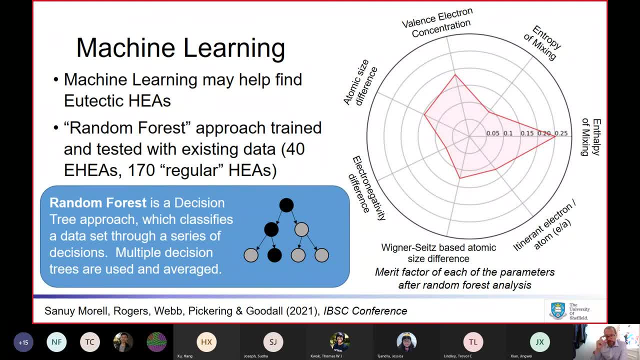 We've used a random forest approach, So this is a machine learning method. It's based on a decision tree. So in a decision tree you have a data set and you split that according to a dichotomous question, a question that can either be this or that. 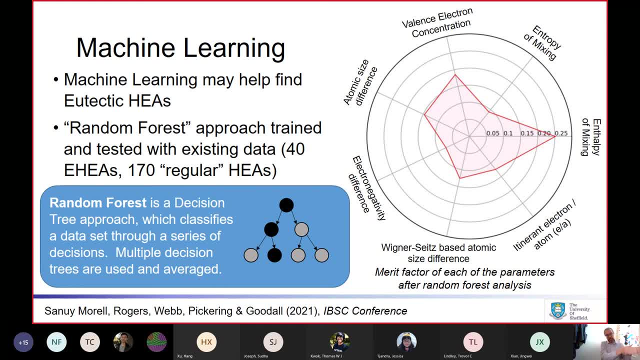 And then you take those groups and you split them again and you keep splitting until you have different subgroups with different characteristics. And you can use that to sort of see if you take a new alloy, if you're looking at alloys, if you take a new alloy through that approach, which of those subgroups it ends at. 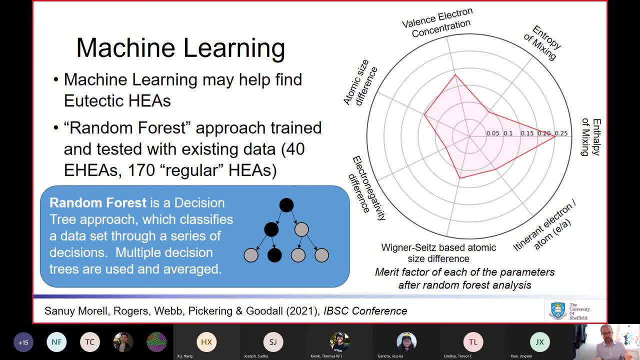 That's a decision tree And if you have lots of those, that makes a forest. And making a forest helps to sort of give a better overall prediction without over overfitting. So we tried this approach, this machine learning approach, With a data set of 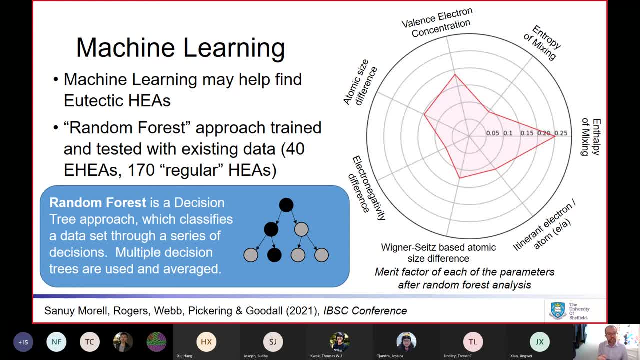 40 eutectic HEAs, which are the only ones that have been reported thus far, and 170 regular HEAs, And we found that, in terms of their importance to that, to that decision, the enthalpy of mixing was the most important characteristic. 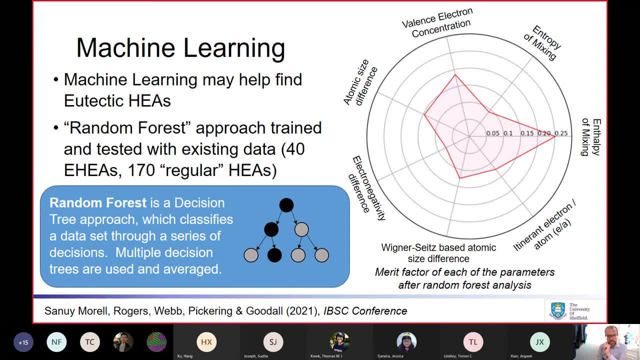 The valence electron concentration and the atomic size difference was probably the next one. So actually we're getting two of the criteria that we were using anyway for our alloy design, Plus the valence electron concentration as being the most important ones. So we've tried this. 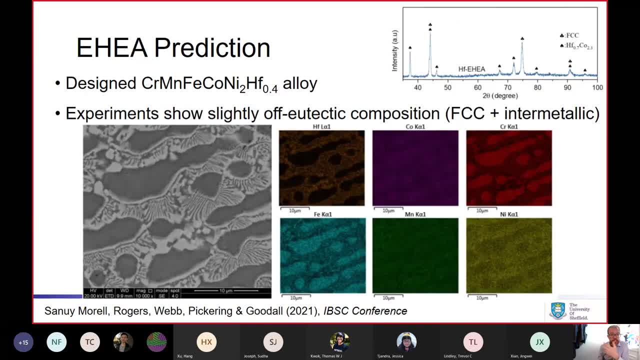 This is very much ongoing work, but we tried this out. We came up with a new alloy. In fact, we ended up with a six component alloy: chrome, manganese, iron, cobalt, nickel, hafnium. We've made this up based on those predictions and we found it's not perfect. 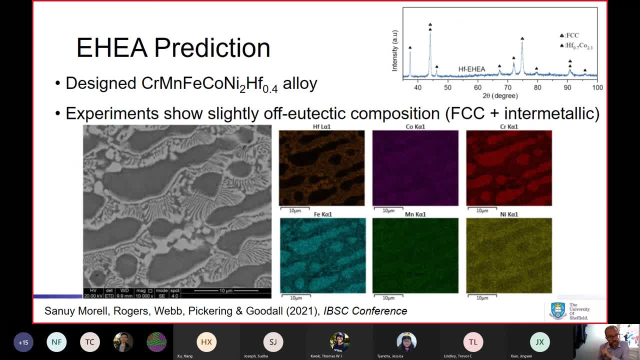 It's not exactly a eutectic. It looks like it's an off eutectic composition. So we've got some primary, a primary phase, which seems to be an FCC phase, And then our eutectic, which seems to be the FCC phase, plus an intermetallic. 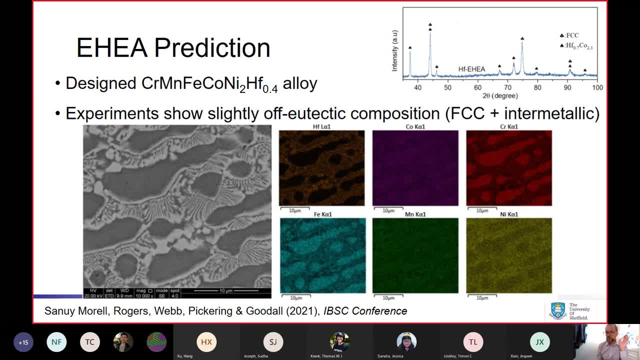 So it's not perfect And certainly this is not particularly optimized as a brazing filament yet, But it does look like we've got some clues as to ways of finding these eutectics And hopefully we can build on this and adapt our method to help us find some high-tech solutions. 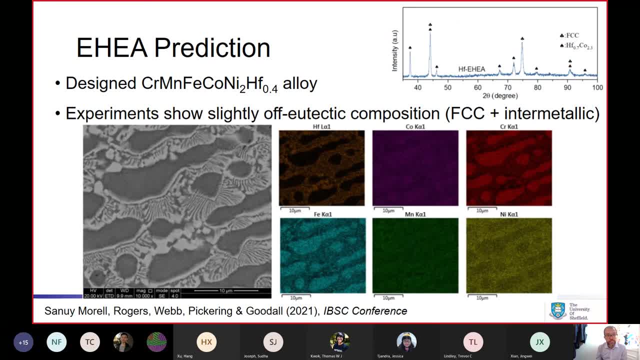 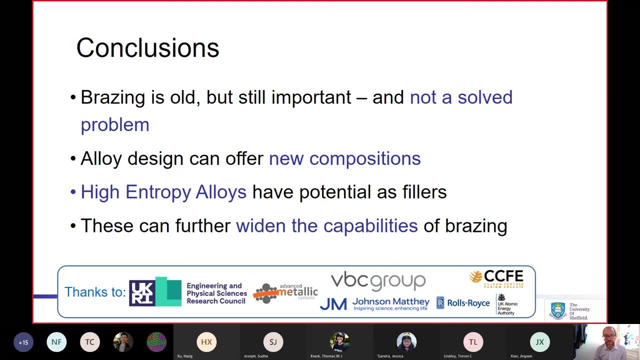 And hopefully we can find some high-temperature eutectics that can be used as fillers. So I'm very much coming to the end of even the extended time slot there, But fortunately I've reached my conclusions And really I simply to summarize to say that brazing is a very old technology. 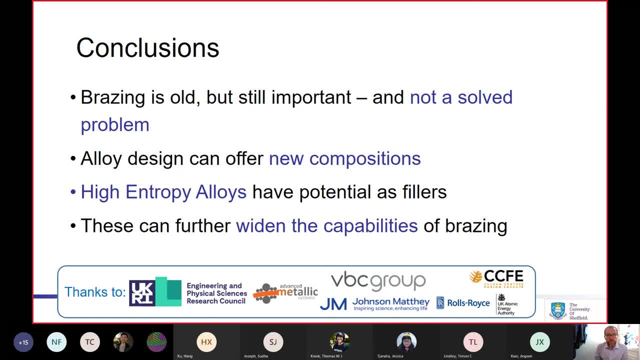 You probably would look at it in that way, But it's not a solved problem. We don't know everything about it yet. Modern alloy design techniques Drawing on ideas like Like machine learning, Like high entropy alloys, Can give us new compositions. 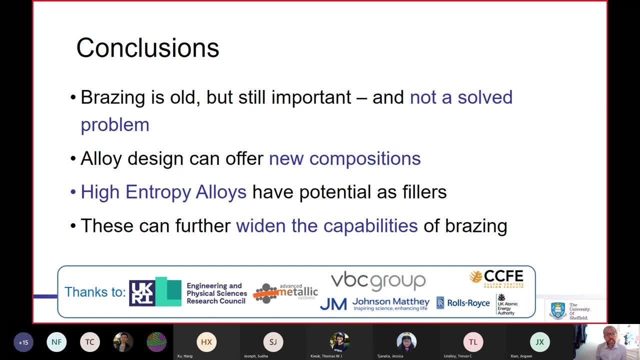 And the high entropy alloys certainly do have potential as fillers. There is a US company that has commercially introduced high entropy alloys as filler compositions, for example, And as far as I know, that's the only commercial application of high entropy alloys thus far. 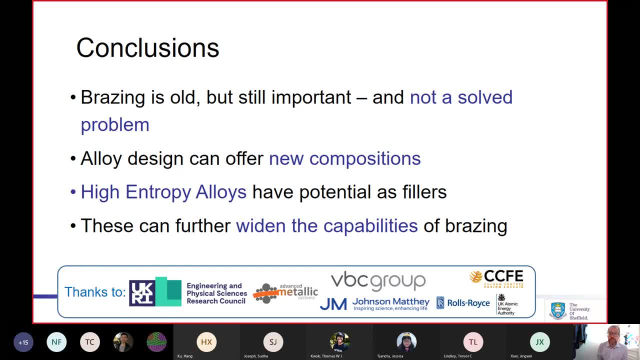 So this sort of approach is to widen the capabilities of brazing To bring it into areas- higher temperatures, lower temperatures, more demanding roles- where it's not currently being used. So with that, I will thank you very much for your attention. 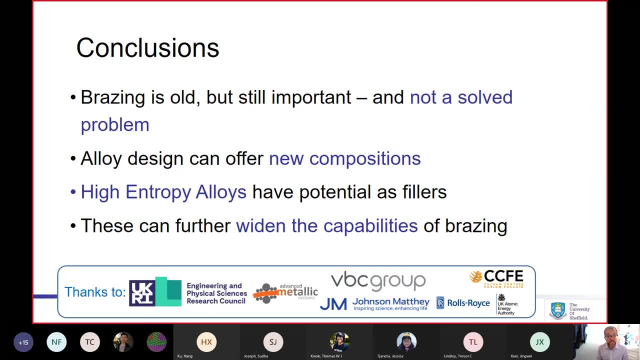 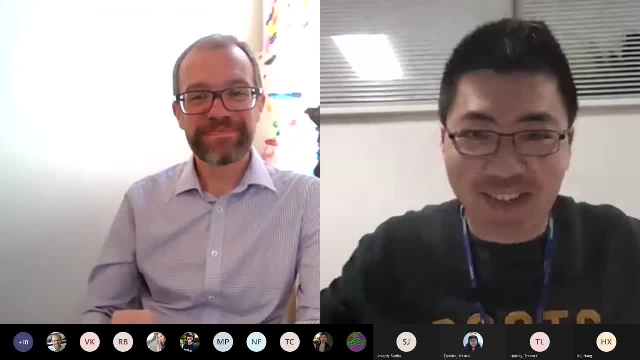 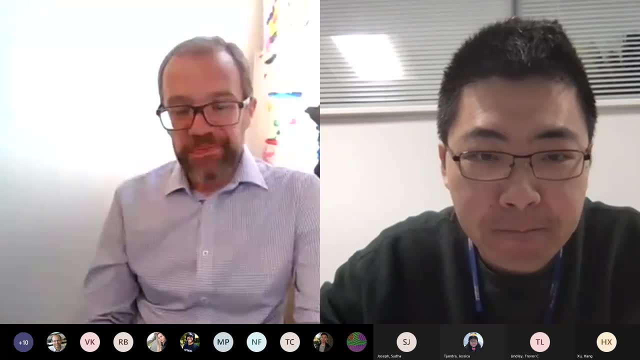 And, of course, invite any questions that anyone would like to ask. Great, Thank you very much, Professor Goodall. It was an excellent talk. Thank you, Does any one of us have any questions? Yeah, So can I ask the first one? 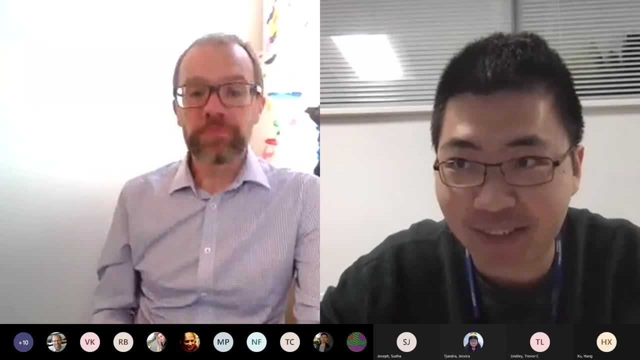 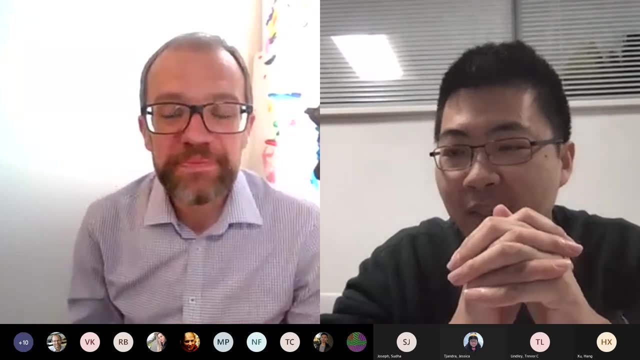 Because we are working on- like I am working on- some soldering stuff And so it's relatively related. So, even like for the last example you've shown, if we managed to get a eutectic composition, and where would the intermetallic go? 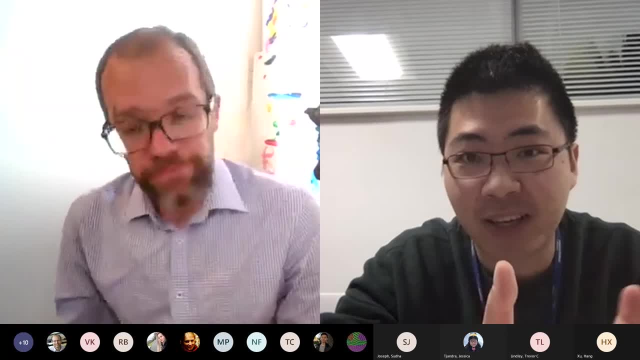 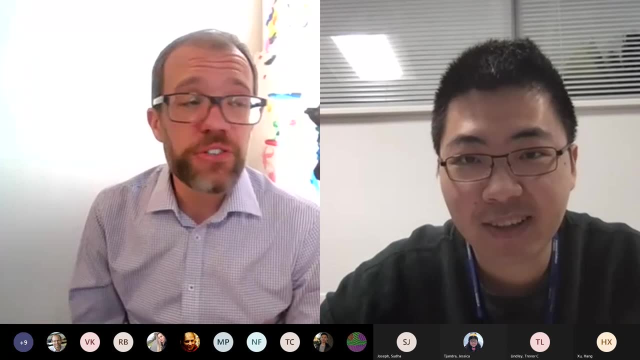 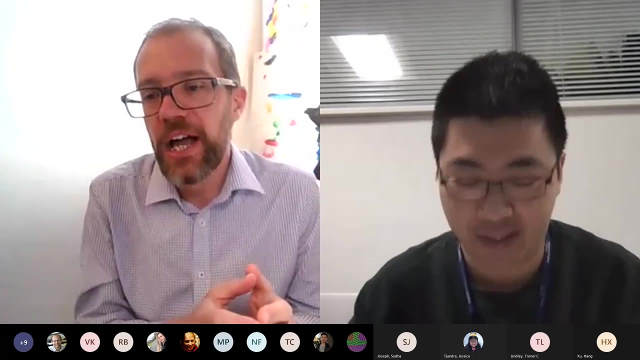 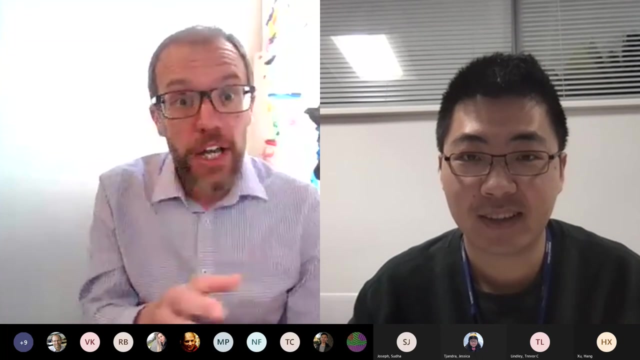 Will they disappear Or they will be in the eutectic? No, that's true. So it's a different strategy, I guess. So each of those examples is a different area, a different solution to a different problem, And that is very much the way that these technologies are. 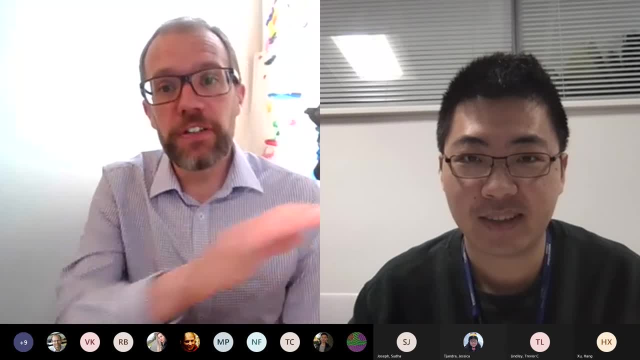 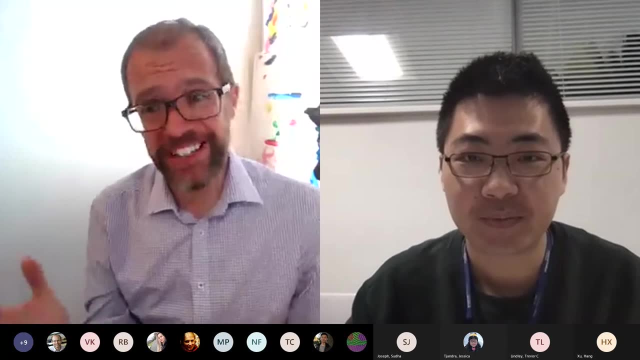 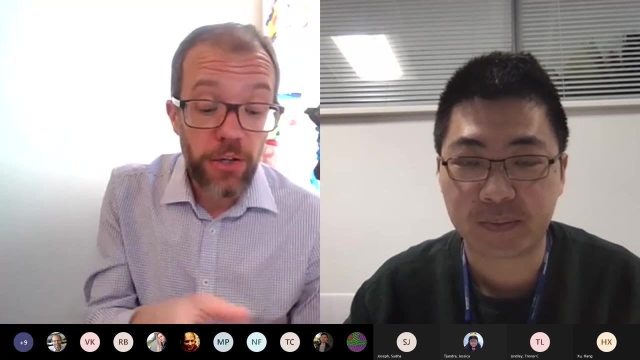 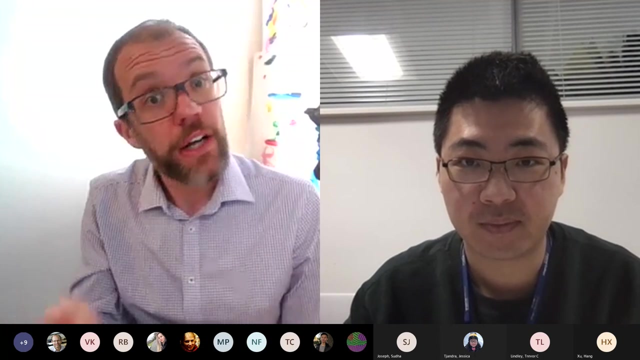 All these different filamentals are adapted for a different use. There is no one this will do everything, And nor could there be really, because the requirements are different. So it might be that a eutectic alloy could be, of course, less strong if the intermetallic in it is less strong. 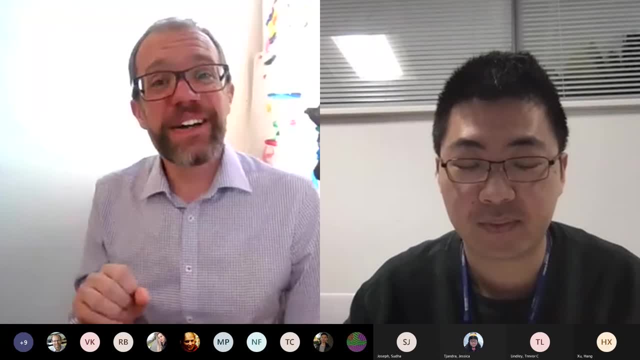 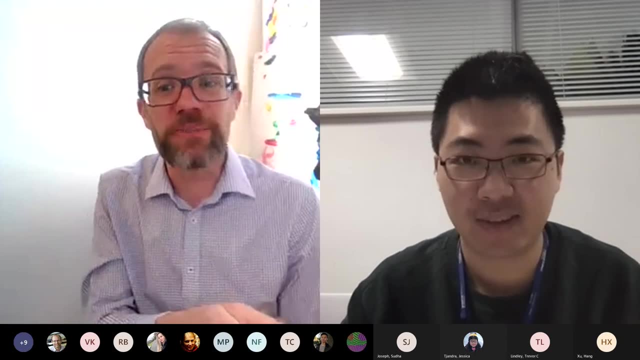 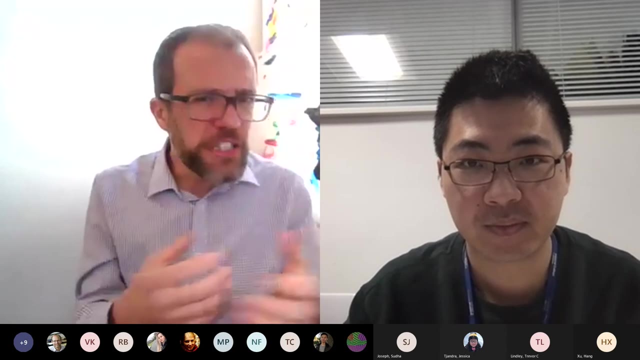 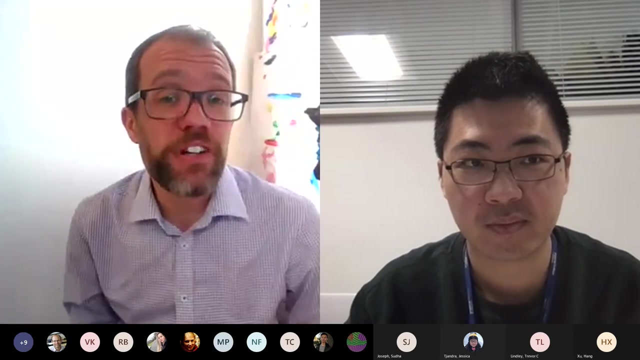 However, we do work with in conventional metallurgy as well as in fillers. we do work with eutectics and get good properties out of them sometimes. But if it can be coupled up with the right kind of process control and the right kind of quantities of the intermetallic, it could even be an advantage to have that sort of two-phase microstructure. 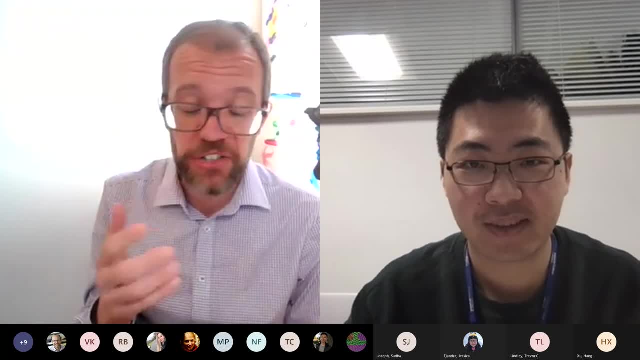 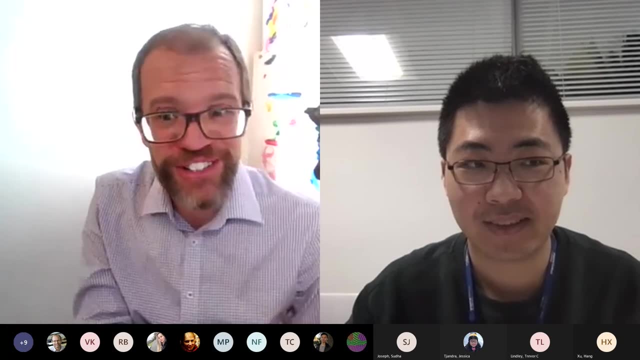 It depends, like any kind of decision you make about a phase in a material, it depends where it is, what size it's in, what the microstructure is like, whether it's going to be good or bad. Yeah, Thank you. 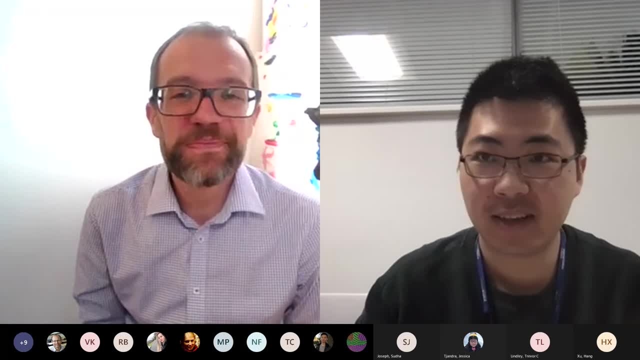 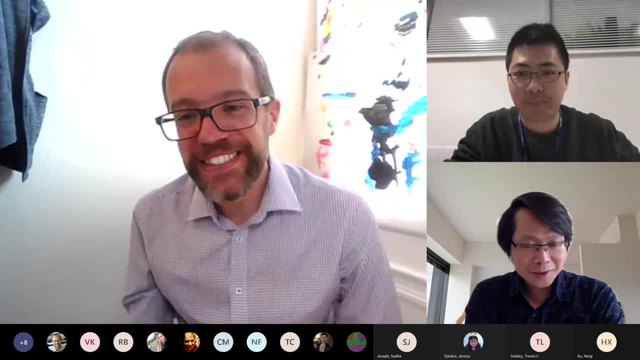 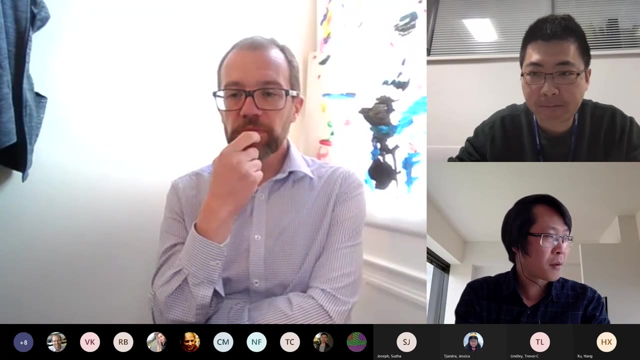 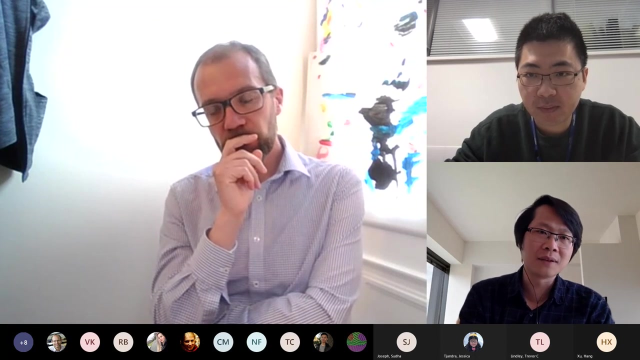 Yeah, Sam, please. Thank you very much, Russell. That's a fantastic talk. Just curious about high-temperature brazing in particular, like with boride. Boride to some extent could be kind of a beneficial element, in particular for high-temperature, like a creep resistance. 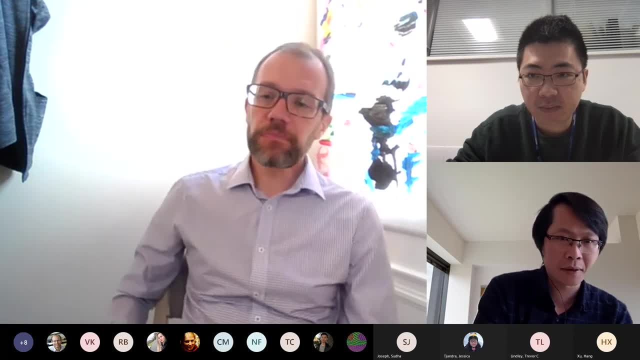 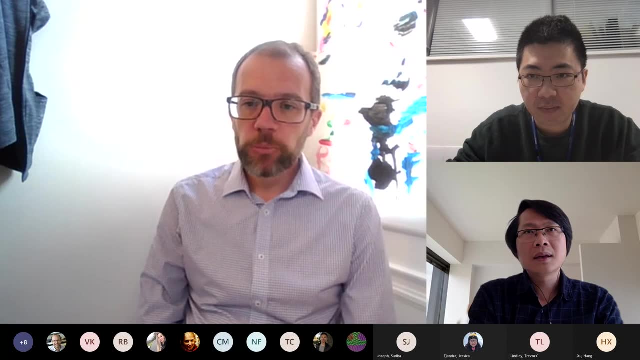 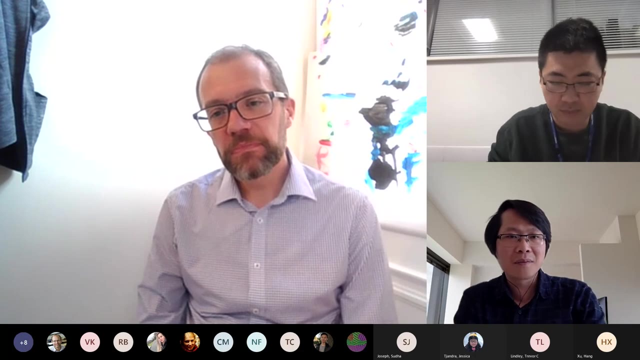 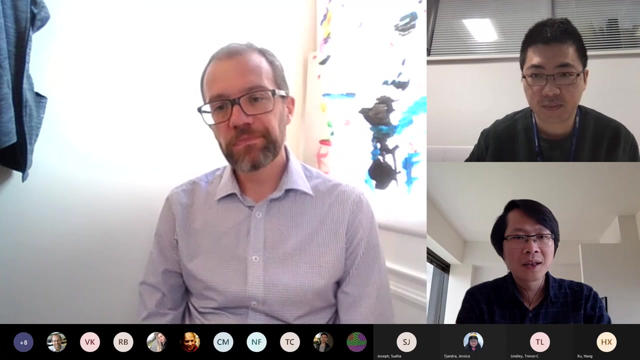 We all know we want to add more boride, We want to increase the creep strength. So when we want to design high-temperature brazing, do you think like a boride? certainly we don't want to have a kind of big boride, but we want to kind of diffuse boron to grain barriers and with that we might be able to increase the creep resistance, for example. 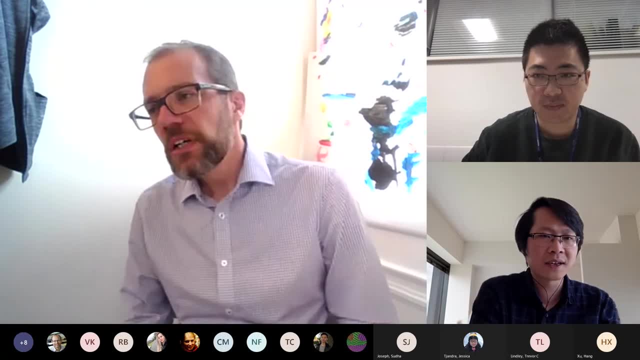 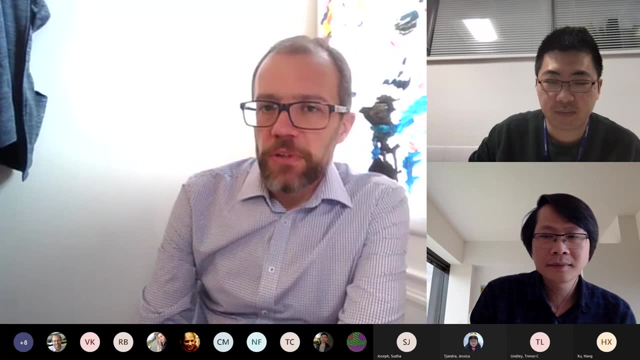 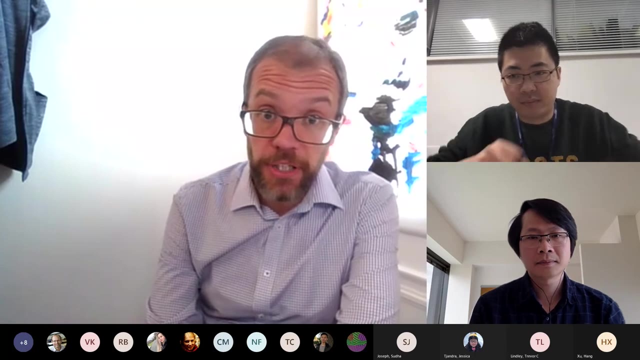 Have you looked into that kind of effect from kind of added elements that might bring some kind of additional benefits? So yeah, we've looked at a number of different compositions. As you saw from what I showed there, we've not totally removed the boron. 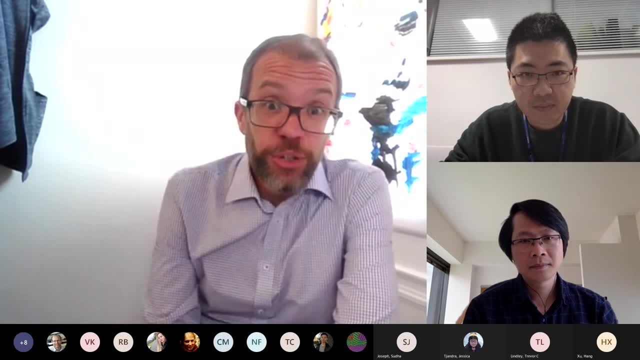 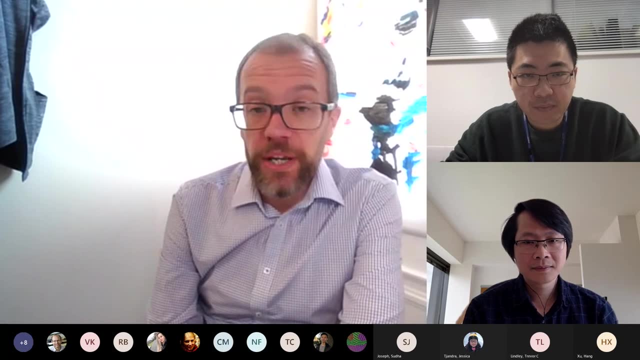 We're still actually, compared to conventional super alloy type material, we're still at a pretty high level of boron. So we certainly haven't taken that out And we have done a bit of work on looking at exact, trying to diagnose it. 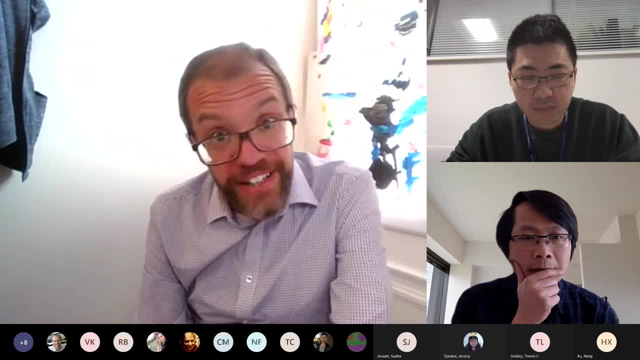 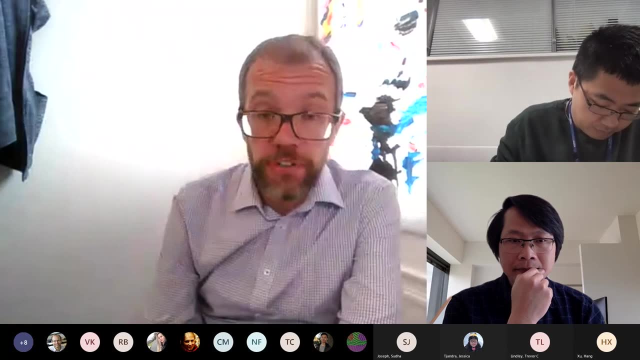 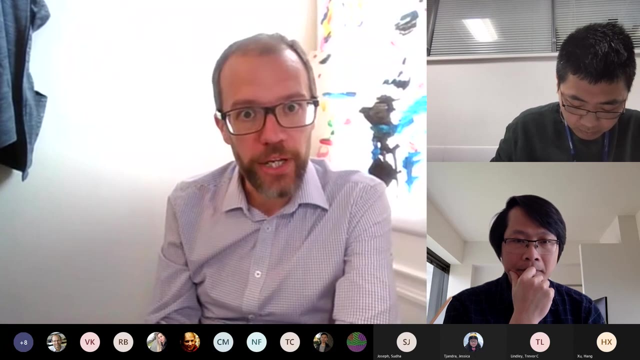 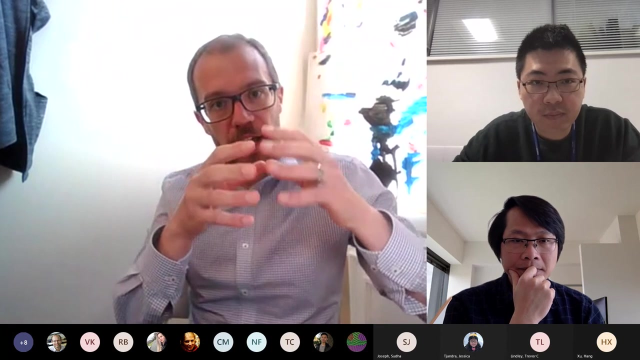 Exactly where it ends up and whether it is in good places or not. The mechanism of the diffusion of boron, which we did not, absolutely we did not invent- This is the normal expectation with the nickel brazes in particular- is that there'll be a concentration of boron to lower the melting temperature. 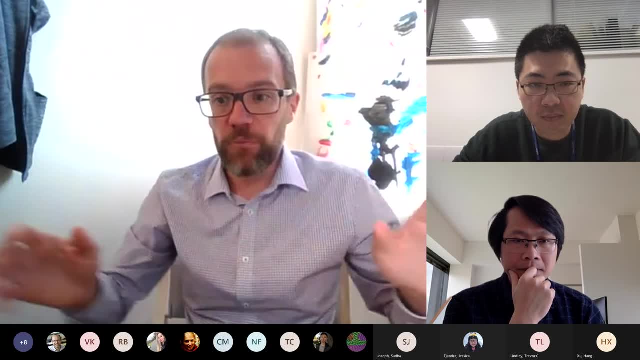 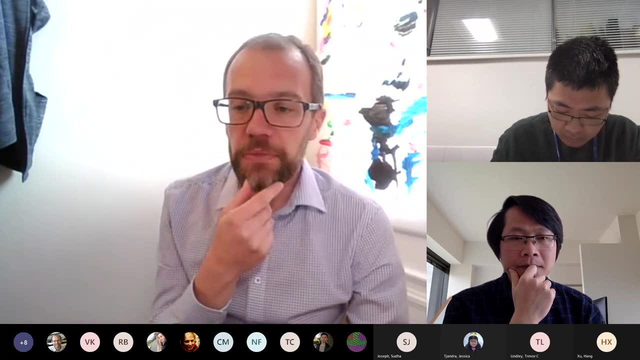 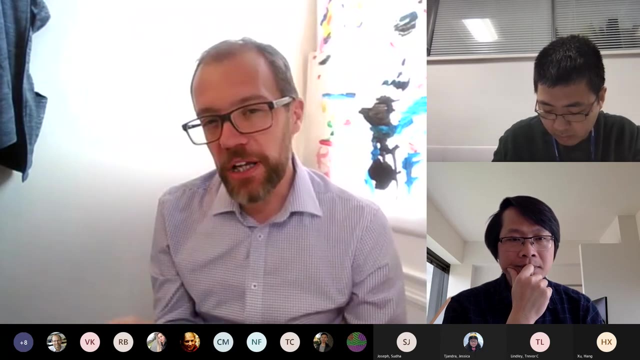 But then it will diffuse out into the ground And then we'll have the material where it's relatively tolerable to have it. So that is part of the accepted sort of process. Now, whether there's other elements that could be introduced into a filler, perhaps not necessarily for the immediate benefit of the filler in performing its role. 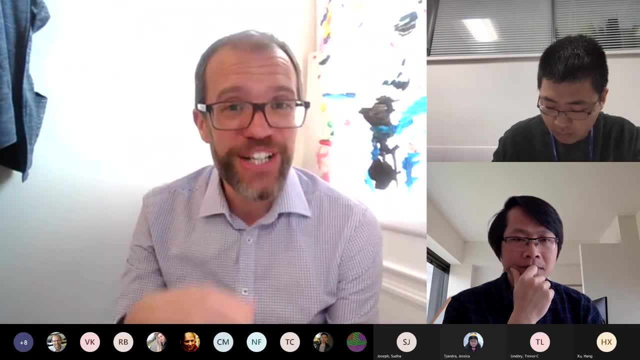 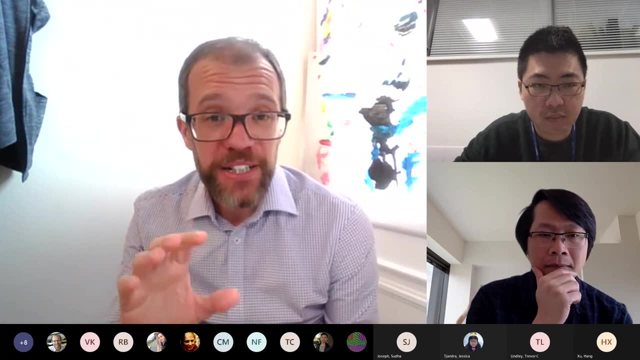 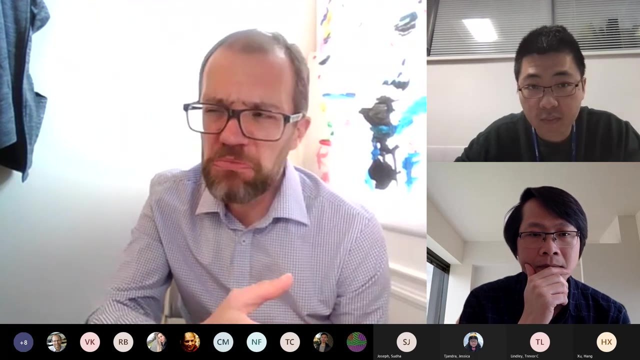 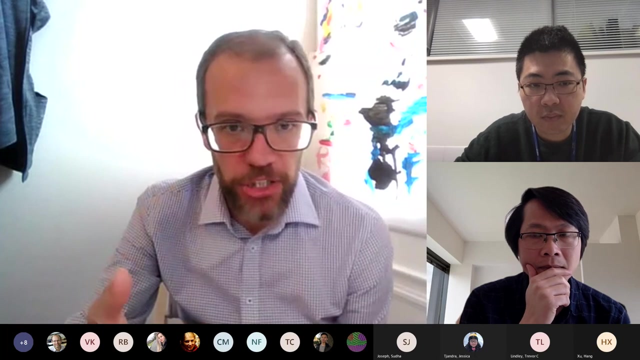 but the longer term benefit of the joint or the alloy around the joint? That's a very interesting question. Of course, the mobility there is of different elements for the durations that the bonding takes place is relatively low. We've certainly seen things coming the other way though, possibly because of some dissolution of the pair of materials. 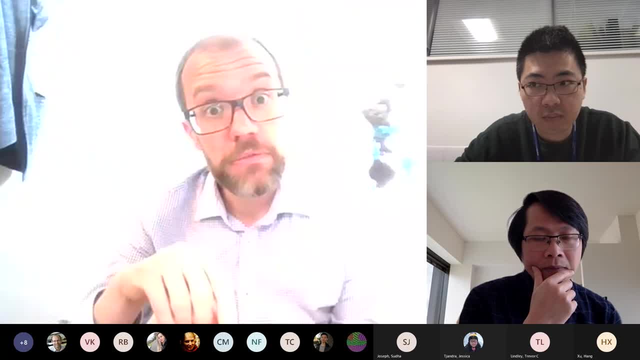 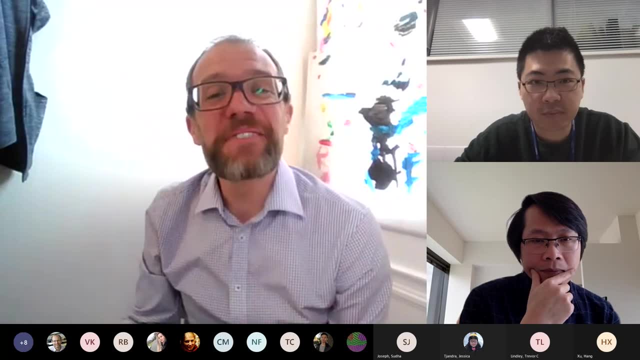 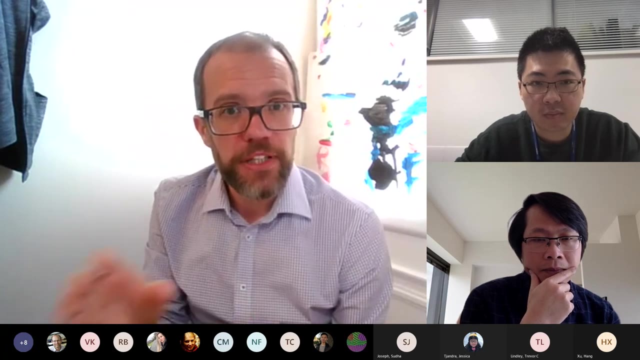 So we get niobium phases in the joint after the process, which obviously there's no niobium in our filler, but it's coming from the 718.. Now that's another area that we want to look at to see whether that's a positive or a negative because of how it's turning out. 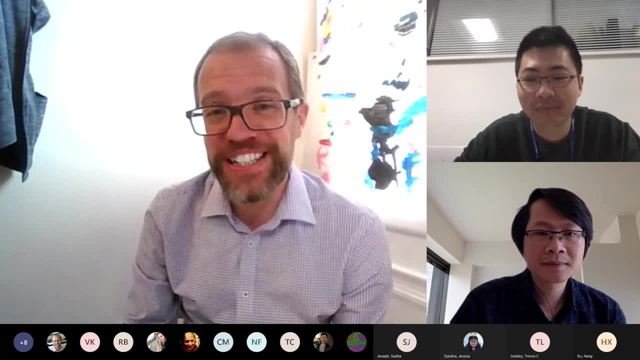 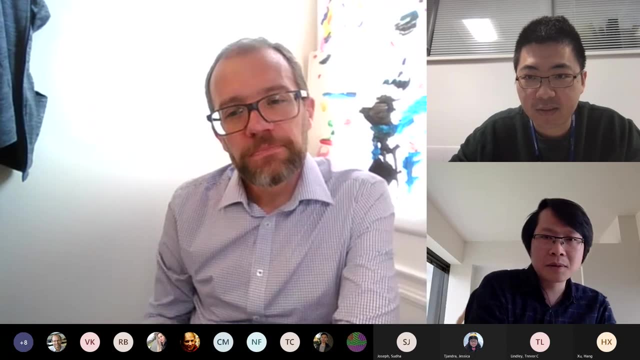 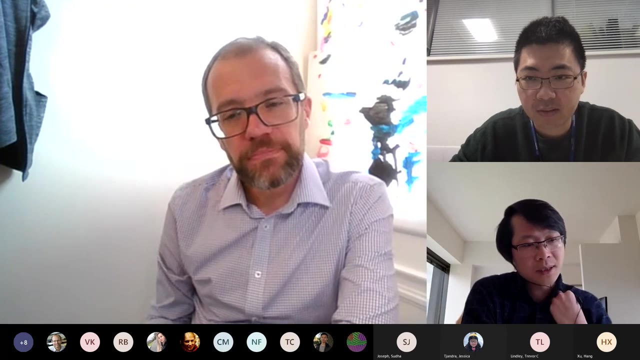 So there's definitely a lot of scope for more detailed understanding of that, Absolutely Yeah, that's fantastic. We have one collaboration with COLUMN to understand the structure, integrity of the unit. a brazed, brazing um and basically we just got brazed um joined between um p91, which is a 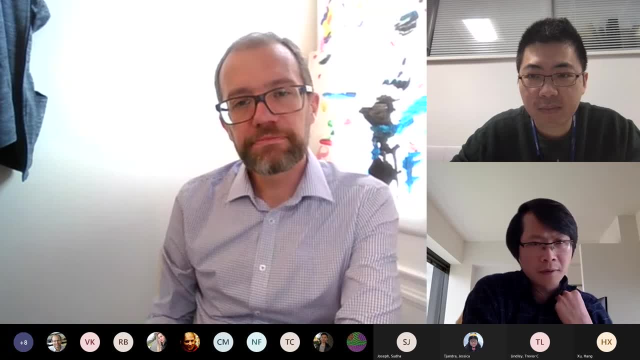 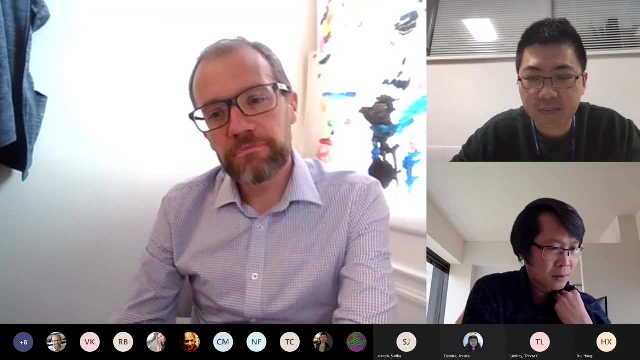 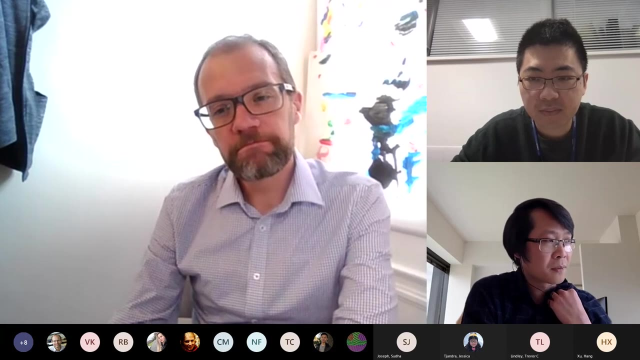 martin sticks and steel and um, it'll fail- kind of steel for fusion, um, very similar to p91, and also tungsten as well, um. so we want to understand the creep fatigue interaction of that joint and i just curious about the kind of when we hit it up and let the elements diffuse. 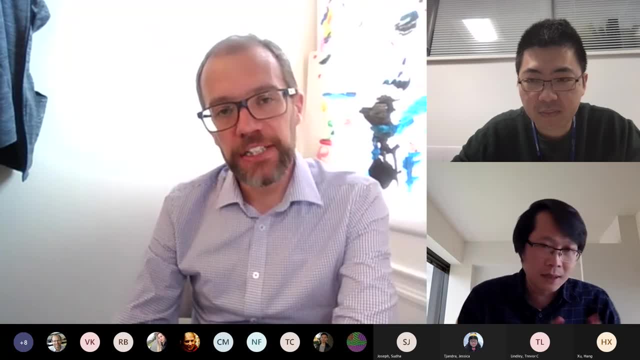 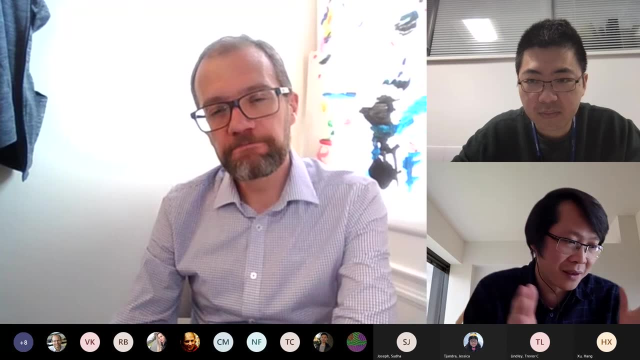 and that would have fight the the grip resistance. but say boron or some other elements, uh, and that might be. i mean with the hand, hand to be alloys. certainly we don't know whether hand to be alloy can reduce the diffusion or increase the diffusion. we don't know. 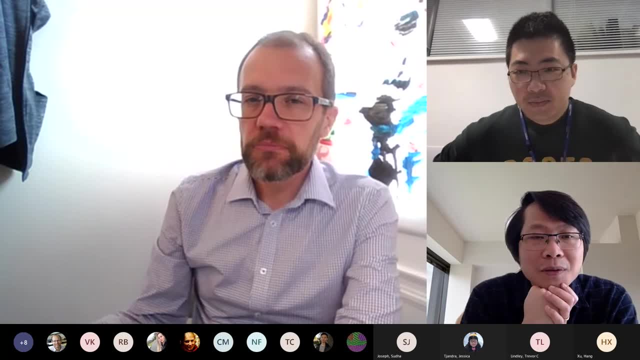 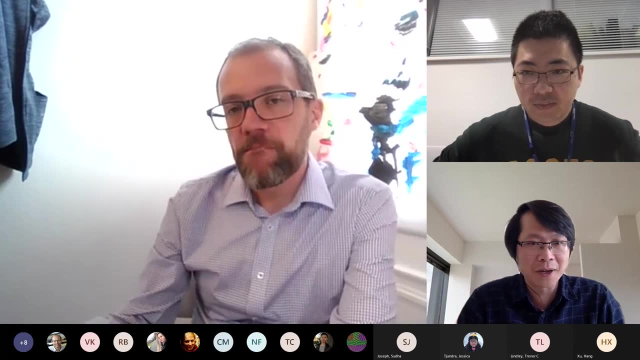 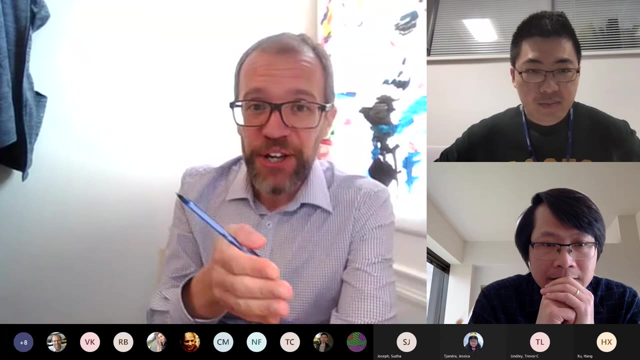 yeah, so. so that would be a very exciting direction to to look further, uh, in particular when you identify an ideal: um, yes, for for soldering, yeah, yeah, no, absolutely i think. i think that that sort of thing is really would be, is really valuable, the, the the longer term. 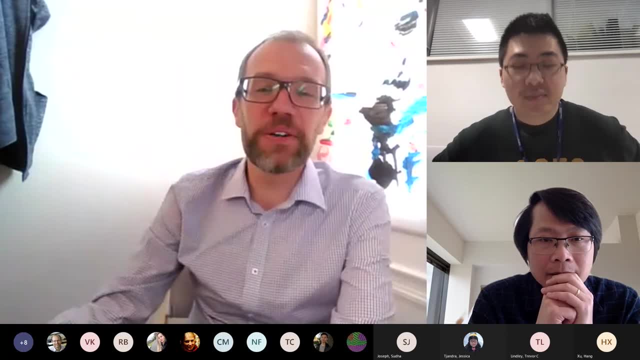 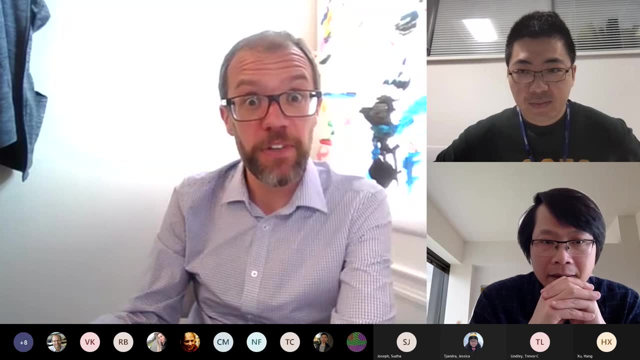 understanding to feed back into that, that, uh, that process, more of the knowledge for the design, the design loop and things like that- what is what's good to have and what's not good to have. yeah, yeah, yeah, yeah, yeah, yeah, that's right, but yeah, fantastic work, uh, russell. yeah, thank you. 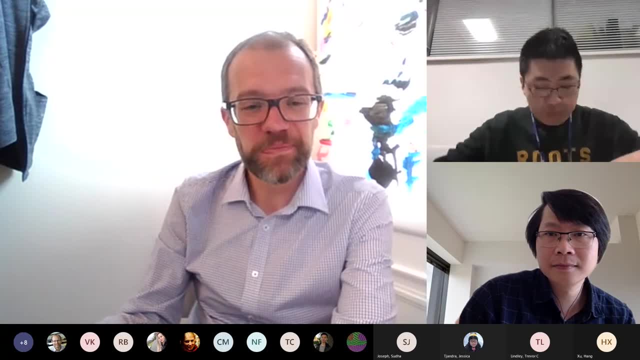 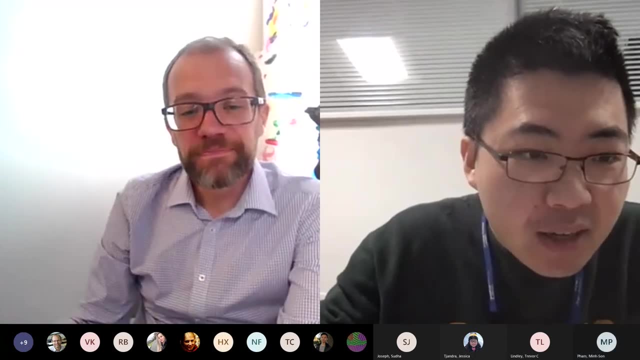 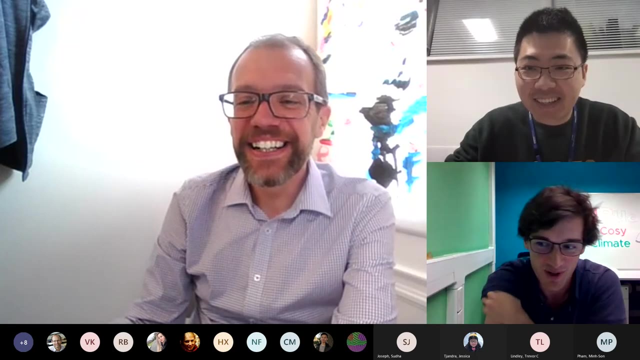 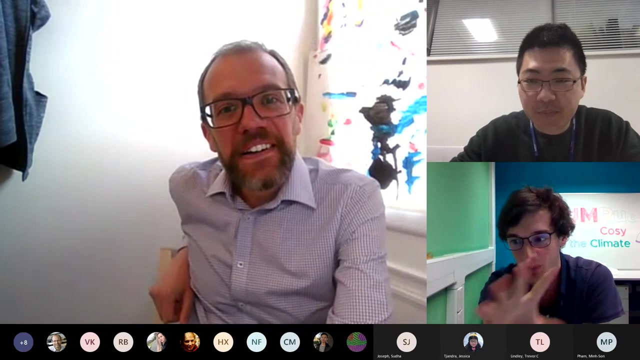 another questions guys. yes, please- i can't see who is okay- yes, please, uh. yeah, actually i'm the phd working with calum on uh, on fusion application of raising, so i thought i'll give my input. yes, um, i mean uh. so i'm more on the mechanical, mechanical engineering perspective: preparation of particular 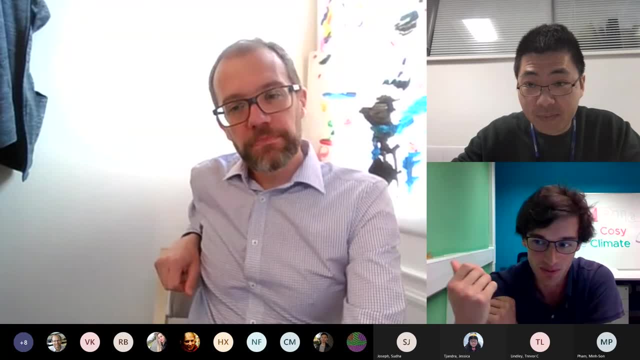 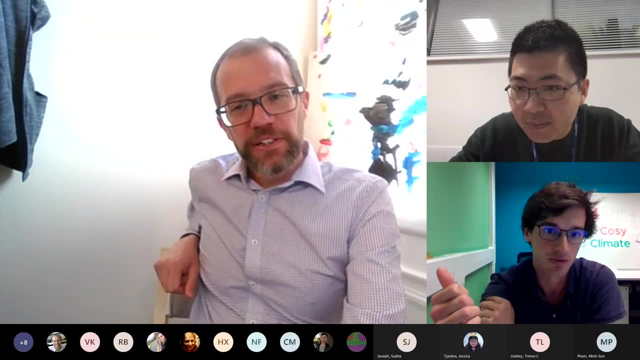 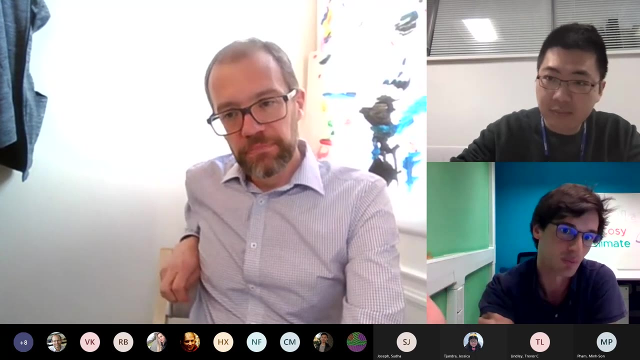 pieces. but i've got two questions that i ask to people. but no, bracing is uh, what are the best elements for? if you know about those like, but have good affinity with tungsten? uh, because tungsten is very high temperature metal and because of that there's a lack of diffusion when you melting alloy. 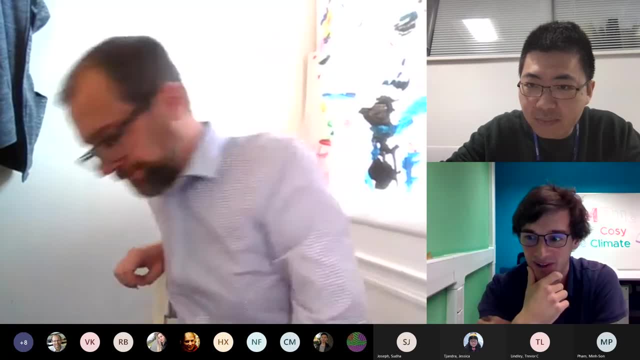 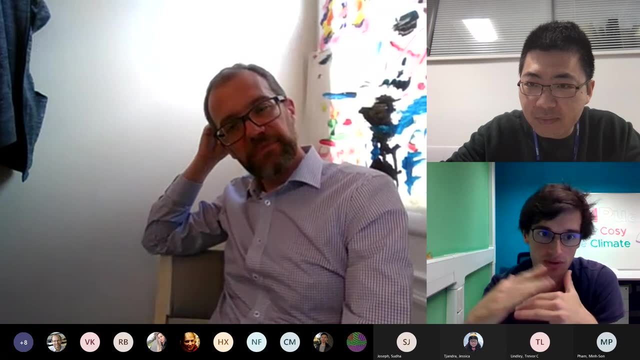 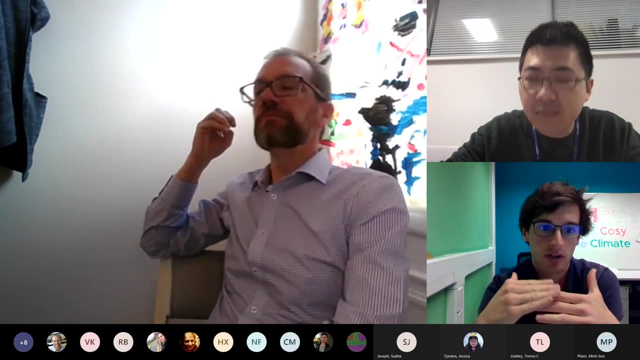 so i mean, i've i've found a few, but i would like your uh knowledge of that. and also, um, do you have only ideas how to make braze yawns as thick as possible? because even though you lose some mechanical properties, you can accommodate some more thermal stresses. so it's very 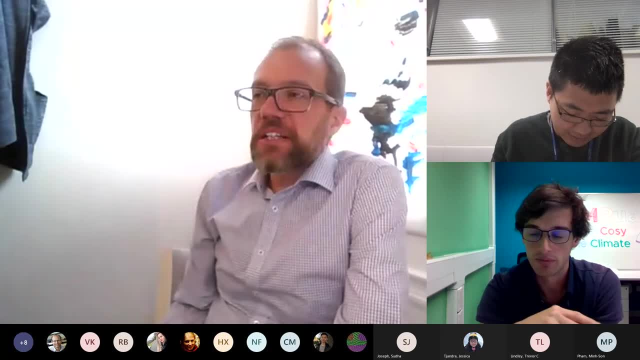 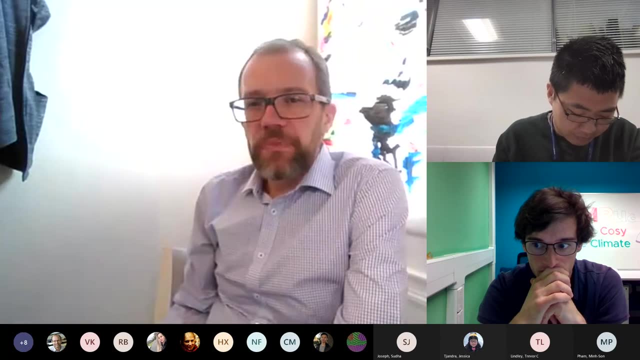 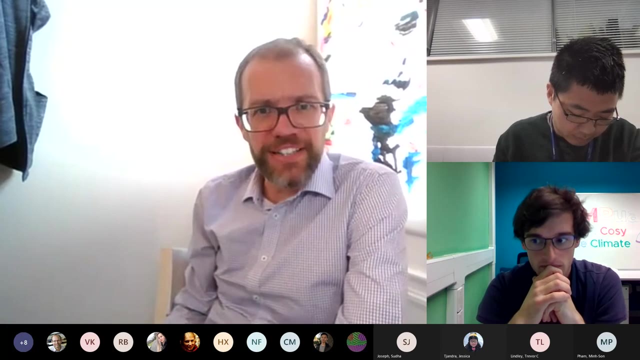 complex, but you can, i mean yes, so there's. yeah, those are both very good questions um where, um, so um, there there are, as you've probably found out, i think, gold based uh fillers can be used on tungsten, which is fantastic. it's always always the expensive things that solve the problem. 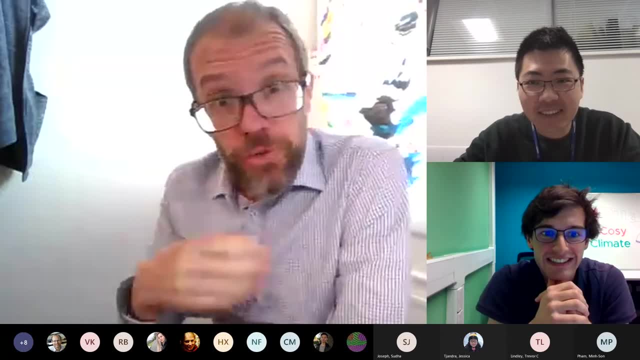 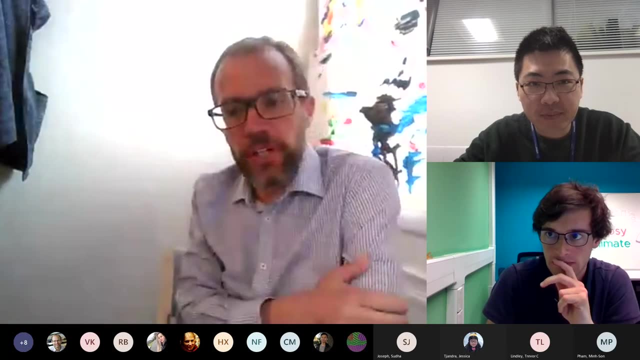 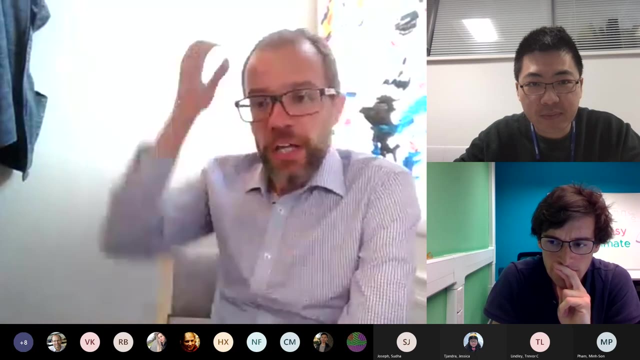 um, the other, the other, the other route or the route that's often used, where things are difficult to uh, to braze, difficult to join um you, you can move into an area called active brazing. so you don't necessarily need interdiffusion, as i showed on the one of the slides in there. if you, if you. 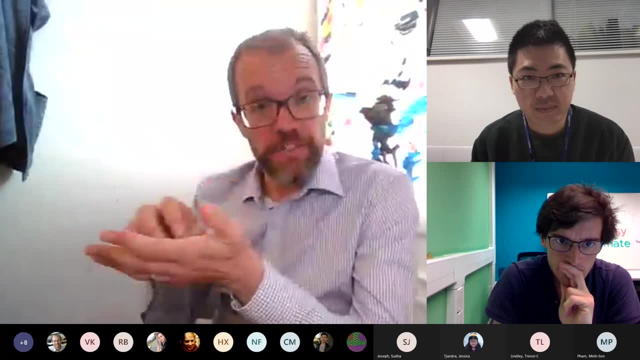 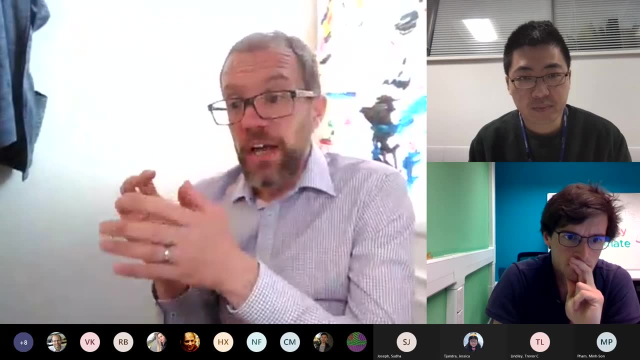 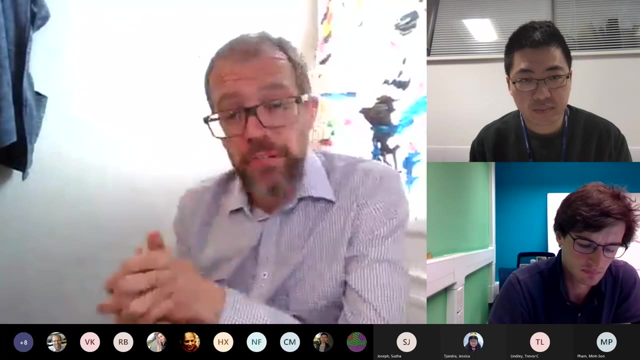 get an interaction, uh, a reaction that can be enough that can stimulate wetting. this is this is why we can braze ceramics. there's no diffusion, but there's a reaction. um so active metal brazing takes a filler that is has all the right properties but perhaps doesn't wet very well. 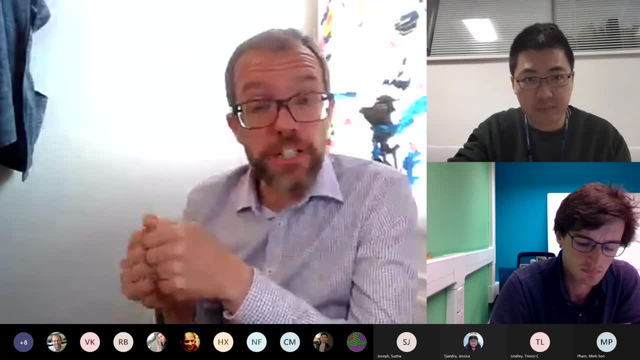 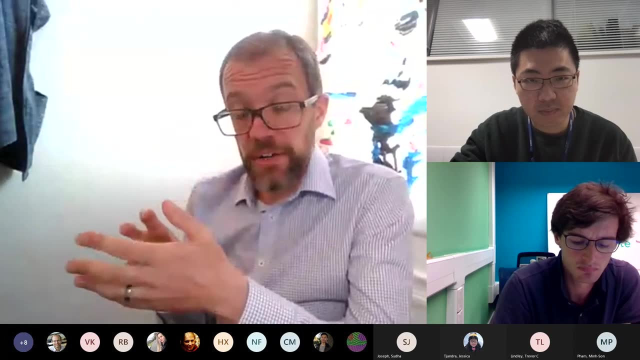 and then introduces a reactive element. uh, often it's titanium, but people have used hafnium, zirconium, things like that as well, and that sort of uh. the idea would be to remove the あすきをつぶして in the. in the metal it goes to the. 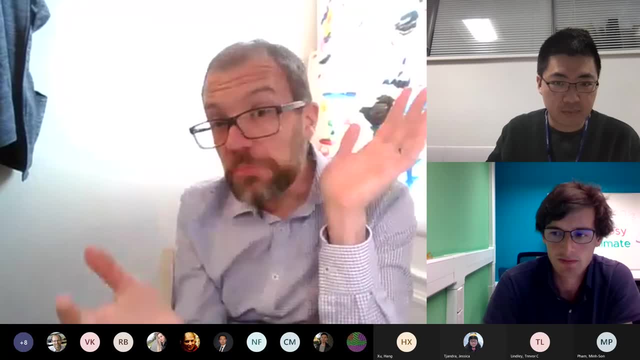 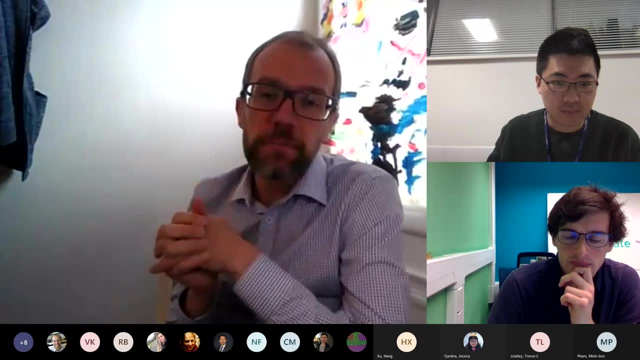 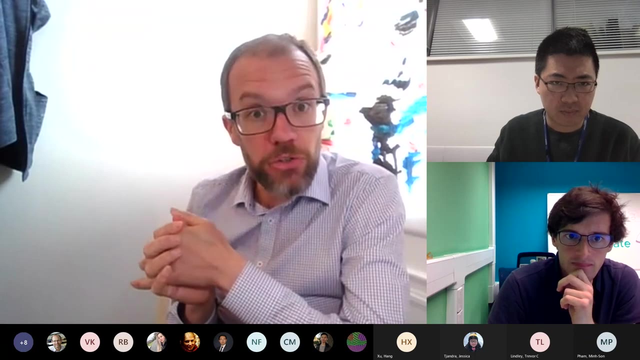 surface. it reacts with the, the material there forms compounds or joints or over bonds of some kind, and promotes the wetting. and if you get good wetting you should get good um one thing, that's the theory. um, i'm not aware of people you having used that for, uh, for those kind of joints, but it 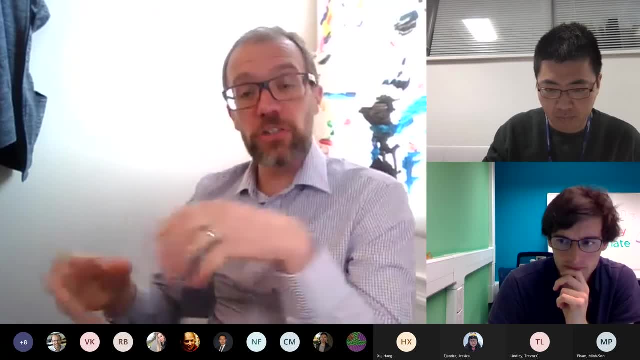 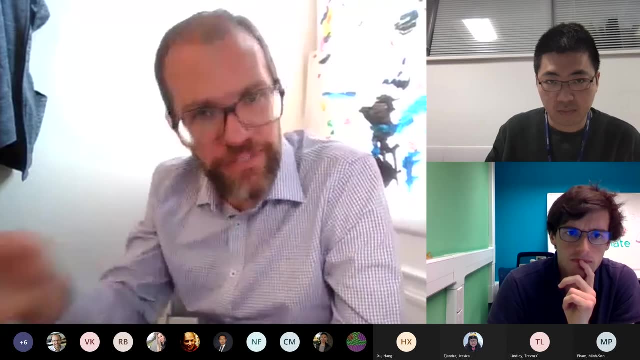 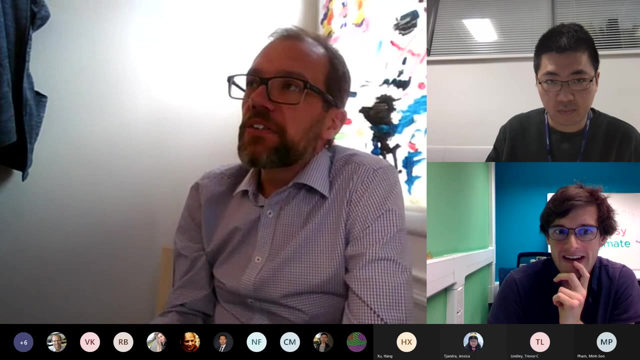 would certainly be. that would certainly be a route uh of exploration. because it would have to be a, because it opens up quite a broad array of uh design possibilities, notwithstanding the limitations that fusion um applies to it. yeah, uh, for the uh, the second part of the question. 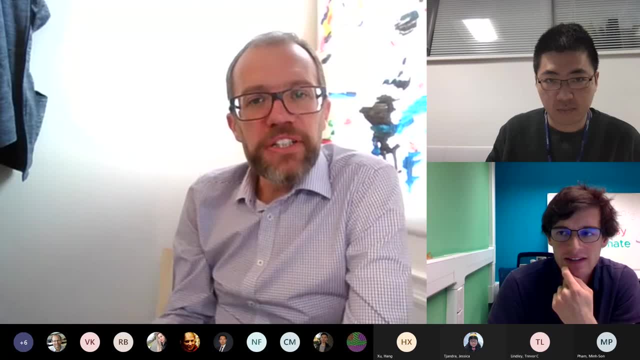 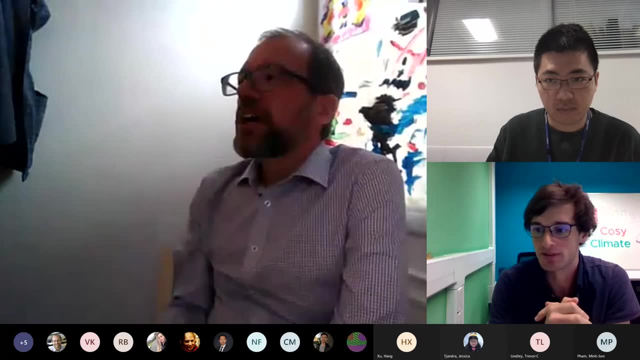 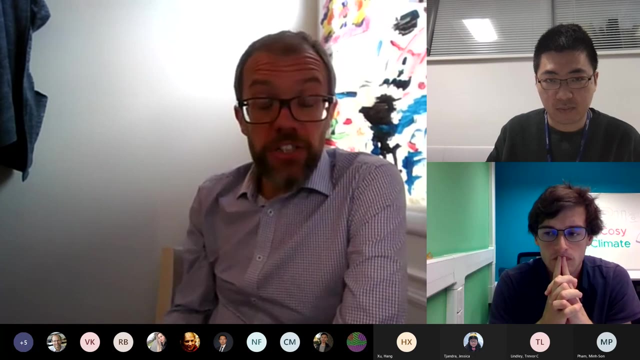 um, well, sorry, can you remind what was the? what exactly were you? yeah, i mean, it's more. we're trying to get the drawing to speak as possible, but there's some thermal stresses and yeah, so there is a. uh, there's different ways of approaching that. one is to, one is one route. 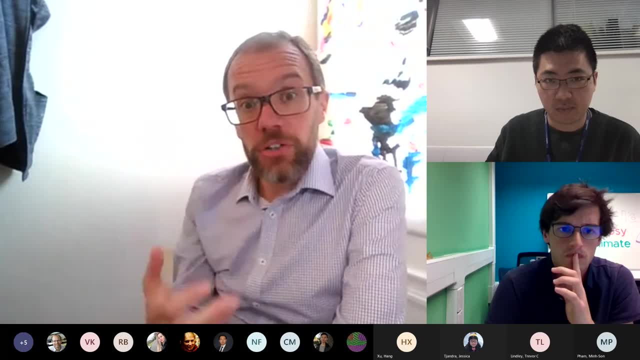 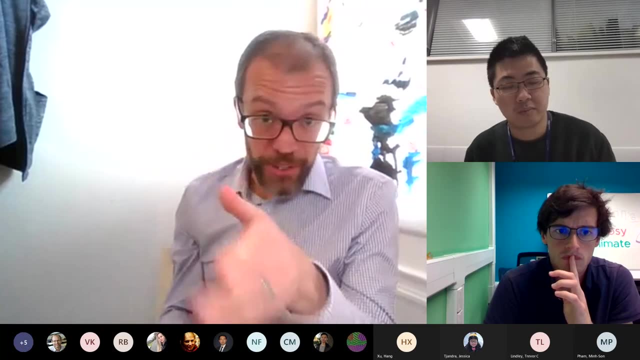 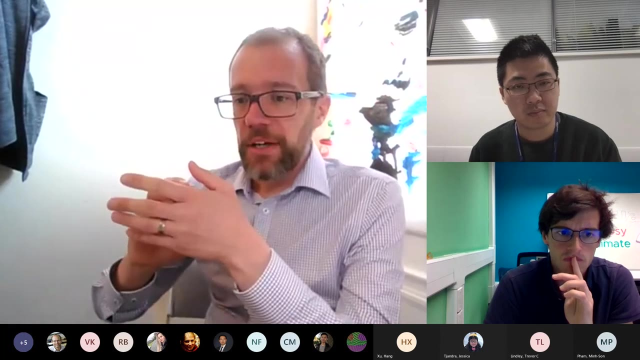 that sometimes people use is to have a joint that is not capable of having a thin- uh, a thin gap. so, um, some of the work that we're doing is looking at the brazing of additively manufactured components. now, um, the conventional wisdom, i suppose, for brazing to be good in that situation. 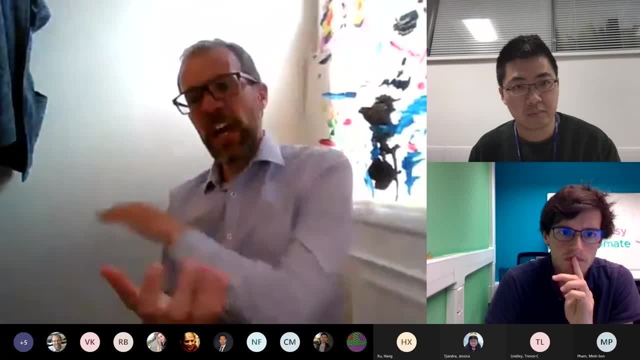 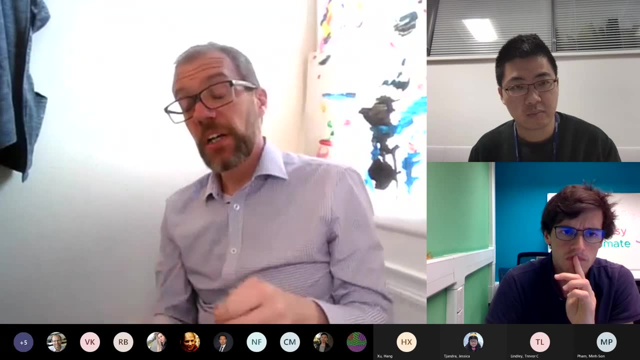 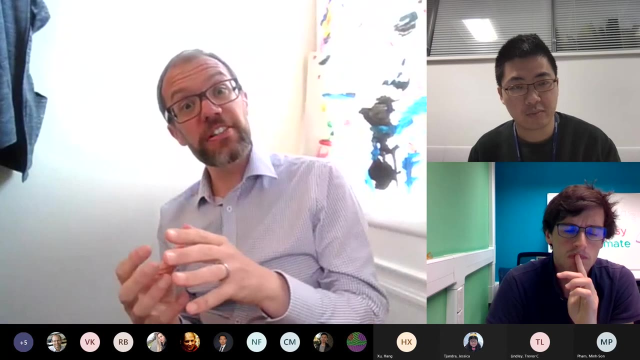 would be that you produce your component, which has a rough surface, and then you machine that off and you polish the surface to the acceptable, relatively low roughness level. but there is potential perhaps, um to to to use a rougher surface that therefore won't be able to approach. 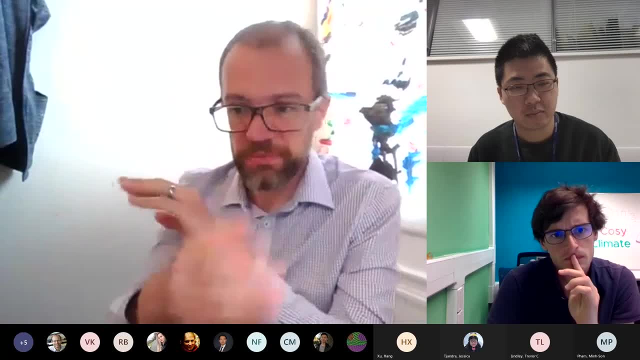 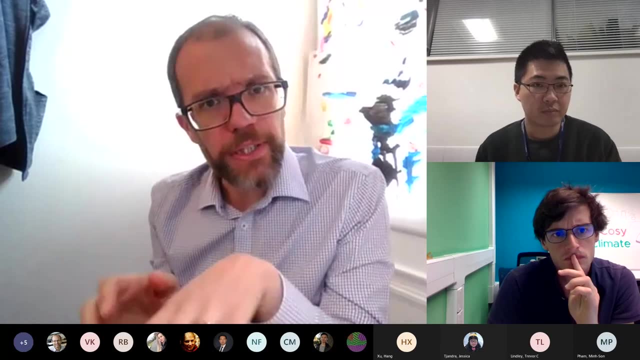 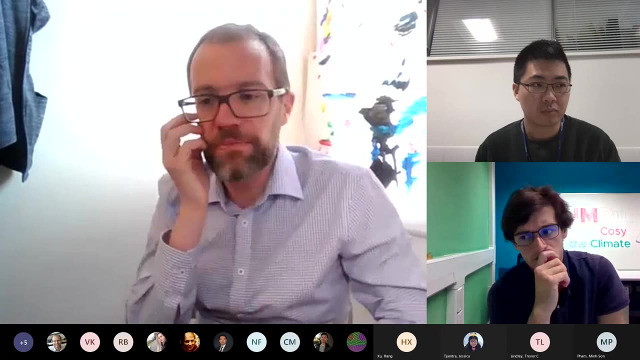 and controls your gap to be to be bigger overall, obviously with with some variation. another way to do that is to use a little bit of fluidity. um, you do need special fillers, because normal fillers um might not be comfortable in a, so to speak, in a large gap. you may need to sort of adjust the 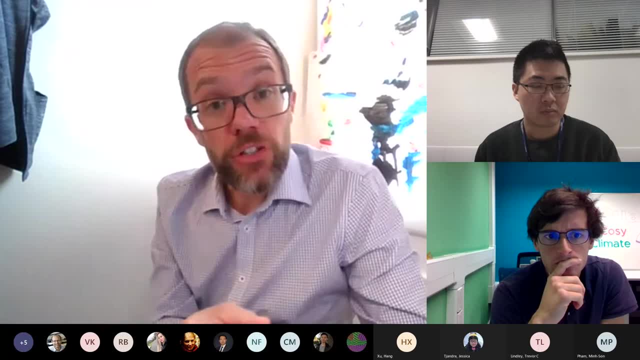 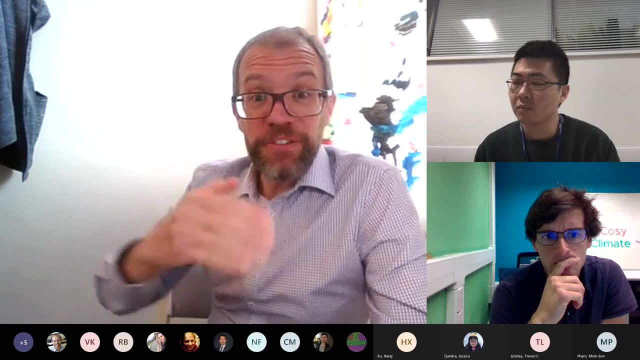 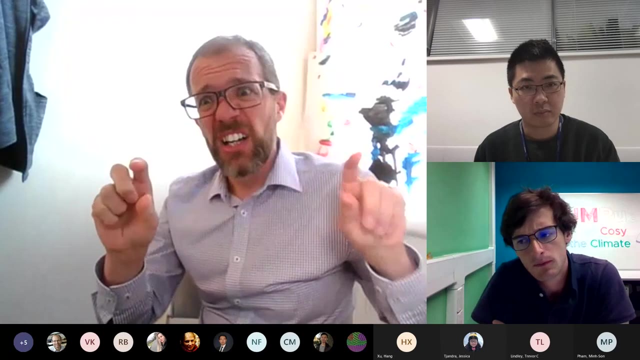 the fluidity. um, another way which is used in brazing of ceramics is to use an interlayer. so there people will do things like: uh, it's almost, you have a triple joint, or a trifoil as it's sometimes called, where you have your filler and then something soft like uh. 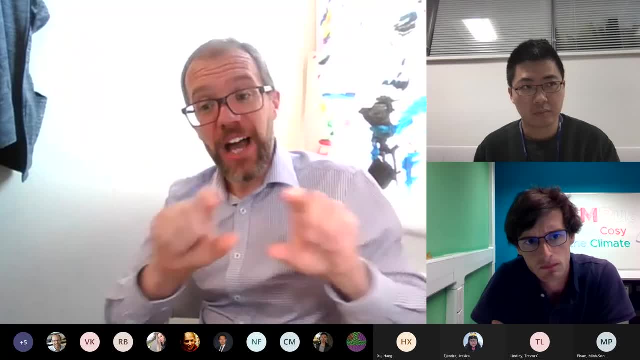 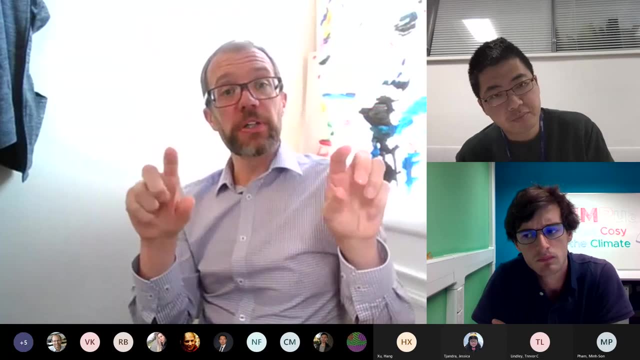 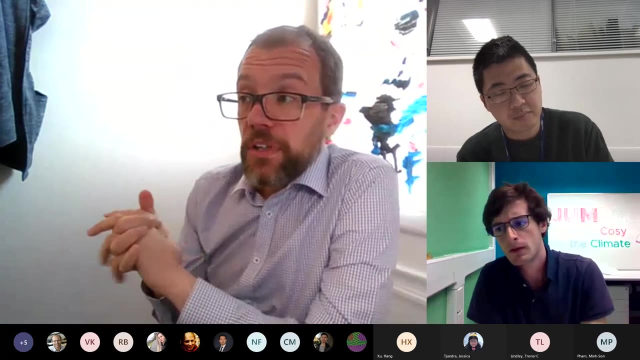 a well annealed copper or something, or very pure copper, and then another layer of filler and you, you join with that, so you have a joint to one material and then something that will plastically deform and accommodate your, your stress, and then another joint, um, that can be a very effective route, um, of course, it also potentially allows you to have 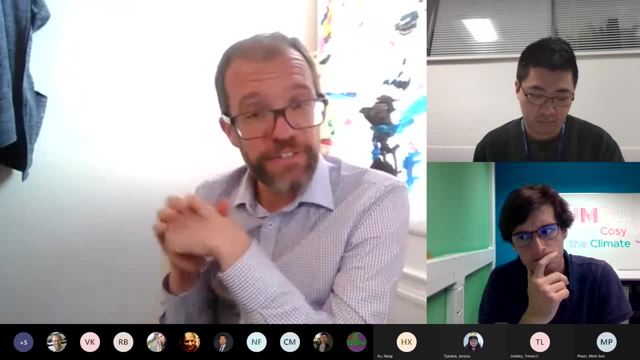 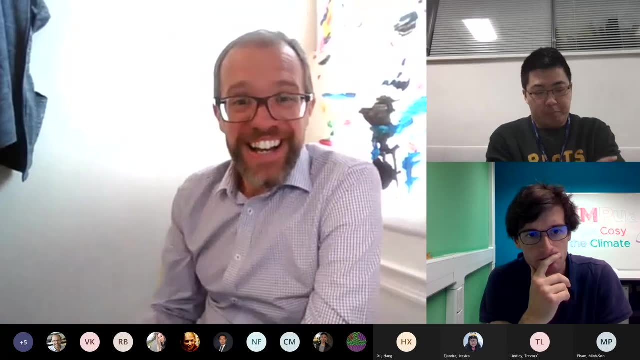 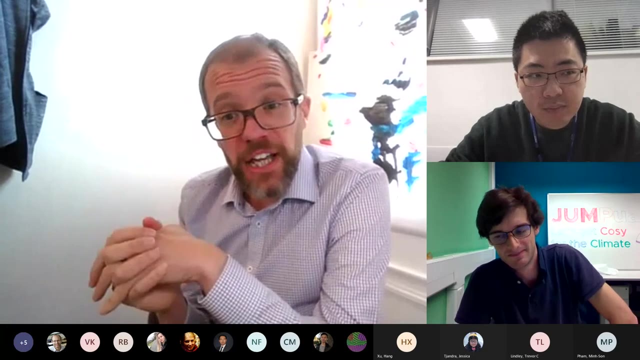 different fillers on either side that might adapt to joining to different materials, uh, where there are different fillers and then you can use a different filler to do that. so different constraints. but yeah, there's. there's all sorts of different um routes there. there's other strategies where people use foams. people use very thin slices of foams as interlayers or scribe. 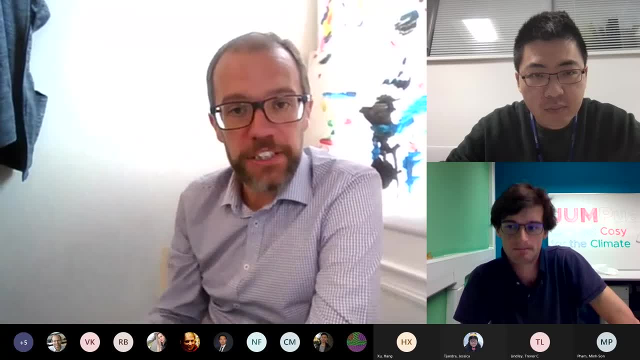 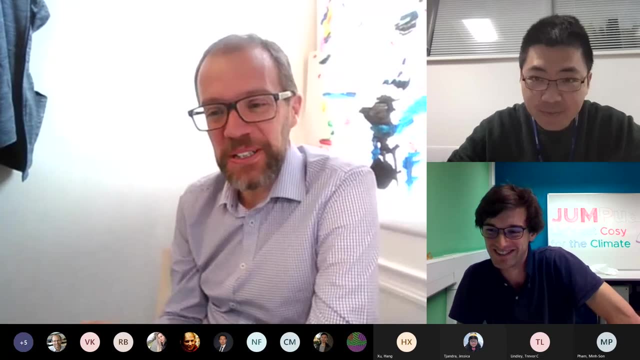 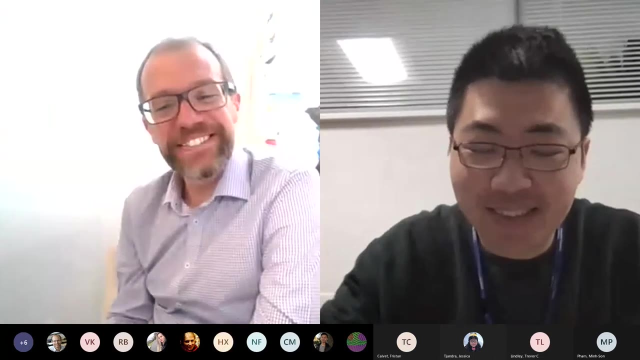 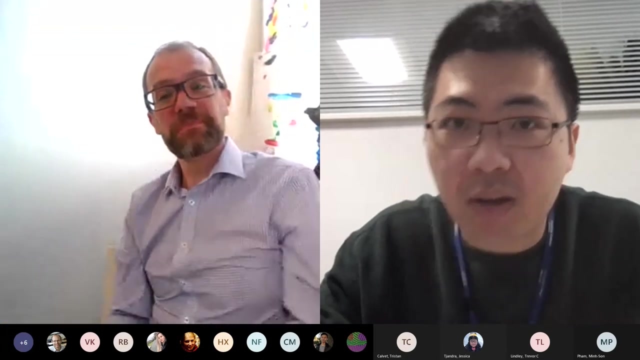 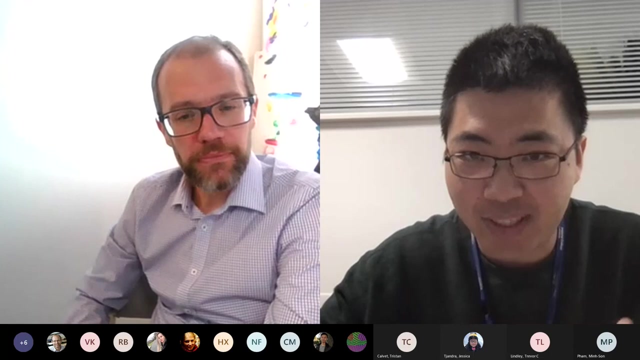 the joints to provide stress relief and things like that. there's there's a lot of different approaches that people have tried. yeah, thank you, thanks for talking. you're welcome. thank you, thank you for the good questions about the application. yeah, yeah, any okay. oh, actually, maybe a last question for myself, so for the machine learning technique, or a? 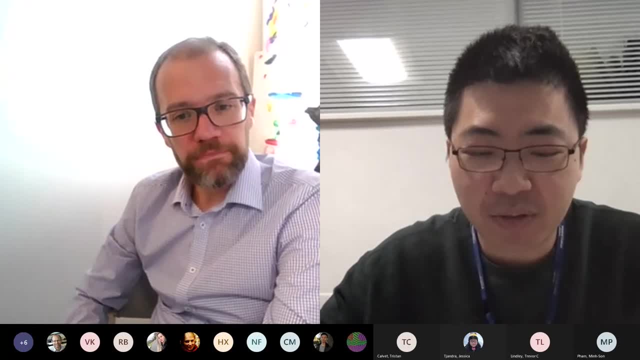 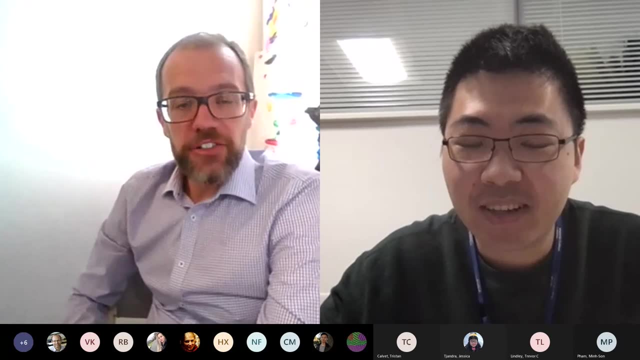 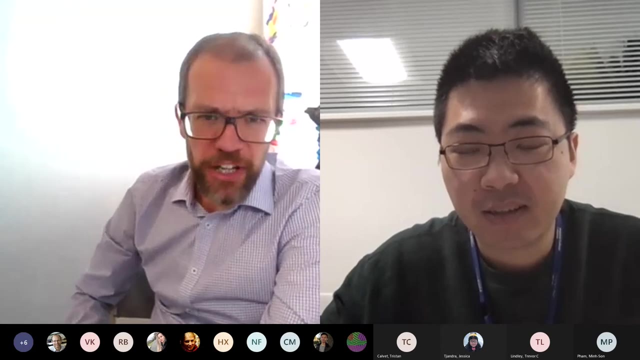 protection you're using? have you account for the dissolution from the current or substrates? no, no, we've certainly not got to that stage yet. uh, compositional drift and things like that we've not looked at. um, but really, this is this is that's relatively early stage work, so at the moment we're really asking: 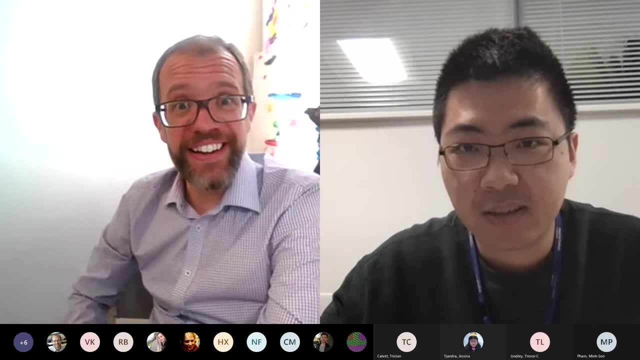 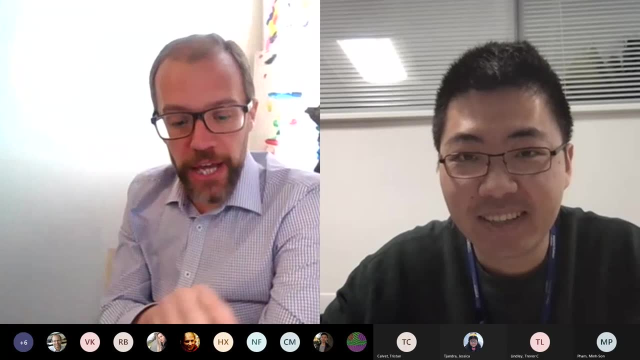 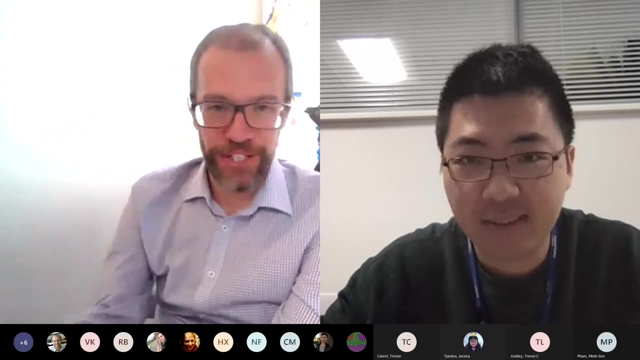 ourselves the question: can we predict a eutectic uh hea composition or not? the next stage, so that alloy that we've, that we've got there, uh that i've shown has has got a very high melting temperature now, not to say it couldn't be used there probably are. that was something that i've, uh, that i've. 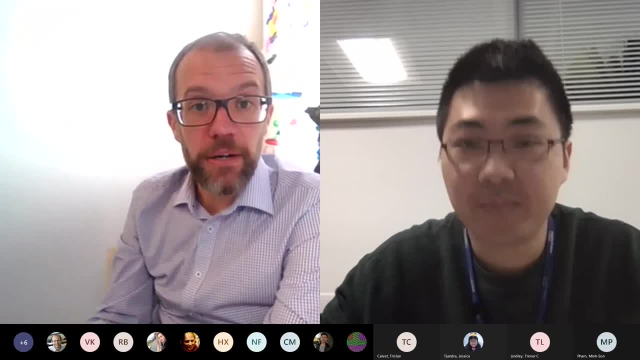 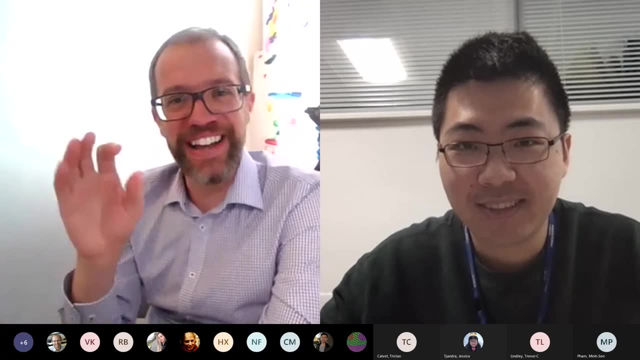 picked up from uh working with various companies about uh different materials and other situations about brazing filler metals is almost any alloy that you talk to them about. they can find some niche application where that those characteristics would be good and there are there's, there's even. 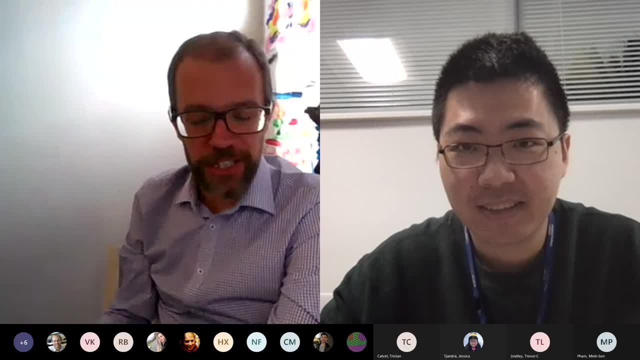 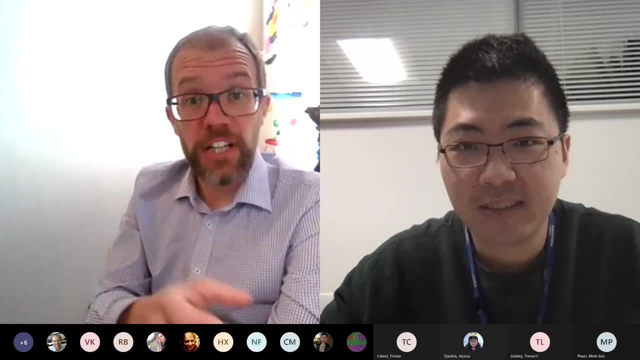 things um. an example that people sometimes choose is um, normally copper, phosphorus, brazing materials you don't join steels with because you make you make phosphides and they're brittle. they're extremely brittle. but there are some applications where you actually want a joint that will fail in. 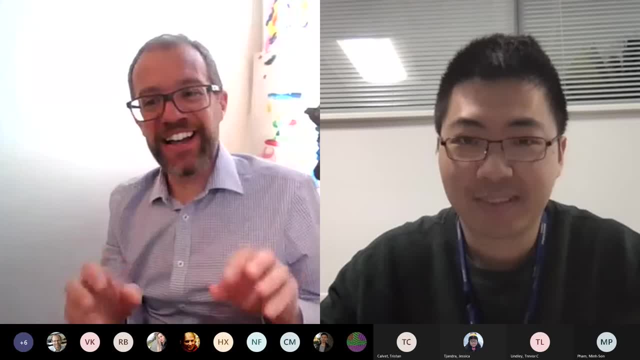 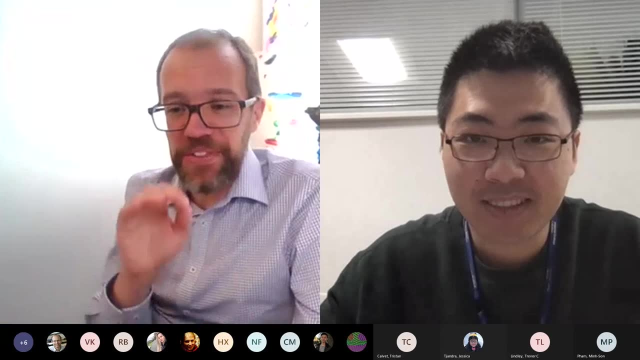 a known place and then you do use them. so even a joint that has bad properties, if you find the right application that can be a good property. so i wouldn't say it's useless. but the intent of that alloy was not to make a a filler, but more just to see can we do it? and if we find we can do it, 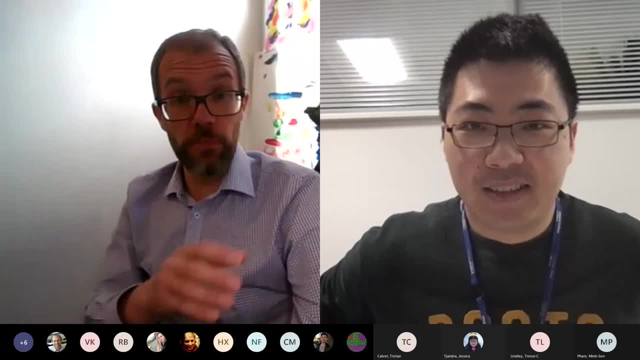 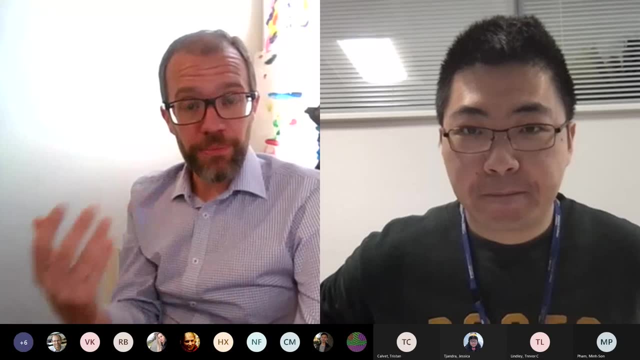 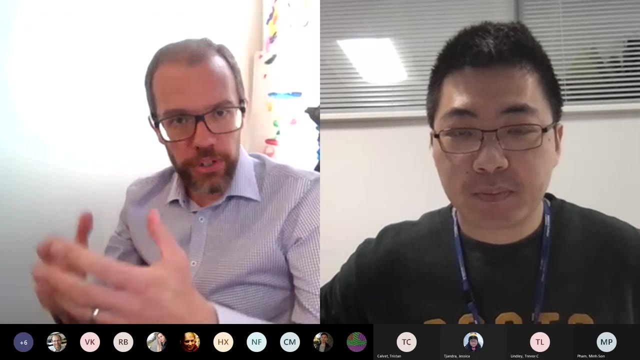 we're going to progress to use um, uh, to more, uh, application oriented designs. now, uh, along with that, we've got some thoughts about improving the model and the sort of directions that we may well go in. is is, as you suggest, looking at how, how would the composition? 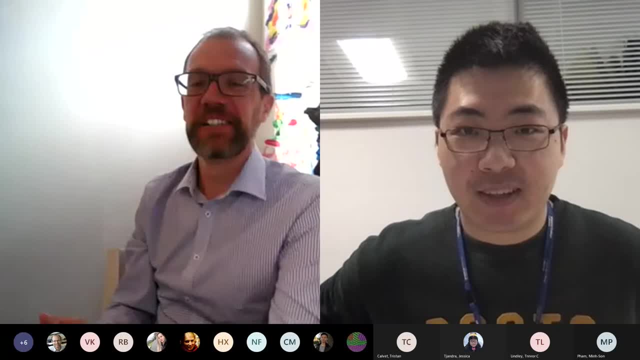 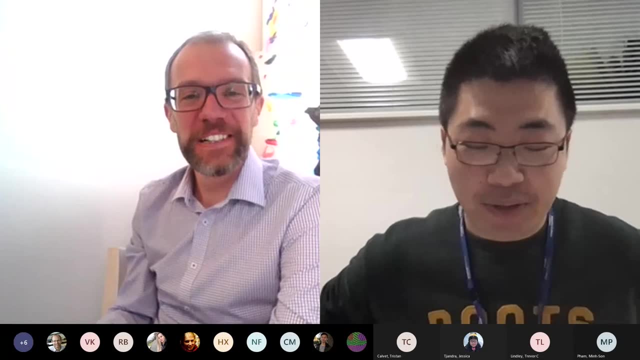 change how, how could the composition change and how would that affect it? yeah, that's definitely at least one step, if not several steps, down the down the road for us, and it's great and it's good for me. like you know, at first time i heard like that you talk about the companies actually. 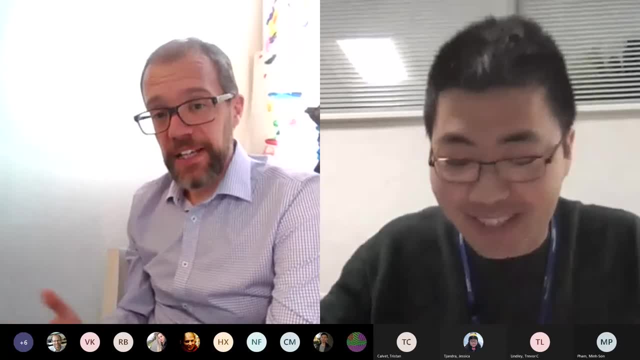 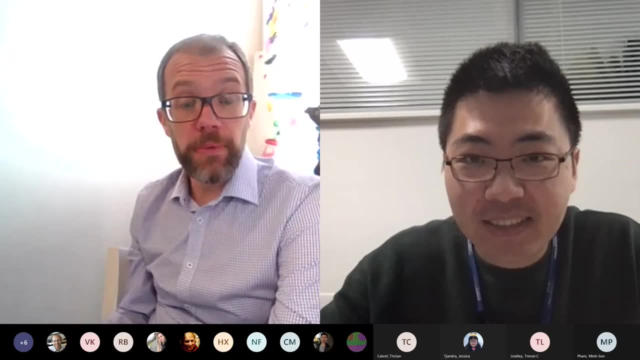 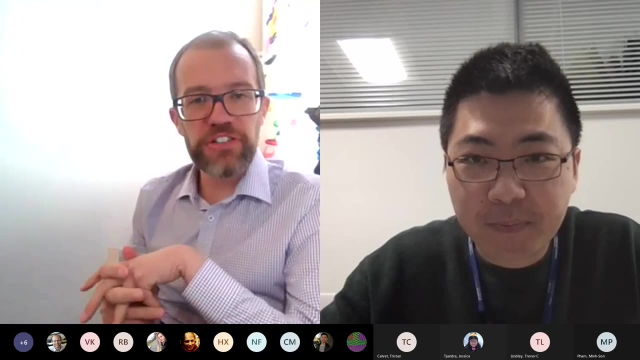 commercialize the high entropy alloy in the field, which is? it's a. it's a good example because for for many years, when, um, um, when talking to people about high entropy alloys- the people who aren't in in that in in doing that themselves- one of the first questions that they come back with is: well, have it has?